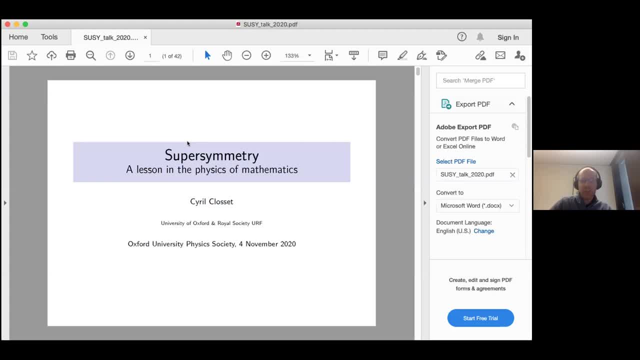 that you could call almost pure mathematics. I will give, in fact, an example of supersymmetry in a toy model of physics. So this is a kind of how you can describe a theory of physics which is essentially elementary calculus, And there I will add some parts which is a bit more technical. 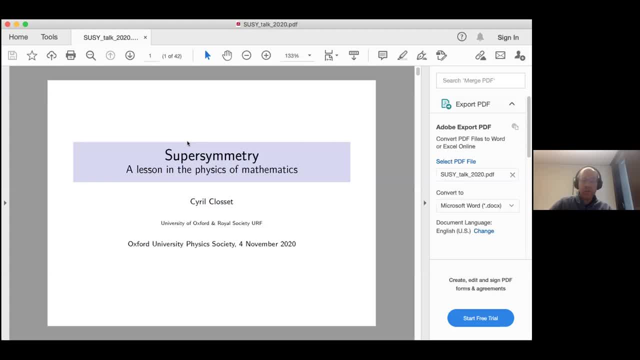 but really that any first year in physics or maths should be able to follow. And then after that I will go back a bit to a more discursive discussion of the application, then of supersymmetry, as we will see, not only in kind of motivated by particle physics, 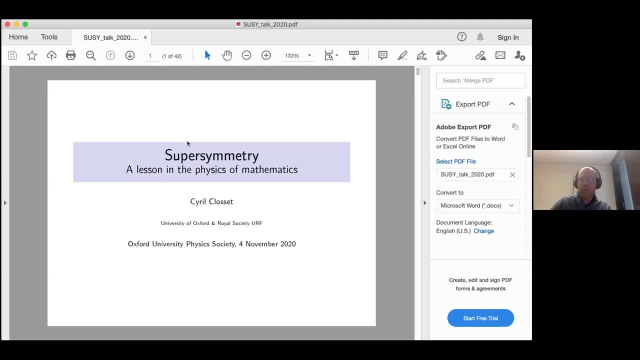 but what supersymmetry then will be like? I will give an example for that. It's a typical symmetry, then it really has an import into pure mathematics. So let me go back to the very beginning with the notion of atom And, as we know, atoms as a, as an idea, as a really physical, philosophical idea in the 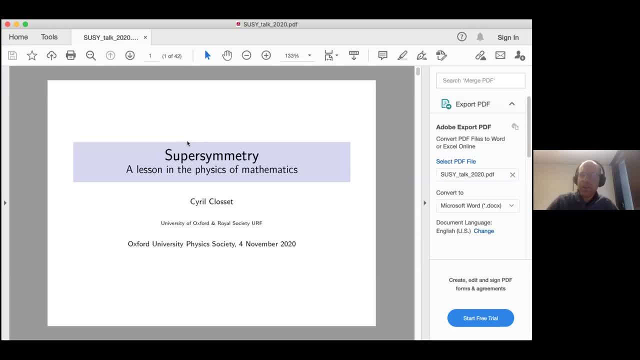 for the ancient Greeks is well, has been there since more than 2000 years ago, And it was just well, I guess, again a physical idea, but nonetheless a very powerful one, that we've come back to again and again. 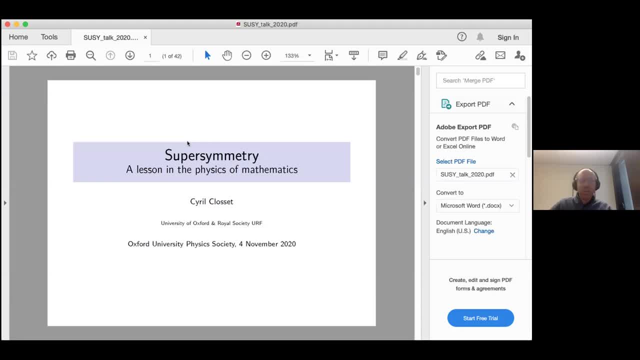 So maybe the atomic principle was most beautifully expressed in that very long poem by the Roman, by the Roman poet Lucretius, in the first century BC, where he was explaining then. then there must be some true beginning of things, some things that no force can do. 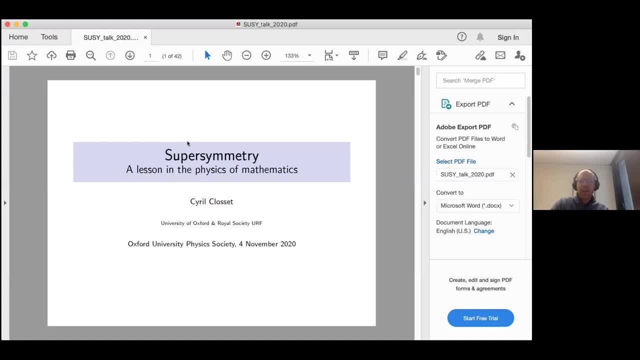 Some things can quench, for they, by their solid body, prevail in the end. So these that the atoms will be the things I quote, which exists with solid and everlasting body, which we show to be the seeds of things and their first beginning, out of which the 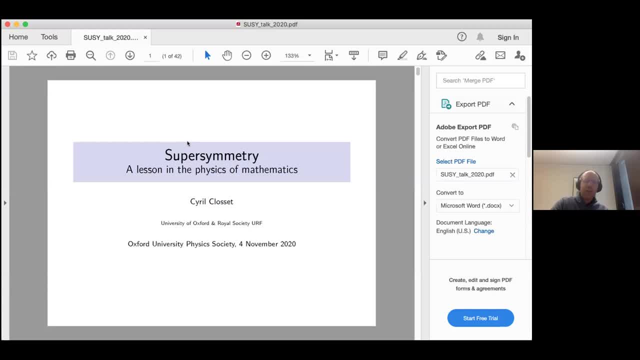 old sum of things, no stance created, And well, in modern physics we call atoms something slightly different than what they had in mind. but they were not that far off And in fact some of the arguments that they had for the first beginning of things, they 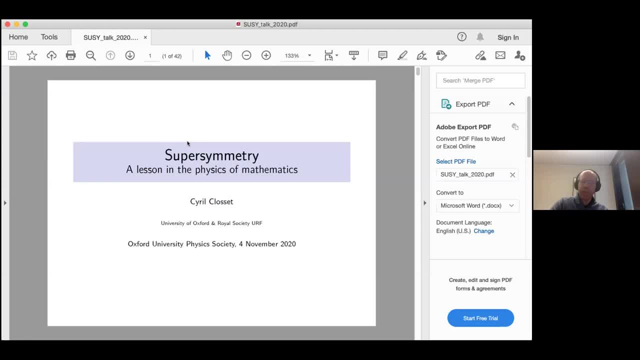 were. you know, atoms back then are actually pretty very scientific in in their, even though they didn't have the like the labs we have and so on. but some of the ideas were pretty much correct. A lot of the details, of course, were completely wrong. 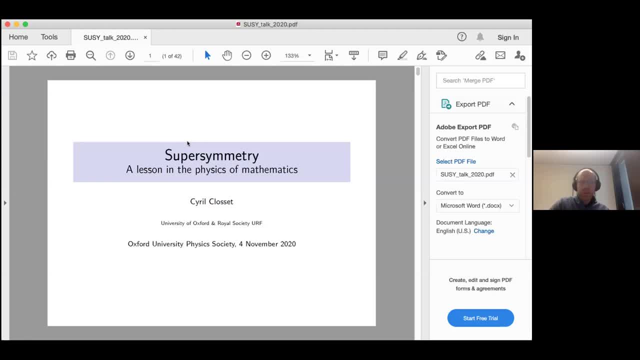 There we go, Just real quick. I'm using your slides right now because we're still seeing the first slide. Oh, sorry, This one It should be sharing. Maybe try restarting it. Yeah, Yeah, that's it, That's work. 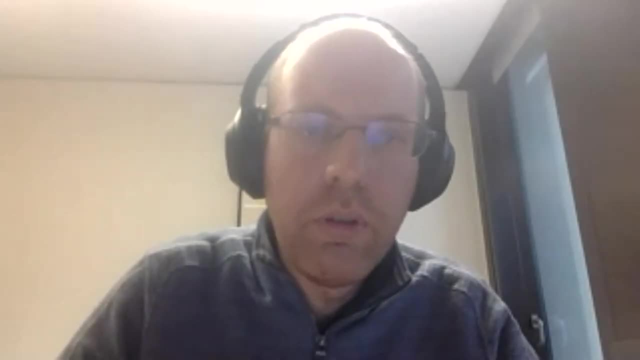 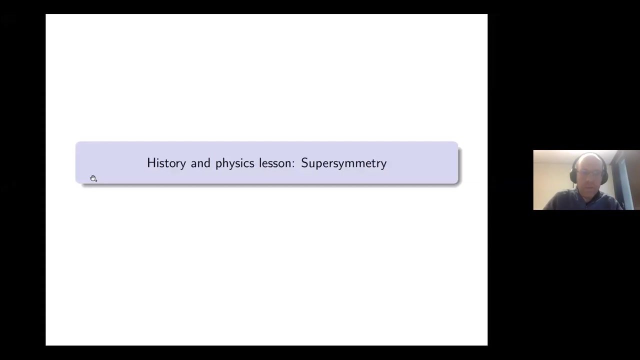 Yeah, Oh, sorry. So yeah, Tell me if that happens again. Sometimes I see that Zoom has this, this kind of bug on my computer. So yeah, so I was. I was showing this. so the you didn't see this, but you didn't see. 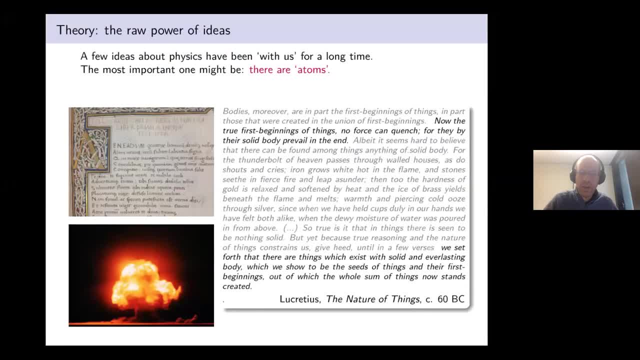 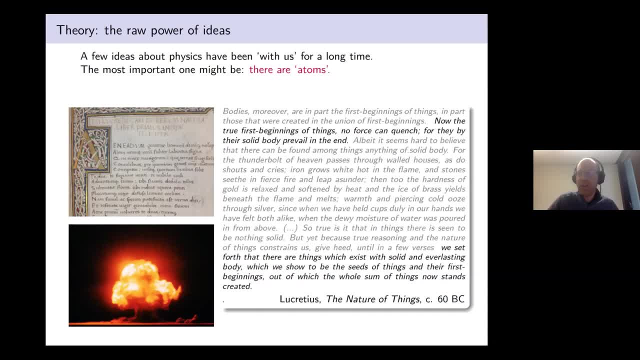 Anyway, of course, they told us that atoms was those little things that are unbreakable. That's the, the, the etymology in in Greek. And then we we called atoms those things that were building, that we discovered in the 19th century. 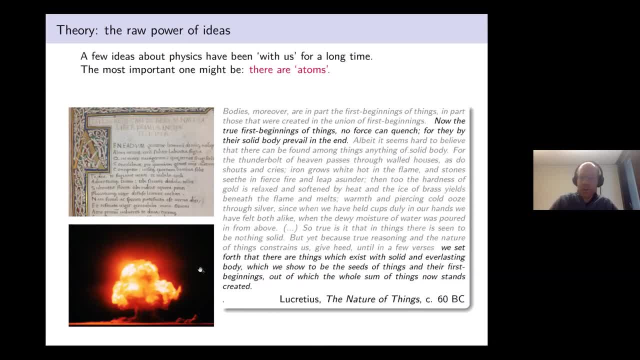 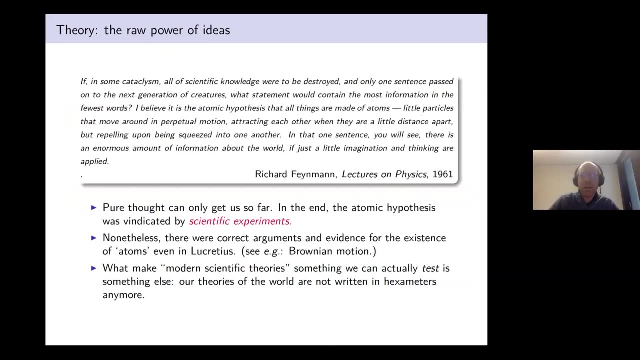 And then we realized, both tragically and and and excitingly, That in the, in the, in, Yeah, in the 1940s, that we could actually break the atoms. Now. Richard Feynman in 1961, in his beginning of: 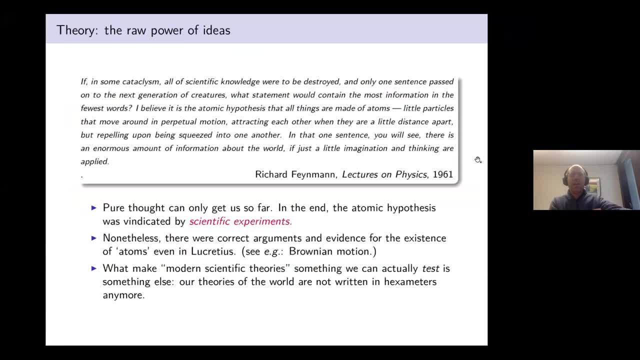 at the beginning of his lectures on physics, asked this rhetorical question: if there was some cataclysm and all scientific knowledge vanished, what? how would you carry on in one sentence, the most important scientific achievement or understanding for the next generation? And he said: let me quote: 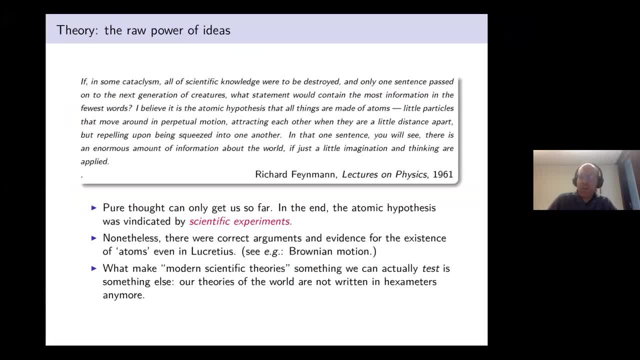 I believe it is the atomic hypothesis that all things are made of atoms, little particles that move around in perpetual motion, attracting each other when they are a little distance apart, but tripling upon when being squeezed into one another. In that one sentence we will see. 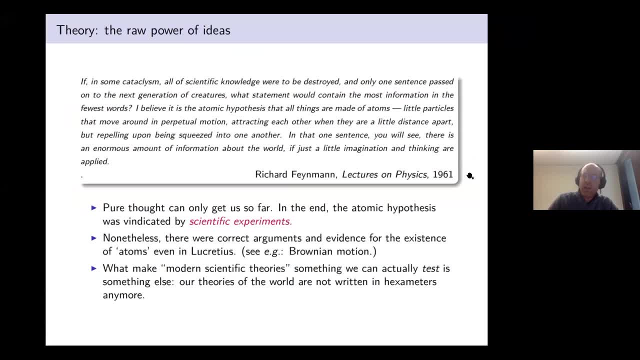 there is enormous amount of information about the world if just a little imagination and thinking is applied, And so we see in this quote, what I want to get at is the is the rope of ideas Of course we use in science and we should be aware. 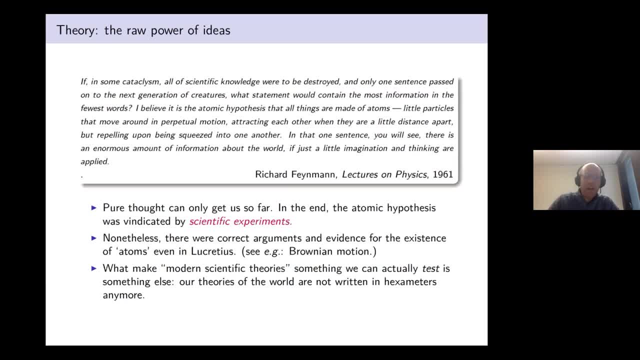 that experiments, scientific experiments, are the ultimate arbiter of the truth or the validity of an hypothesis, But nonetheless, if you take ideas and using mathematics and so on, if you take ideas and logic seriously, you can often get a very long way towards the truth. 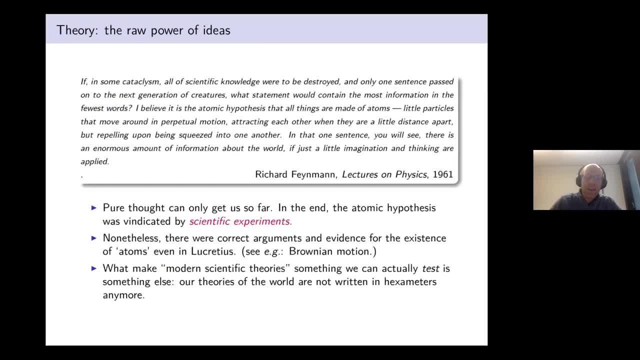 whatever that might be. In fact, as I said before, even in Lucretius there were some correct arguments about atoms or, we would say today, molecules, when they describe the thing that we know called Brownian motion. when you have a little speck of dust in water. 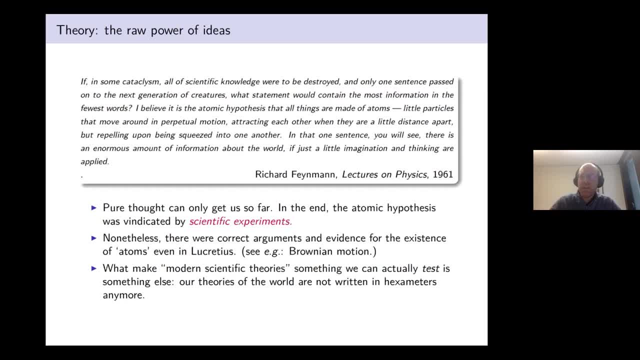 and you see that it moves randomly in water. you can explain that by the fact that there are molecules that make the water Okay. so, of course, what makes our scientific theory much stronger, in some sense, than ancient philosophies? that we can test them very precisely. 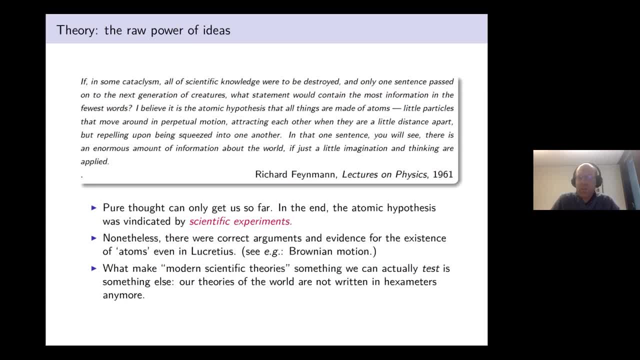 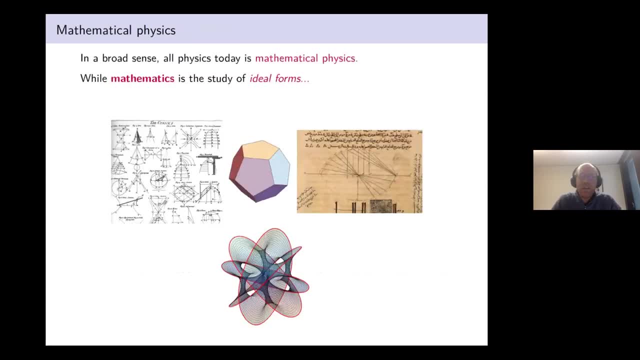 And this is because we rely not on examiner versus, like Lucretius, to describe these theories, but we rely on the mathematics, And so this talk is really about mathematical physics and, in a very broad sense, all of physics today, at least since Galileo and Newton, is mathematical physics. 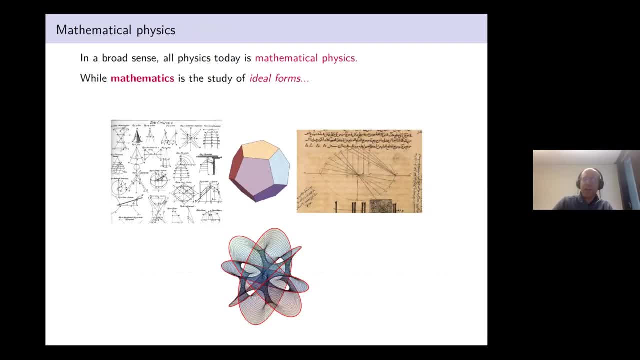 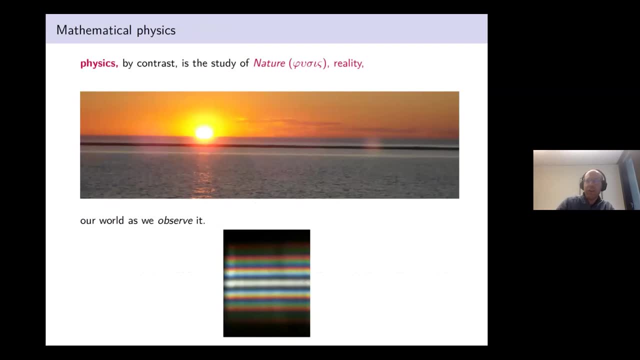 So mathematics by itself would be the study of ideal forms, But physics, by contrast, is a study of nature, physis in Greek, so what I will call just reality, or the world as we observe it. And we observe the world more and more precisely. 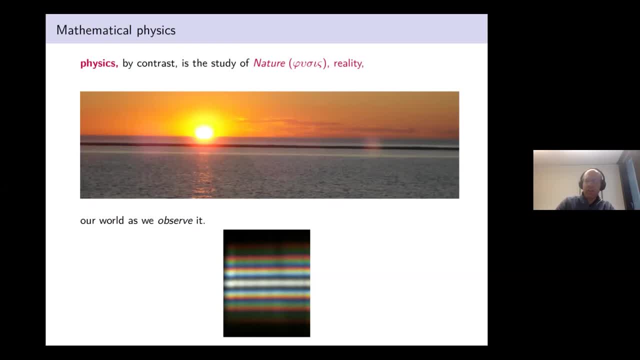 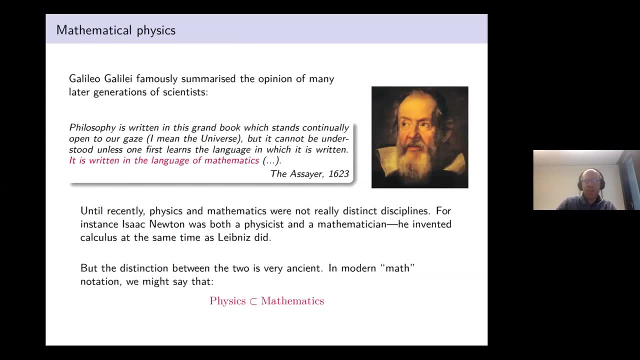 with more ingenious tricks and methods, labs and so on. So Galileo summarizes this opinion of many later generational scientists when he wrote in the 17th century that philosophy is written in this great book which stands continuously open to our gaze: the universe. 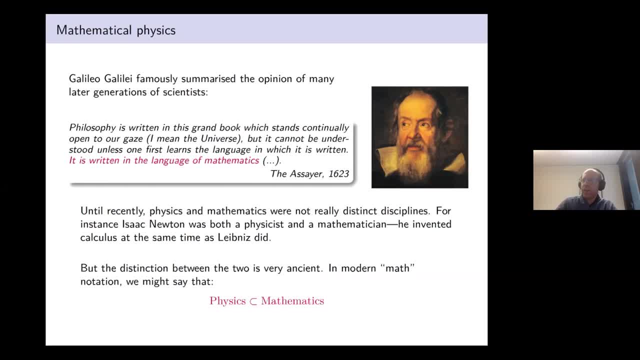 but it cannot be understood unless one starts learn the language in which the book of nature is written. And this language, he said, is mathematics. And it's interesting to insist on the fact that, until relatively recently, physics and mathematics were not really distinct disciplines. 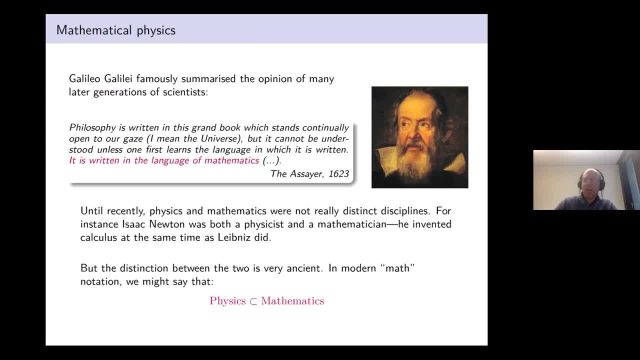 I mean, some people were maybe more mathematicians and physis, but many people who were like we would consider scientists today were called like natural philosophers. They were often as much mathematician as physis and they would develop whatever mathematics they needed. 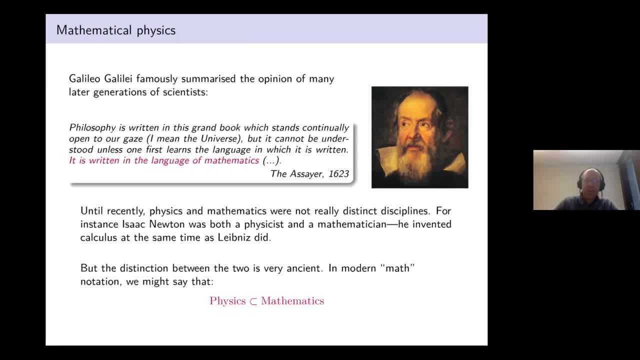 to understand the world, and so on. For instance, Newton himself invented calculus in parallel with Leibniz, who invented it independently. Nonetheless, the distinction between physics and mathematics, in the sense of having some sign of pure ideas and something which is the world we live in, is very ancient. 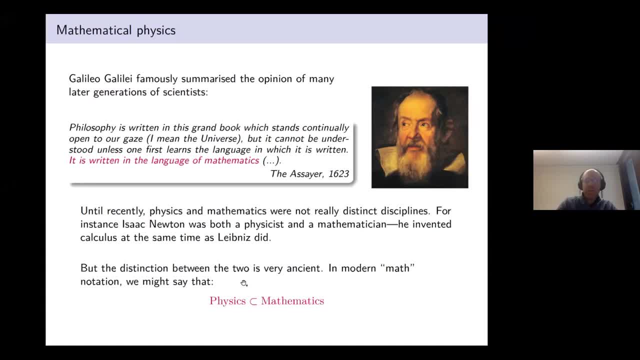 And in modern notation- maybe tongue in cheek- we could say that physics is then like a subset of mathematics. If mathematics is really the language of the world, well, there is a unique world, and we need to actually read this book now. 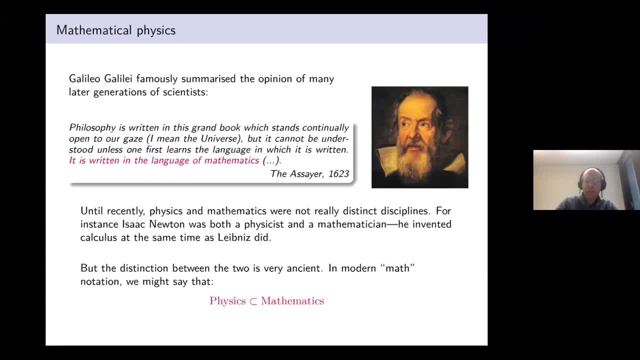 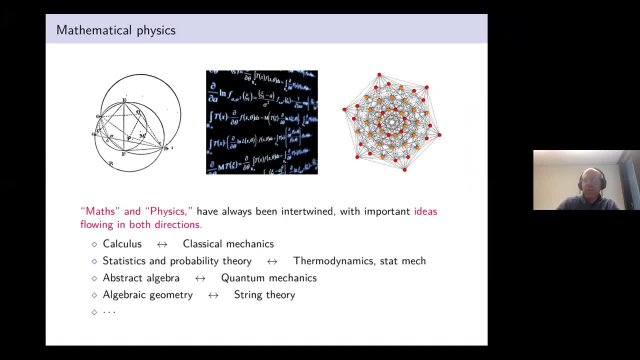 And so we first learn the language and then you try to see what the world is actually look like in this language, And physics and mathematics have always been intertwined, with important ideas flowing in both direction, As I just mentioned, precisely to understand mechanics. 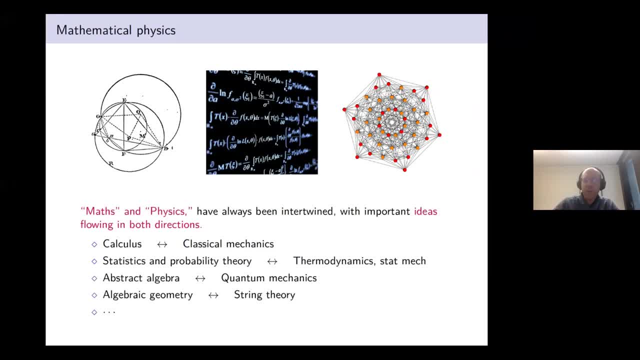 the motion of planets and so on and so forth. we have to invent the proper tools, and those are calculus that we now teach in high school and in first year at university. Similarly, the old field of statistic and probability theory was developed in good part because of the need of physics. 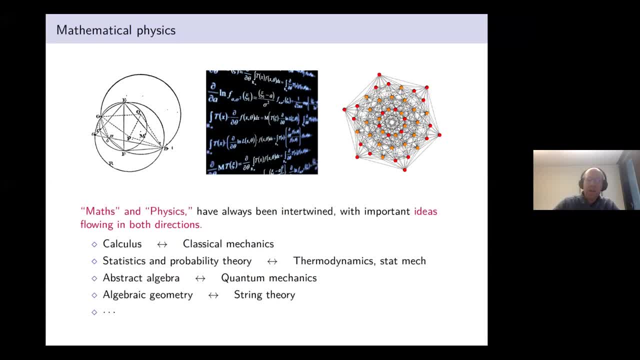 to understand thermodynamics and statical mechanics. There are also the huge realm of abstract algebra, a huge part of mathematics which in good part, was invented by mathematician over many centuries. for their own reason- not directly, directly connected to physics, but a lot of it- then become much more useful. 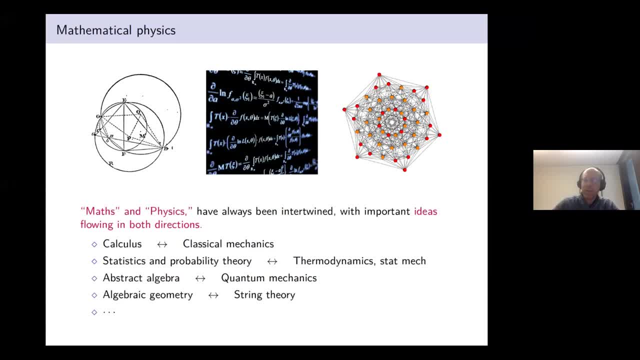 in 20th century physics, starting with quantum mechanics, which in some sense is just linear algebra, And more recently there are a lot of like more advanced physics, like string theory and some of the things I will talk about, which rely on more. 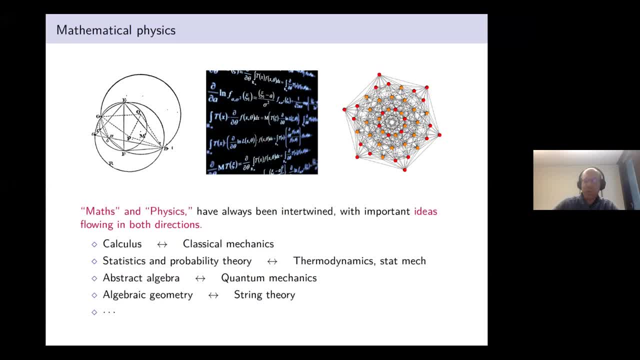 you might say highbrow, advanced mathematics, which is very much studied to this day by the mathematicians here, for instance at the Math Institute, like algebraic geometry. Now let me go back for a second to this notion of the atom. 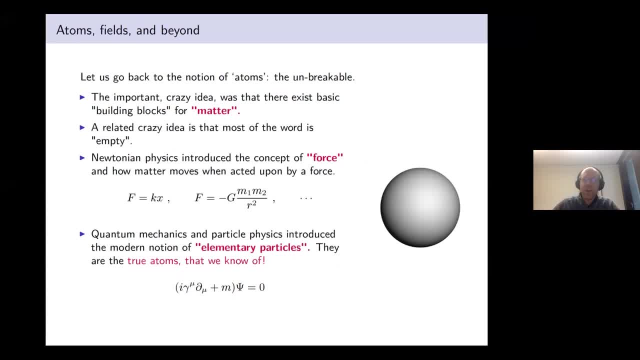 this unbreakable unit of things, of stuff, of matter, this building block, So related to this crazy idea, this crazy hypothesis that we know to be true in some sense. there is the idea that the world- there was the idea back in the days that the world is empty. 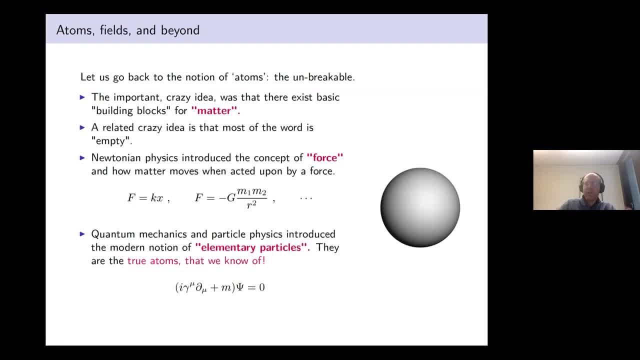 There is such a thing as a vacuum, which is not obvious at all. if you really think about, you know the world as we experience it. of course, everything seems very solid. There is air or water or everything around us. but there is this idea that if you think of this atom, 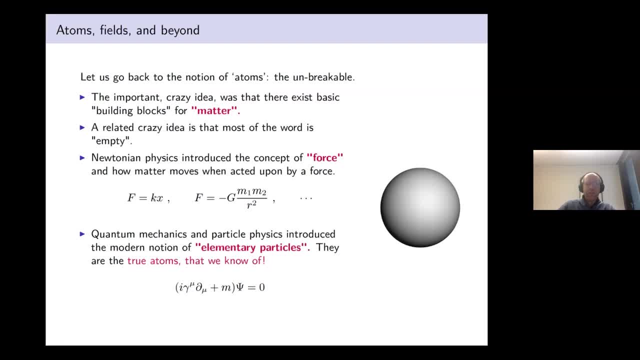 as some kind of a small small marble that it has to move around in vacuum. And of course this idea was taken on again much more powerfully by Galileo and Newton to understand matter and how it's acted on by force. So modern physics really starts with Galileo and then Newton. 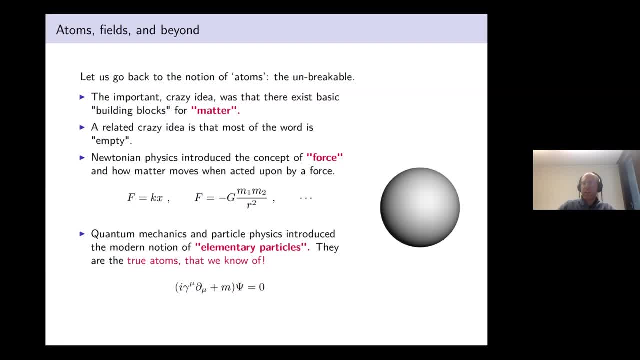 when they describe precisely mathematically how particles are acting at accident by force, with this kind of differential equation that you're all familiar with. Then more recently we had the kind of slight upgrade. I mean rather conceptually, it looks a bit daunting. 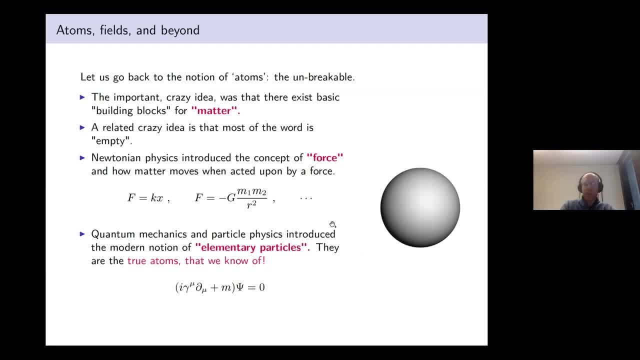 but in the end it's only a slight upgrade on this picture of the world, which is quantum mechanics, where the kind of notion of what is a matter is slightly more subtle, but still there is such a thing as elementary particles and those elementary particles. 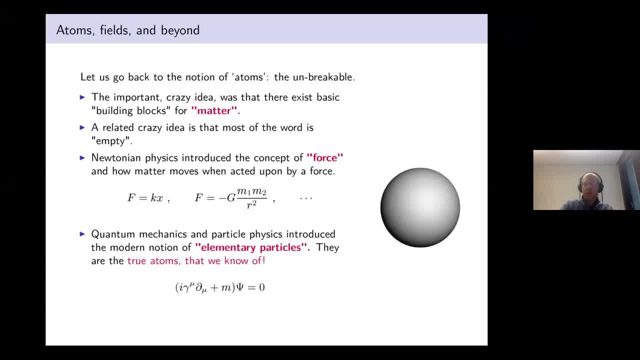 that's what I'm talking about. We discovered the electrons, then the protons and neutrons, which are themselves actually made of quarks. I will review some of it in a little bit. Those elementary particles, the building blocks of particle physics, are then the true atoms. 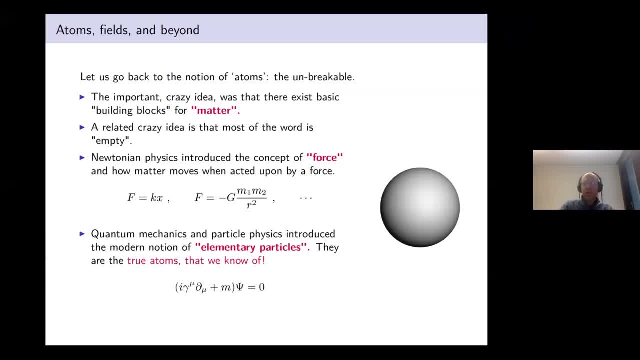 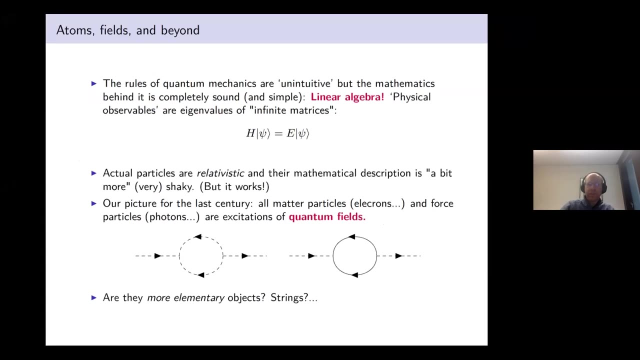 as we understand them, the true elementary stuff, And they satisfy an equation like the one below here, which this is like the Dirac equation that governs the motion of an electron in the vacuum. Now The role of quantum mechanics are a bit unintuitive. 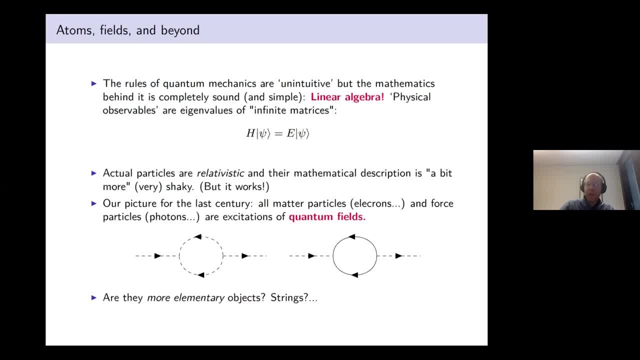 and many of you will not have studied it just yet. But in the end it's essentially linear algebra and you've all seen probably linear algebra already, like matrices and vectors and how to diagonalize the matrix, And quantum mechanics essentially tells you. 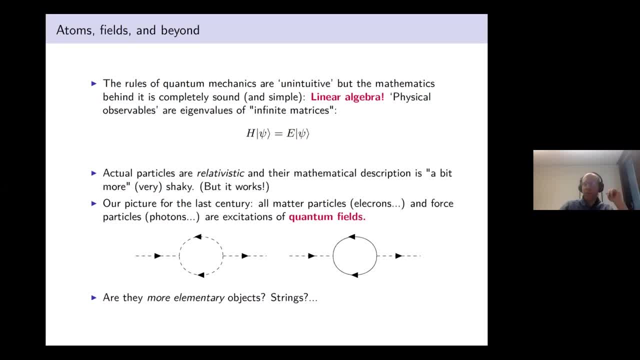 that a lot of what we call physical observables are just big matrices that you need to diagonalize. For instance, this equation would be when you have some particular quantum states denoted by psi, and you want to know what is this energy? 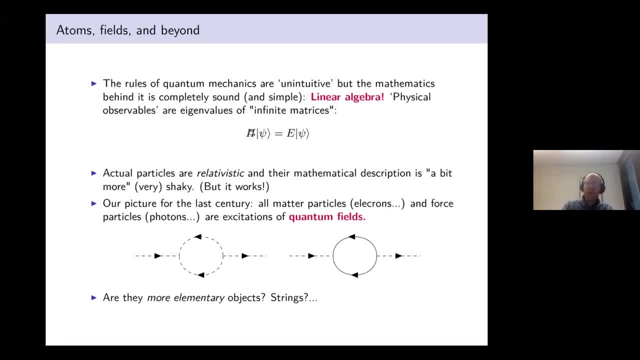 And to do that you need to diagonalize a big Hamiltonian operator, which is essentially an infinite dimensional matrix. OK, so that's what we will call non-relativistic quantum mechanics these days. Then there is the extra-liberal subtleties. 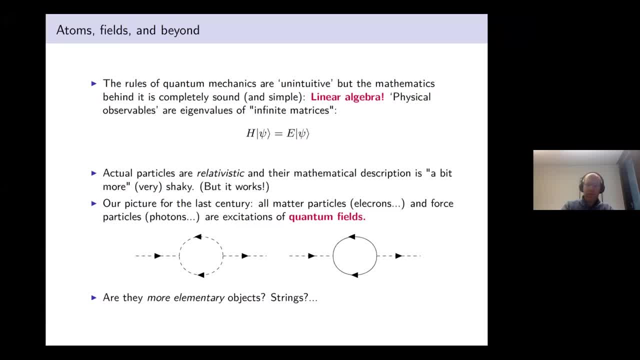 that particles are actually relativistic, So they satisfy this symmetry of special relativity. It was discovered by Einstein in 1905.. I will describe this a little bit more in a couple of slides. But the fact that the relativistics make the old mathematical description, 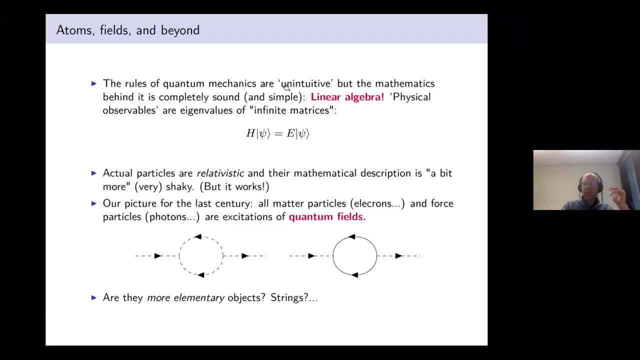 of particle physics a little bit more shaky. I just said that quantum mechanics was essentially linear algebra And this is literally. I mean, there is a precise sense in which you can deal with infinite matrices and so on. This is very well established mathematically. 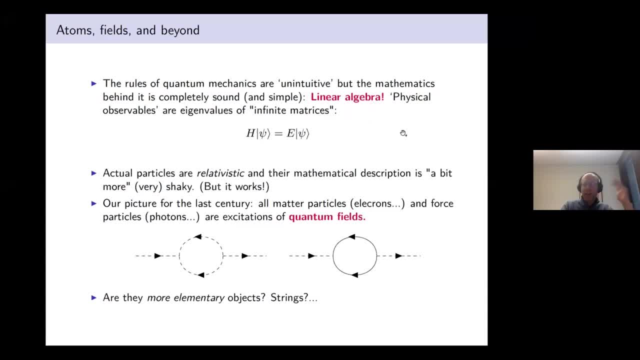 There is no problem with that. We can expand that to our mathematical friends. as this is The situation with relativistic particles in particle. physics is a bit more shaky. It works. We know the rules of the game. We know how to compute. 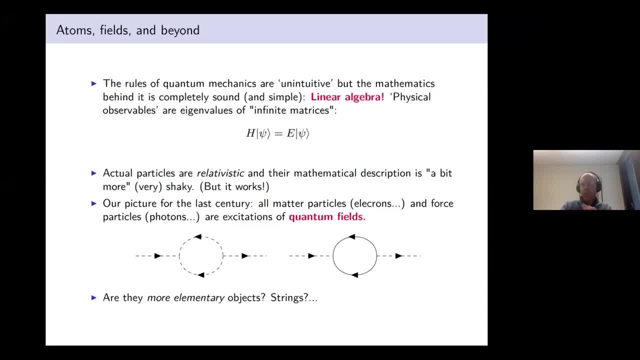 But on the other hand, I see a completely hard time, or it's almost impossible, to really explain to our mathematical friends what it means, Because essentially we don't have all the axioms and the very rigorous framework, probably because we don't understand what we're doing as precisely. 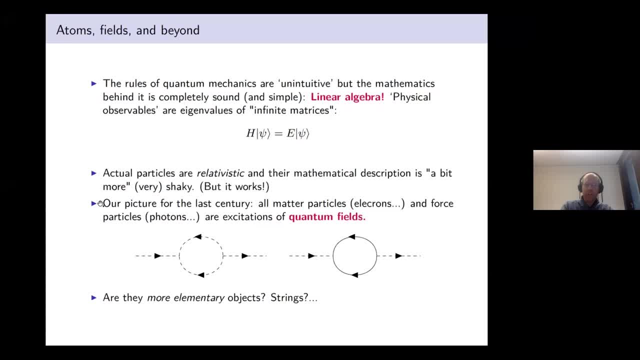 as would be needed for a fundamental understanding of it. Nonetheless, we have this, This rough picture- I mean this very precise picture, but rough mathematically- of the world as a bunch of particles. There are electrons, and so on, for the matter. 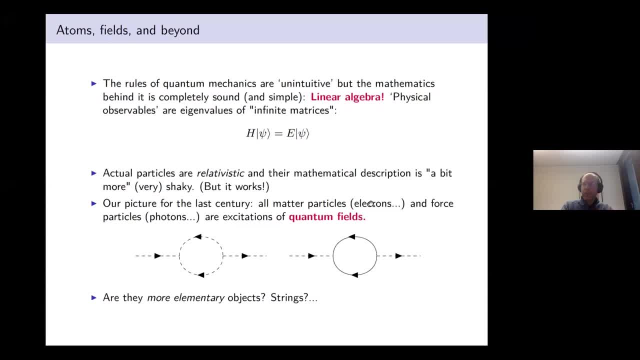 And then there are also particles which are really the force carriers. So whenever there is a force like attraction of two electrons- by electromagnetism I mean repulsion of two electrons or attraction of an electron and a proton- then there must be those particles that exchange the force. 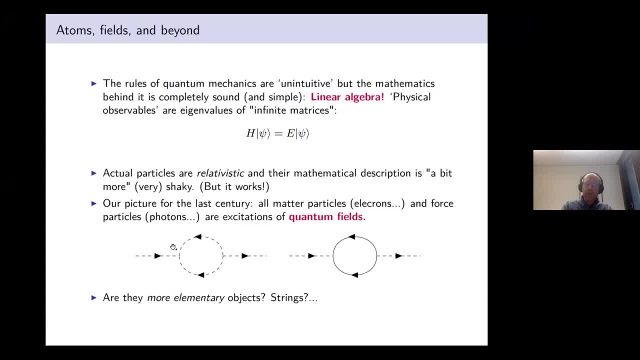 And those particles are the photon in this case, And we will kind of process In particle physics that we represent by those little diagrams which are called Feynman diagrams, when here it could represent, for instance, an electron that emits another particle. 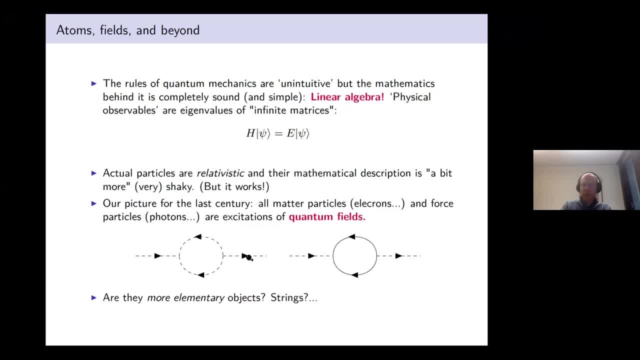 And then this particle is absorbed again And this kind of thing mediates forces over its interactions. So those are the kind of picture of the world we have very roughly today. And you might ask: are there more elementary objects? We know that we thought for a little bit of time. 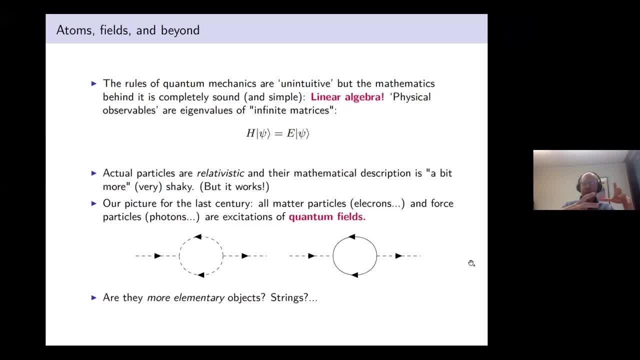 for a brief period of time in history, we thought atoms, We found the atom, And then soon people discovered the atom is really made of electrons and protons and neutrons, And themselves they are made of quartz, And you might ask whether there is something more elementary. 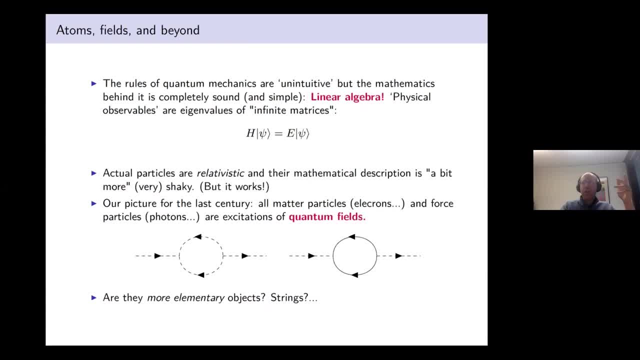 For instance, string theory proposed such a picture, But we don't really know that this is really all experimentally, for various reasons. I think you just had a lecture about string theory last week. So as far as theory is concerned, I'm going to say 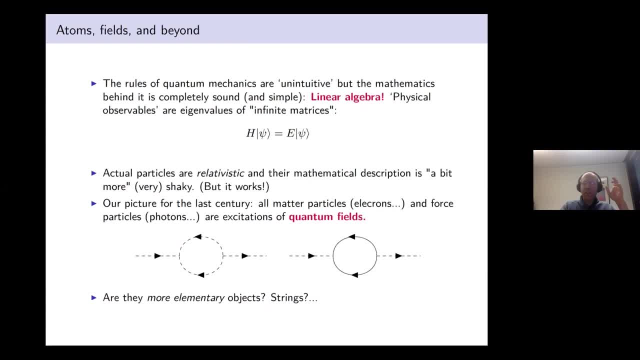 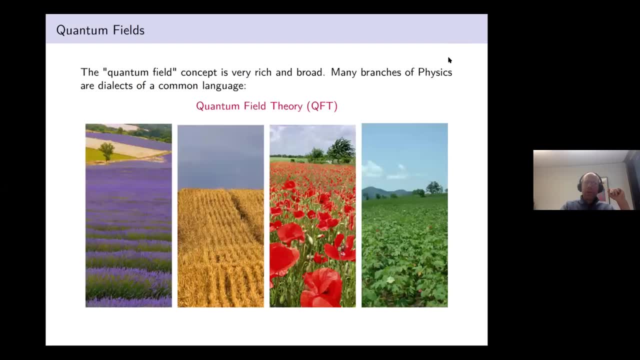 as far as we know, those elementary particles are the ultimate atom, as far as we know so far, the atom in the physical sense. Now, interestingly, quantum field theory, for various reasons, is a very broad and rich concept, So it is applied to describe elementary particles. 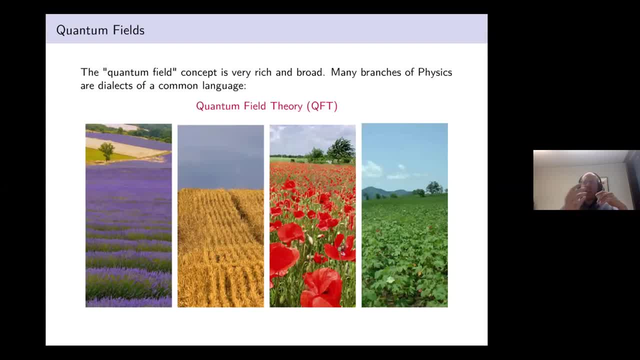 like the electron and the photon and so on, But it's also applied in many branches of physics for describing other type of phenomena which are not like fundamental, in the sense that there will be some description, for instance, of water. You can describe it as some wave equation, and so on. 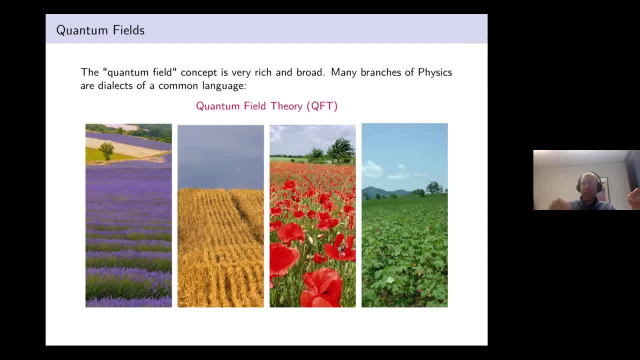 You describe water with some things that has nothing to do with the fact that it's made of molecules, which describes some effective motion of the waves, And in many cases this kind of wave motions in a quantum world, which is our world. you can describe by some what is called effective quantum field. 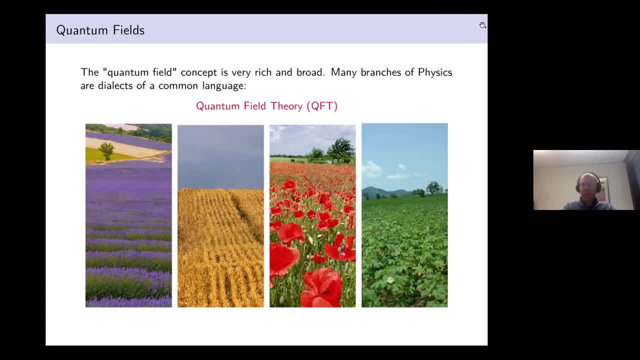 theory And the rule of this are the same as for elementary particles. So really I can say with confidence that the most important branch of physics today, or the most versatile language of physics, is quantum field theory, And those quantum fields come in many kind of flavor and colors. 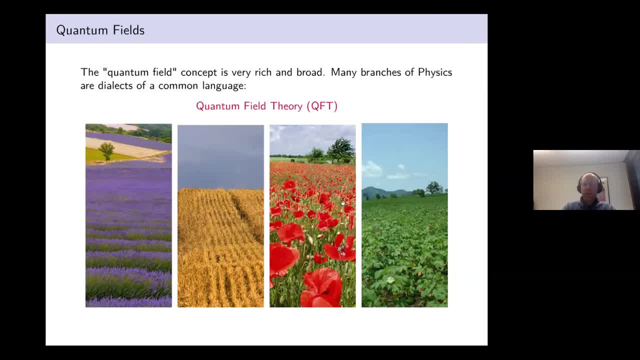 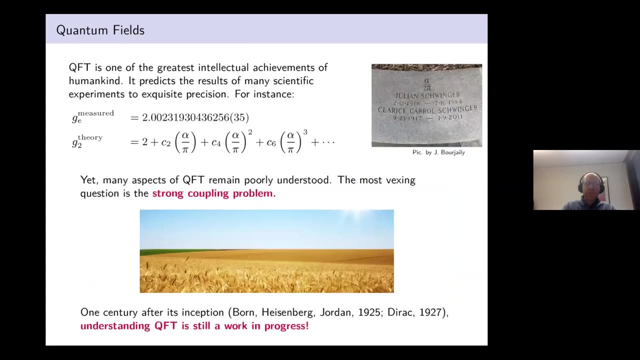 and so on, But they're all fields And then, once you specify the kind of fields you're dealing with, you can play the game of quantum field theory and try to extract prediction for experiments. Do you still see the slides? right Here we have. yeah. 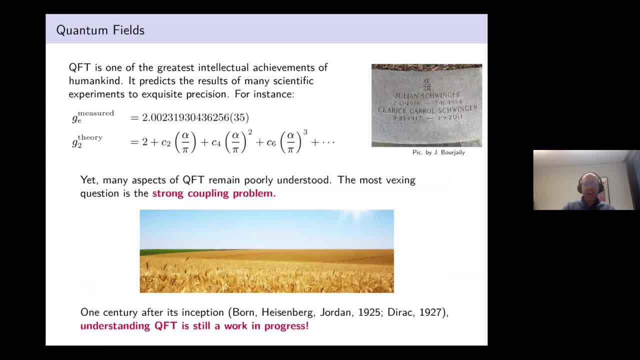 So QFT, then, is one of the greatest intellectual achievement of humankind. I can say that, qualitatively, There are many quantities that we can predict from theory, And then you check in particle accelerators And it matches to astonishing precision. 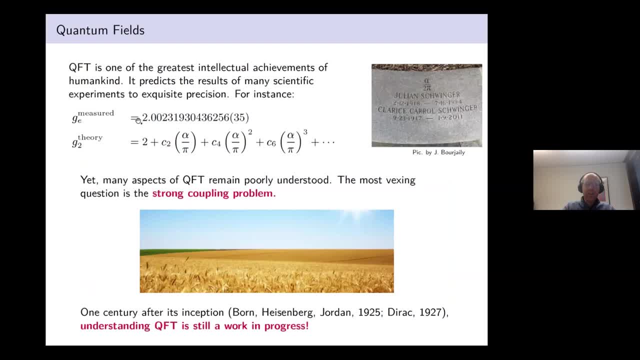 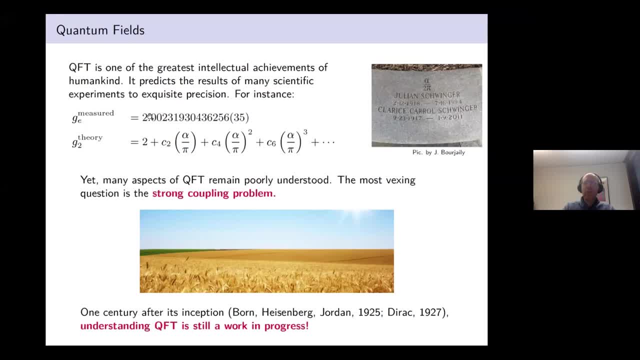 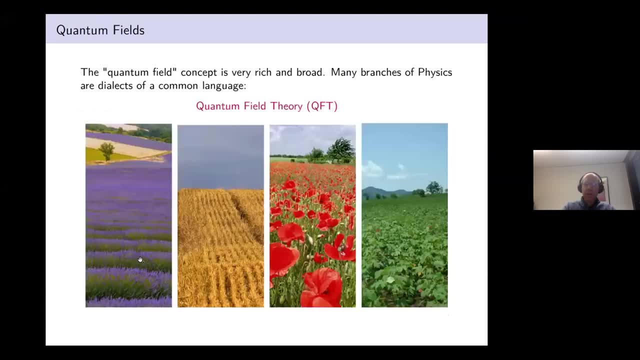 Without all the subtle corrections from quantum field theory, it would be equal to 2 in some units. And then you look at the corrections that that has to do with this kind of diagram that I wrote here That you have an electron that interacts with itself. 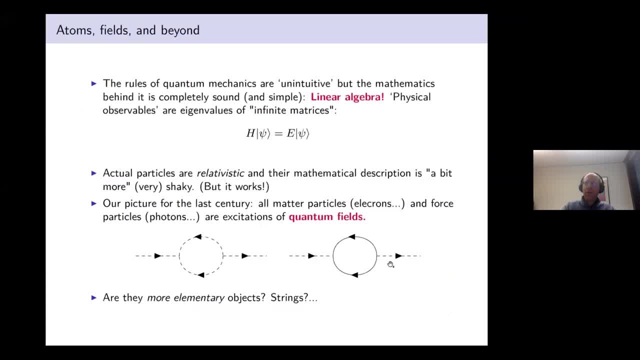 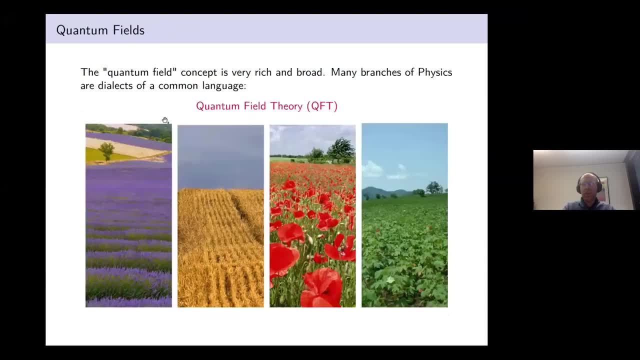 Or it interacts with a photon And direction. We correct this result, But you see, it corrects with a tiny amount, in this case by one thousandths. And then you have all these numbers that you can really compute and match to experiments. 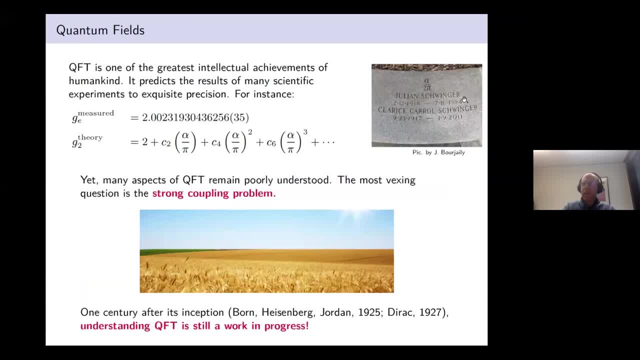 In fact Julian Schwinger, here, that tombstone on the right. he was so proud when he first computed at least the first two digit here of the correction uh, that you know he put that on this tombstone- the alpha coefficient. so despite this, uh, these beautiful successes, um many aspects of qft remain poorly understood and 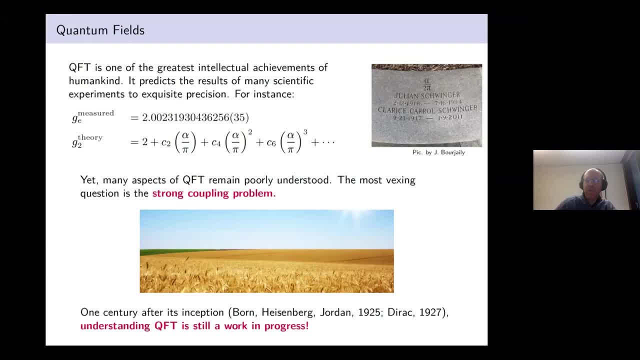 and one of the conceptual reasons for that is relatively simple to explain. it has to do with the strong coupling problem. though this is the issue that in many cases, like in this particular problem, i have this number, i want to compute the correction to g equal two and i compute and i see. 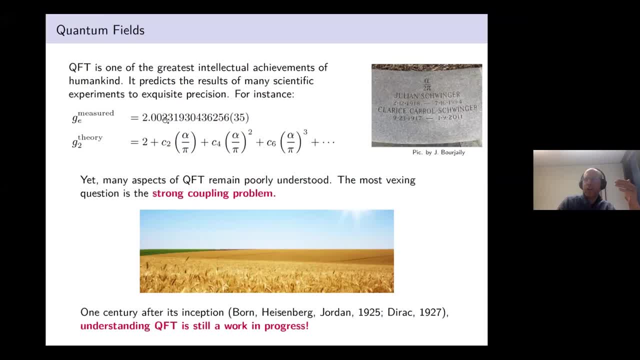 that the first correction. when i correction i mean that quantum correction. there is something which you might call a classical physics approximation, and then you, you have quantum corrections, and in many cases those quantum corrections are tiny numbers, like here, 0.01 right of the the original result, and then you can organize the, the correction, in this kind of series when 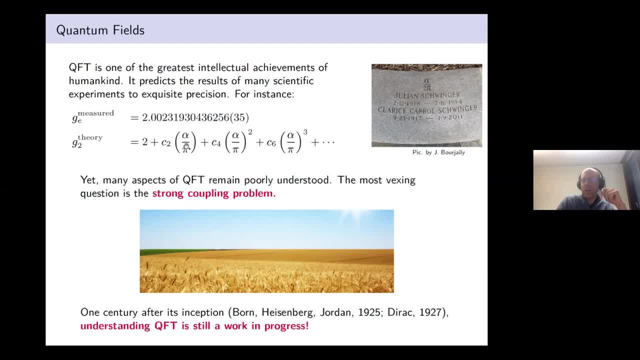 if alpha is a tiny number, alpha over pi is a tiny number. and then with a coefficient c2, and then i follow, pi squared is an even smaller number. so we have this what we call small coupling, and this small. and then you, you just need to compute order by order in this, uh, what we call. 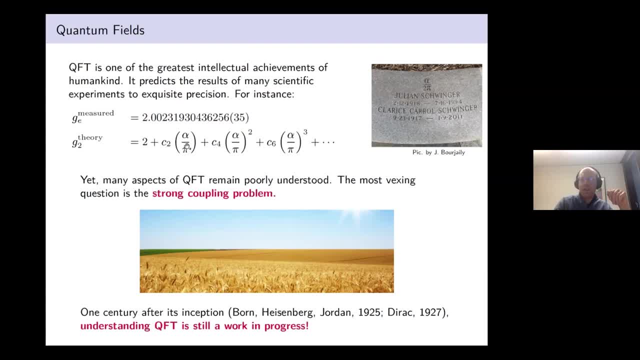 a perturbation theory of series. so there is a series of coefficient all smaller than the previous one and you just sum all of these corrections. so when you, you do that, then you're you're on good shape because you know what you're doing. you, you know that you can neglect the next correction. but 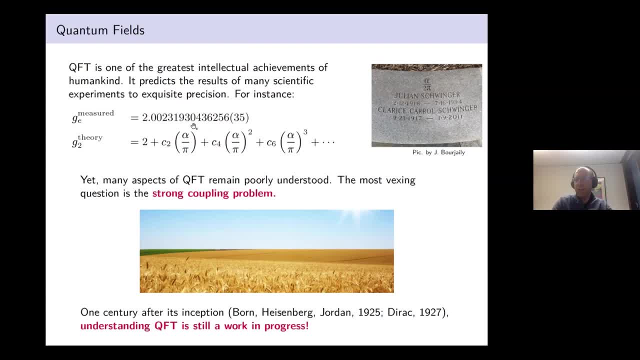 it will only appear on the at the fifth digit or the seventh digit. so you know what you're doing. but what if this, this, what if it could happen- and it does happen in some theories- that in principle, this correction, this alpha parameters would be, uh, or would be one instead of one percent? it will be. 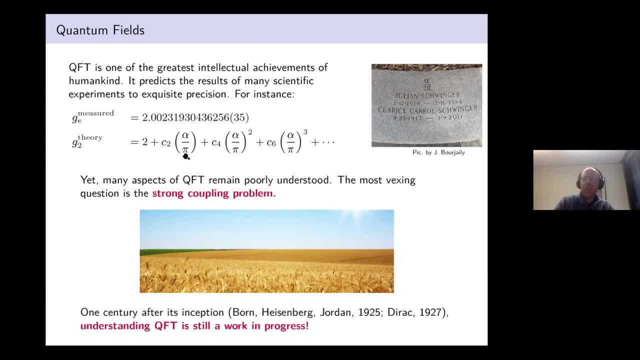 10 percent or 50 percent, and then you will have like two plus one equal three plus one. then you don't know what you're doing. it could be whatever and in principle you still have to sampler this correction, but you don't really know how to make make a sense of this computation. 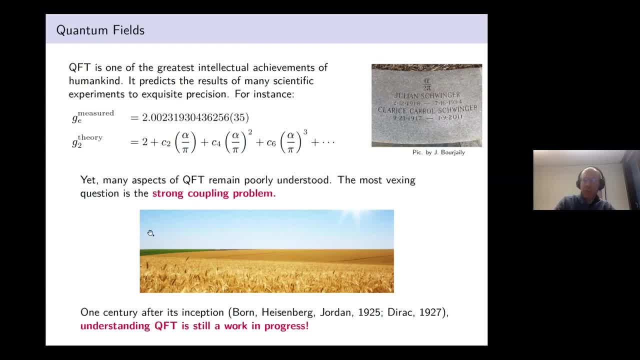 precisely so. this is what is called a strong copy problem. i have this metaphor of a field here. if this is a class, if this is what we call a perturbative field, it's something with only small corrections. that's a very nice picture of a sunny sky, but 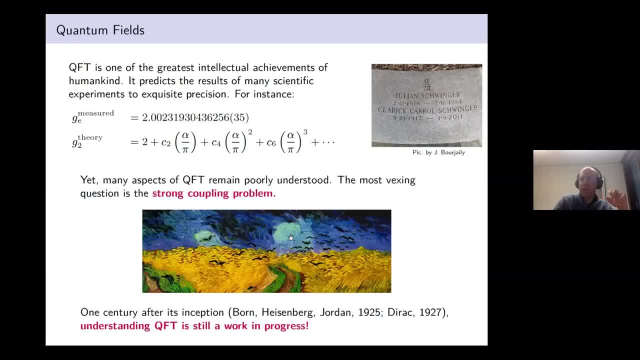 this is my strong coupling problem: when all the interaction or the self interaction of the field with itself is so strong that it becomes very messy and we don't really know what we're doing. so for this and other reasons, but mostly for this reason, i think: uh, one century after, 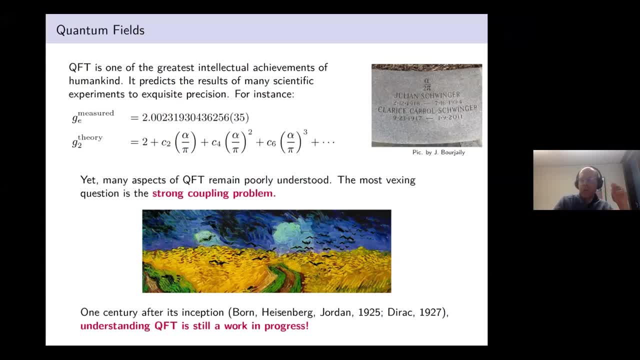 in its inception. quantum field theory was first described, at least for electron and photon- in the 1920s. but one century later we are still trying to understand what qft- quantum field theory- is all about. it's still very much a work in progress and we're still developing new tools. 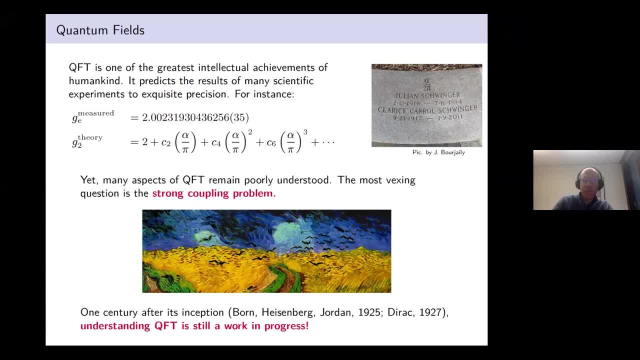 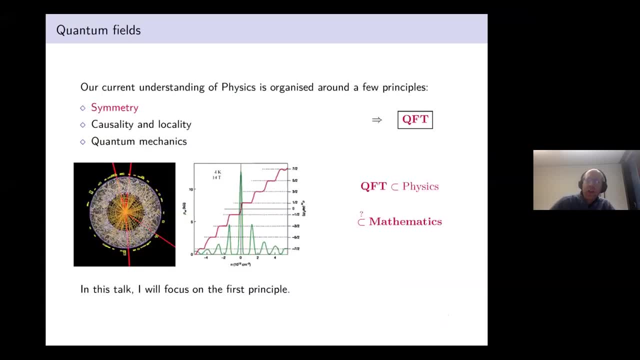 to to do computation and quantum field theories in a in an efficient way. so quantum field. now let me. i thought i was telling you about quantum field, but maybe i should tell you a little bit more about about what they are. well, some, i guess i won't tell you too much about what is a quantum field? 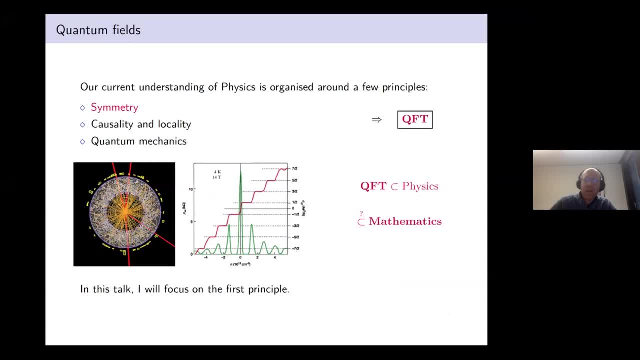 our current understanding of physics is organized around a few principles which which all point to quantum field theory, and those. those principles are symmetries, and i will focus a lot in this talk about symmetry, since we want to talk about supersymmetry. then there are other principles which are very important. there is causality and locality, which 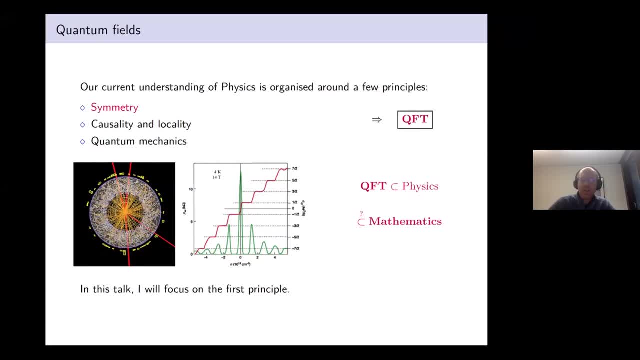 are related to some symmetries, as we'll see. but this is, like the, the key site of einstein's theory in 1905- special relativity- and that i will discuss a bit less today. and then there is a very general principle of quantum mechanics, essentially these things that 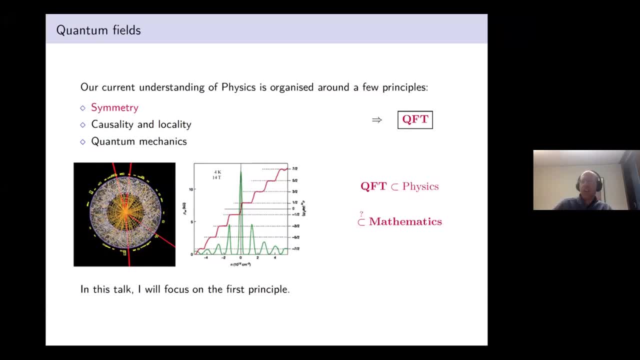 i was thinking about quantum mechanics in some broad sense is just the statement that observables satisfy some kind of linear algebra. observables means means anything that i can actually measure in experiments, and using only those three principles one can derive the general structure of quantum field theory, the general rules in which quantum fields interact, and- and we can write rules for. 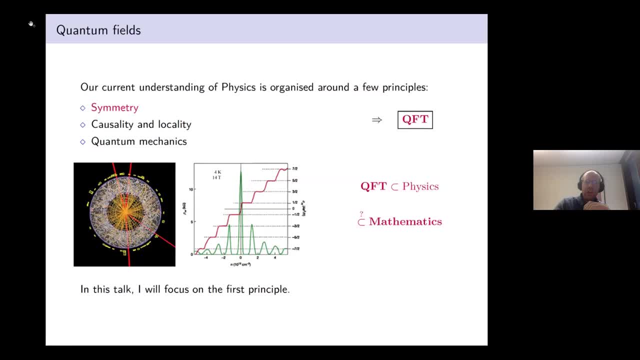 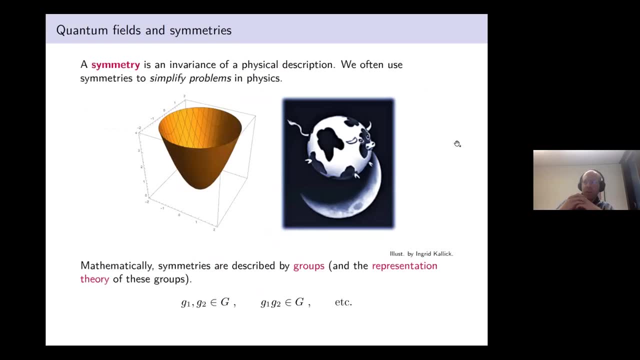 computing, things like this, this correction here, and so on. so let me first focus on the on the first principle. uh, of course, symmetry is a very important concept in physics. from from day one, symmetry is just an invariance of some physical description. so, for instance, we might have some 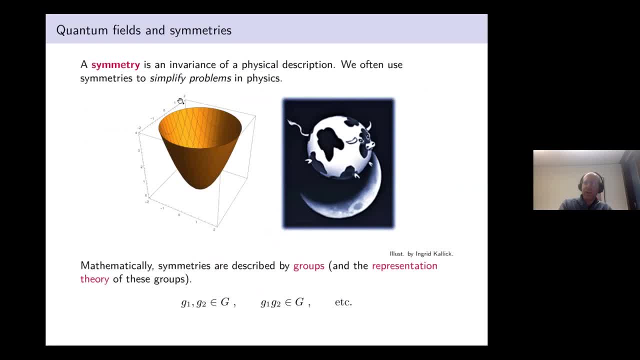 problem with some potential or something like that in classical mechanics which has rotational invariance, like on this picture on the left, and then we will use the right coordinates, for instance radial coordinates, to take advantage of the of the rotational invariance. so in that sense they are just something that we use. 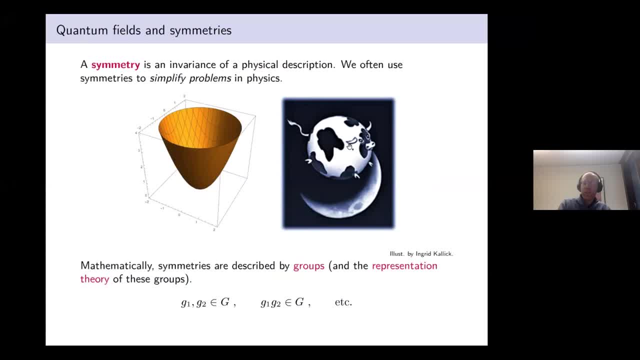 to simplify a problem in physics, and there is this classic joke about the spherical car- that if faces try to model a car, it will first assume that the car is spherical because it's simpler, and then you will try to see if the legs and the head are small corrections, while in that case they might not be. 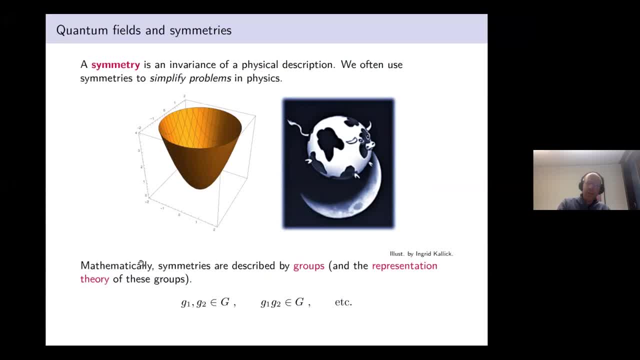 but that's the same problem. mathematically, symmetries are described by groups and the representation theory of the group. so i don't know how much, uh, you might have seen about groups formally in mathematics yet, but roughly speaking they're just a bunch of transformation. 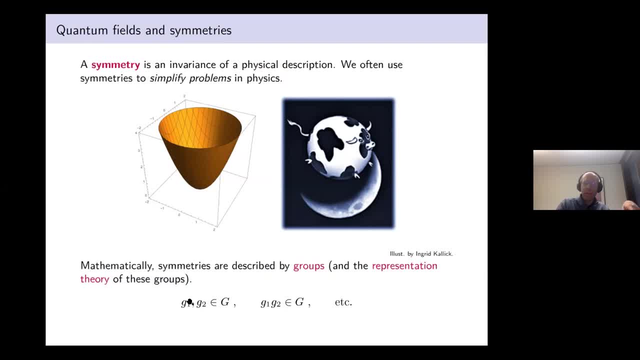 laws and how to to combine them right. so if i have, in particular, one of the definition of a group, if i have two elements of a group g2, i can multiply them and get a third element of a group. for instance, if i have rotation in three dimension, i can go rotate along one axis. rotate along the other axis is the same as doing. 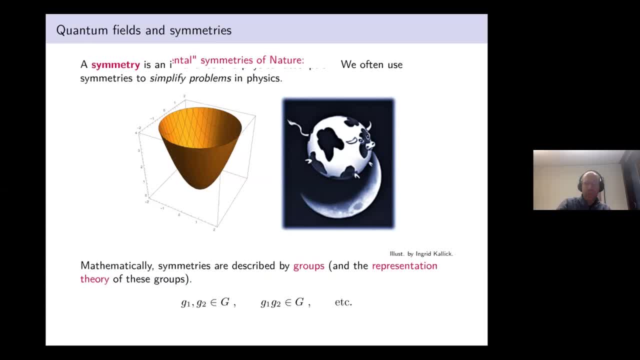 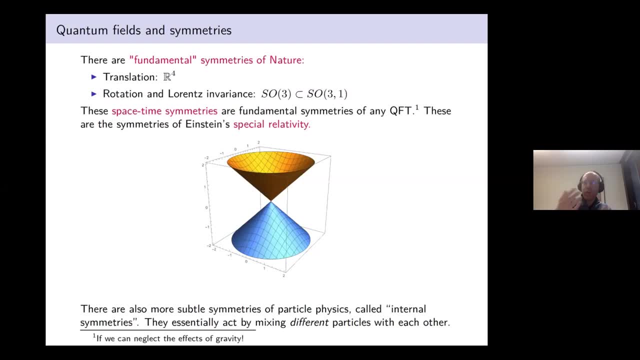 a rotation along the third axis. so in general we can just use symmetry to try to simplify. maybe the symmetry is not an exact symmetry of the problem, it's just an approximation and so on and so forth, and it's a game we we try to to to play it from the start and it's an important 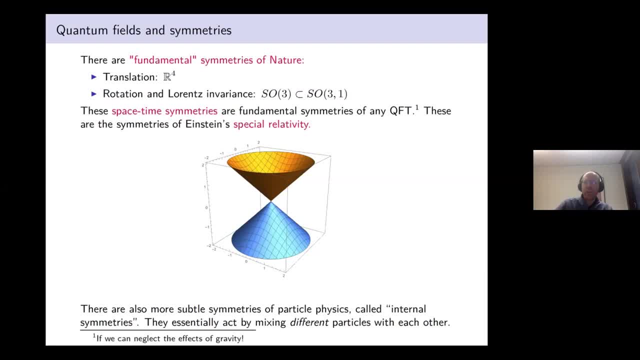 part of becoming a thesis is to try to rely on which approximately and what you are looking for in this problem. approximation is accurate, to try to get an angle of a problem because in general we cannot solve physical problem explicitly or exactly, but we try to have an approximate solution first. 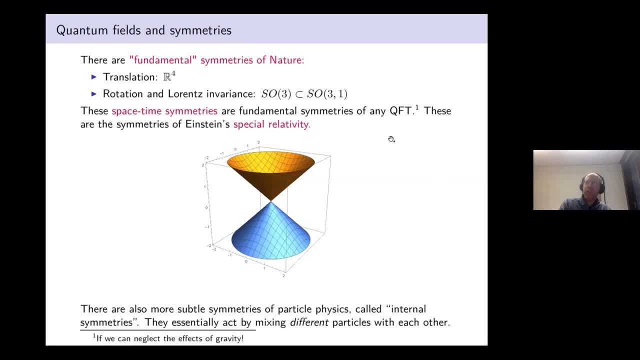 but there are also what we will call fundamental symmetries of nature, because those, as far as we know, are exact symmetries and one of them is translation, so meaning that if there is empty space, we can go in translation a long time or a long space, and the physics look the same. 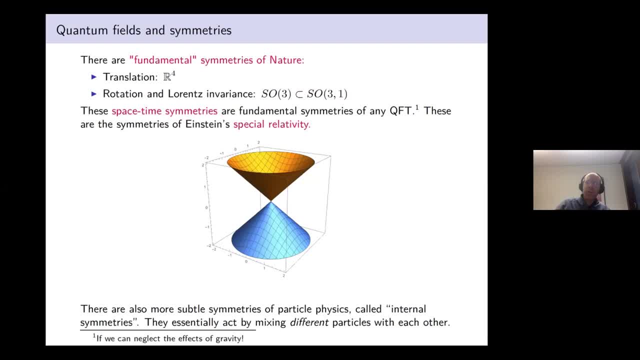 uh, then there is also rotation in space and rotation in space time, which is the variance, which is the the last part. lawrence invariance is the part which was discovered by, by einstein, and that is what is related to causality. here i drew the the light cone of an event, of a person. 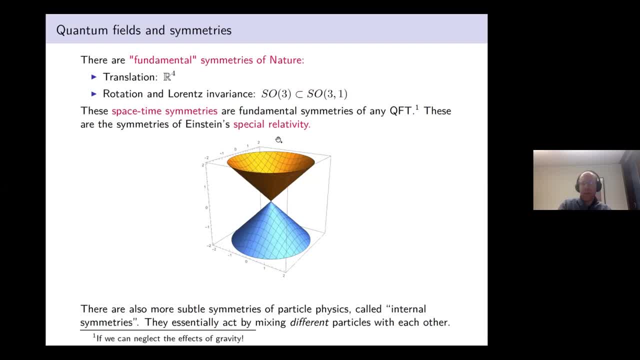 so light cone means that so vertically there is time and horizontally there is space, and light can only go along the light cone because it go at fixed velocity, the velocity of light, and then any information can only go less fast than light, so it has to go inside the cone towards the future. 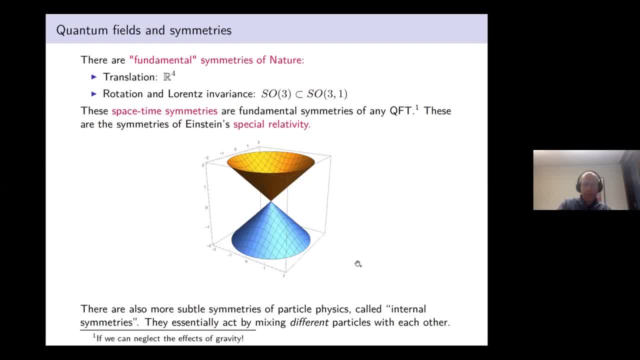 up in my picture. so this is, uh, what we call space-time symmetries, or sometimes a point carry group. so rotation, lawrence, invariance translation. there are also a few more subtle symmetries of particle physics as we know it, which are called internal symmetries. they are essentially symmetries. 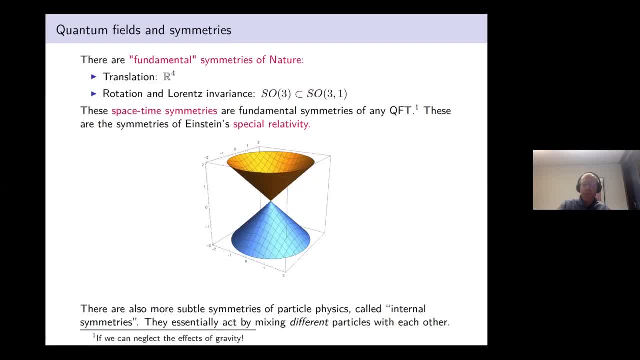 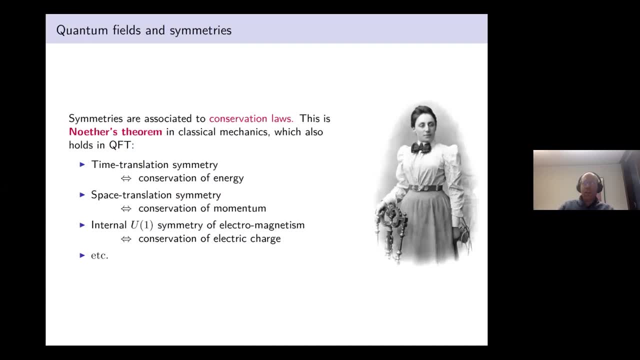 that mix particles with each other. now, any symmetry is associated with the conservation law. this is the, the content of newton's theorem, discovered in classical mechanics as a mathematical statement, in fact, uh, by emmy nutter in the early 20th century. uh, but newton's theorems. 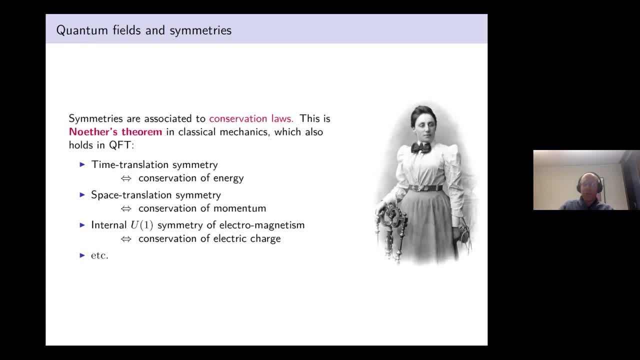 also are all in particle physics, in quantum field theory for instance, it says that if you have time translation symmetry in any physical system, then you have conservation of energy. and it's essentially if, and only similarly, space time translation, space translation symmetry is equivalent to the conservation of momentum, of the total momentum of a system, and for 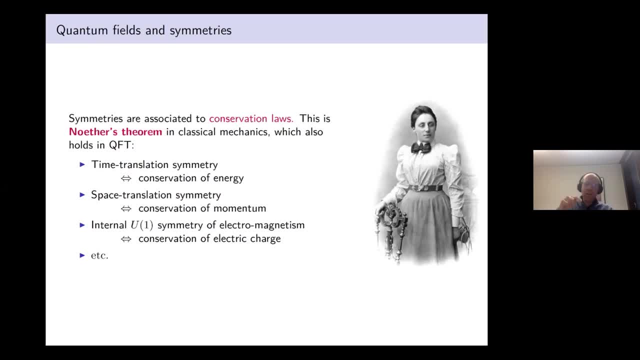 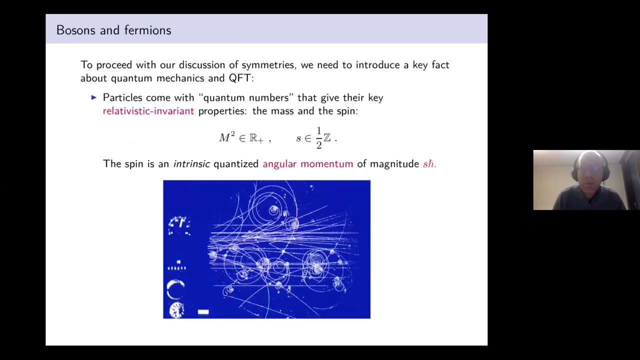 entire symmetries. there are similar conservation laws. for instance, there is a kind of u1 symmetry. that means something that essentially rotates the electron into which, into itself or the electron field, and this is equivalent to the conservation of the electric charge in the universe. now to proceed with my discussion of symmetries, i need to introduce a couple more uh concepts about. 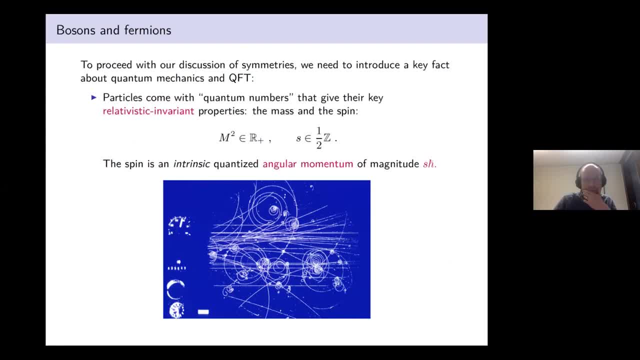 physics, um, which has to do with those symmetries, uh, which is that particles, a given particle, like the electron, will come with just a small list of what we call quantum numbers which are key properties of the particle, uh, which are relativistic invariant. that means that invariant. 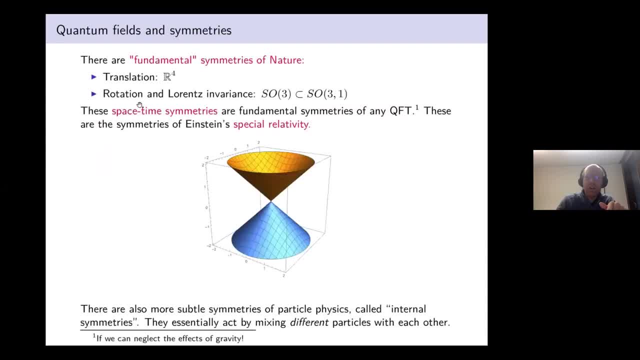 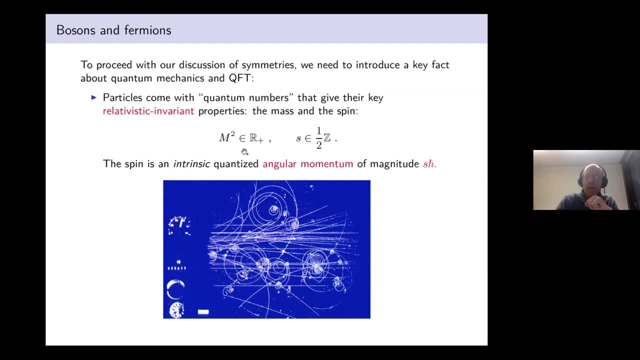 under all this lawrence, transformation and translation and rotation. one of them is the quantum of the particle, is the mass of the particle, um, and the other is: the other is a spin. the spin is some intrinsic angular momentum, as the, as the word spin suggests. so it's, but it's intrinsic to a particular. 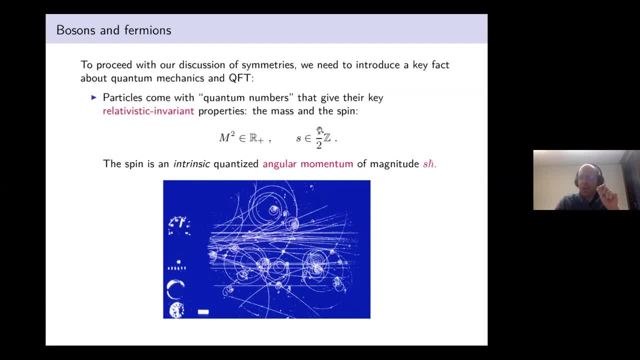 particle and it's uh, it's just an half integer in unit of h bar the quantum of action in quantum theory. so in particular the electron has spin. one half is a spin one half particle here. i show a picture in blue here of uh, what used to be called bubble chambers in in particle accelerators in a couple of generations. 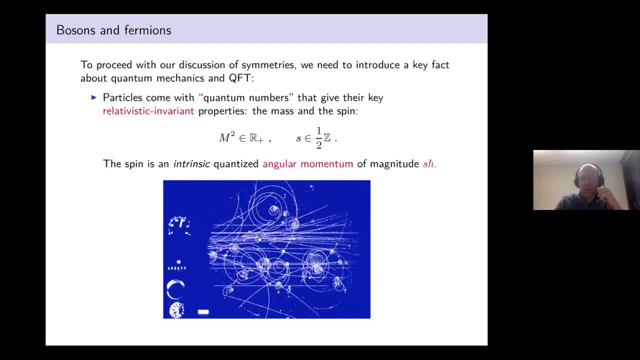 ago already, when you have like something like an electron or other particle that moves very fast in a bubble of water and leaves a trace and because of his spin essentially it starts when you put a magnetic field it starts spinning and doing those beautiful lines. and by looking at the 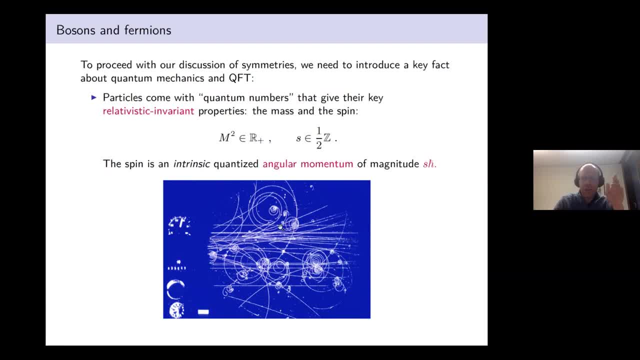 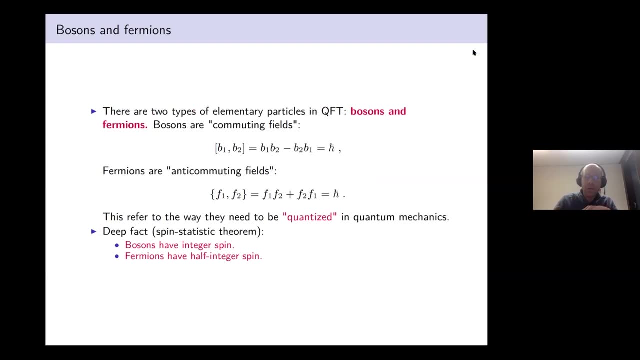 those lines that these techniques like was already invented one century ago. then you can determine things like the spin and properties of the, of the particle and its mass, the, the, the second and, i think, last uh bit of uh of a fact about quantum field theory i want to 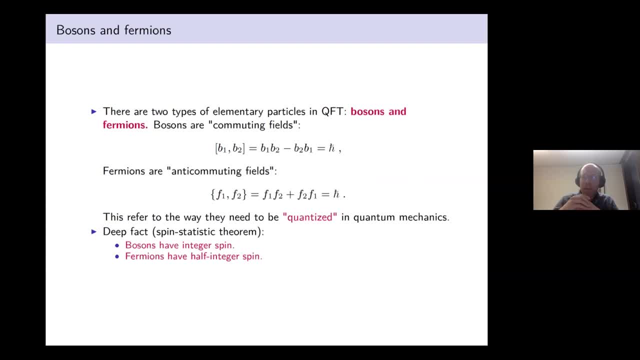 emphasize is the fact that there are two type of elementary particles- uh, of any, any type of particles in in relativistic quantum field theory: the bosons and the fermions, and the. the definition is a bit subtle. it has to do with quantum mechanics and the way 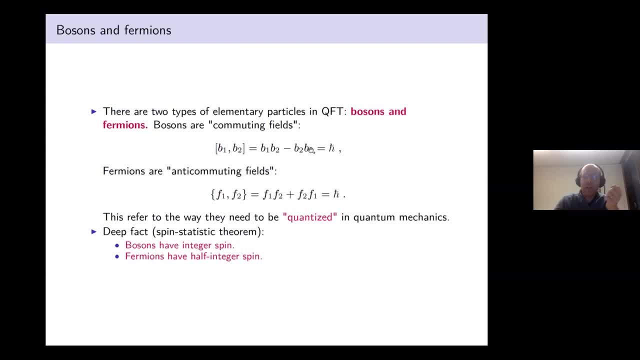 quantum mechanics works is that you can act with a field, because any field is also a particle. uh, and when you act with a field, on the, on the, on the state of all state in quantum mechanics, you can act with one field and and another one, so to speak, b1 and b2 or the other one, b2 and b1, right? 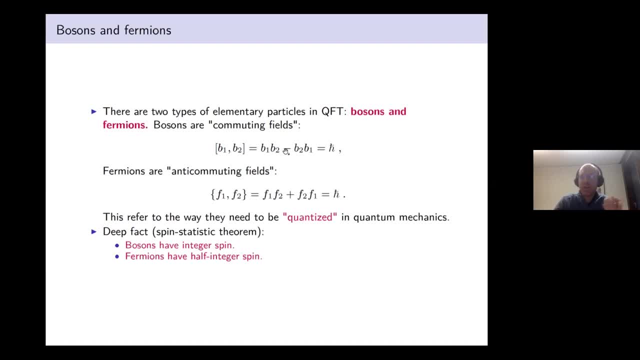 and you can do in one order or the other. classically, uh, we would say they commute. if you get the same result in quantum mechanics, they will almost commute, but they do not. the commutator. the commutator will be given by h bar, and this is for what we, for what we call a boson, a fermion is a. 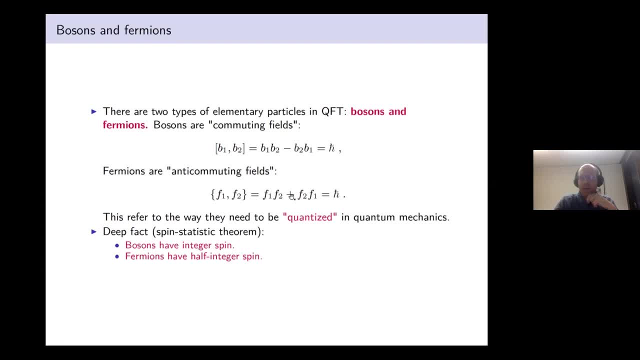 field that behaves almost the same way, but with a plus sign. so if you classically so h bar, when h bar equals zero, uh, you, you. if you put, if you act with a field, and and another one or the other one and the and and the first one, then you get the same result with a minus sign. so this is what is. 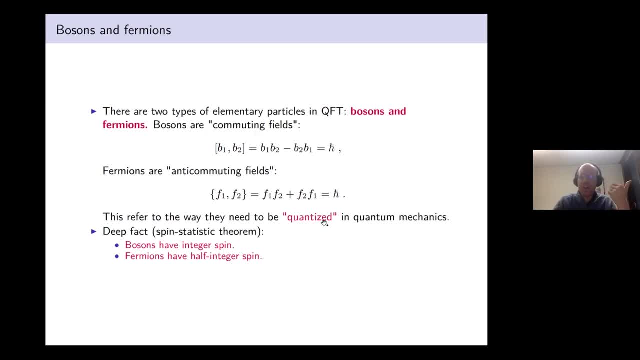 also known as a statistic of the field, and it has to do with how you quantize this uh fields in quantum mechanics and a deep fact that i want that of that is really a theorem of quantum field theory, is that all bosons is integer, spin like spin zero, one or two and the fermions save. 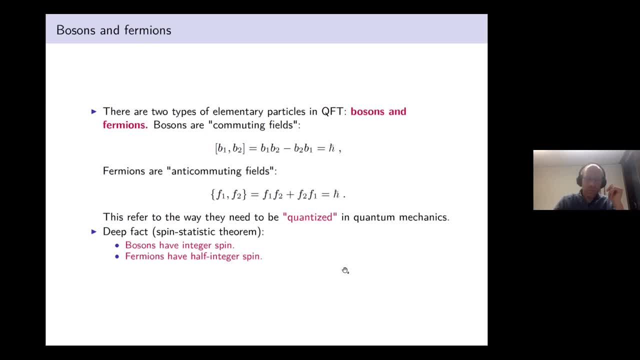 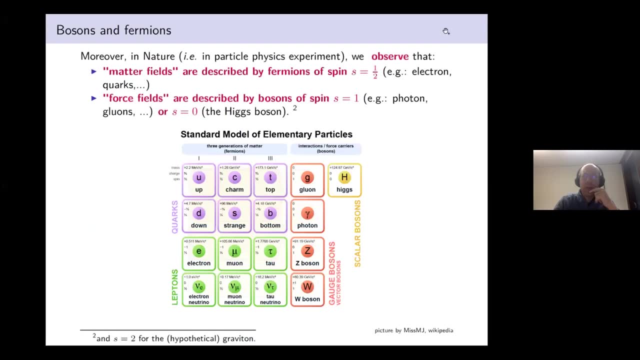 half integer spin, spin, one half, essentially, um in all the case we we care about, okay, and then finally in in actual nature, in the, in experiments we observe that matter fit are described by fermion. we don't know why is the case really, but we just observe that all what we call matter that makes 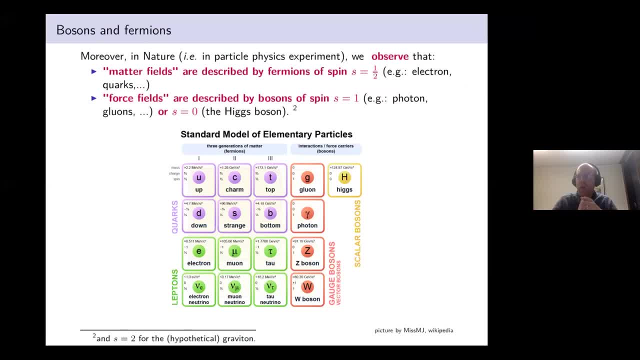 the stuff we are made of are fermions. the electron is a fermion, the quarks inside the atom are fermions. on the other hand, the force fields, the like, the photons that carry the interactions between between matter particles are bosons. so that all the here in in red in this picture there. 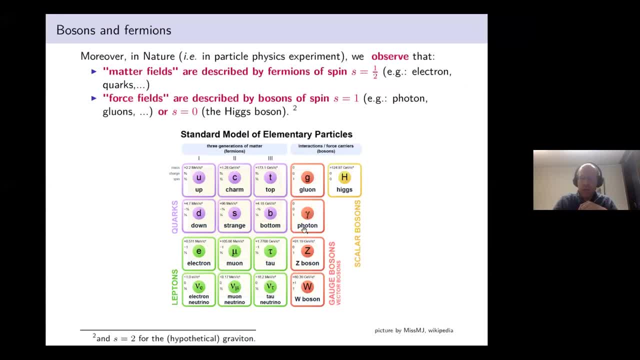 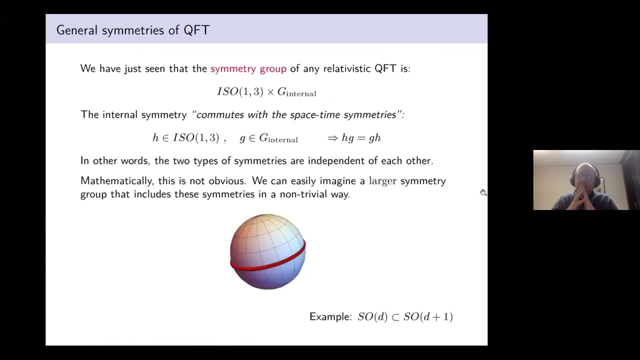 is the, the photon, and there are gluons and other particles, elementary particles for other sources, and then there is one, so those are spin one and there is one spin zero, uh particle, the x boson, which was famously discovered- uh what? eight years ago? um, yes, now we just saw, as you said, that the symmetry 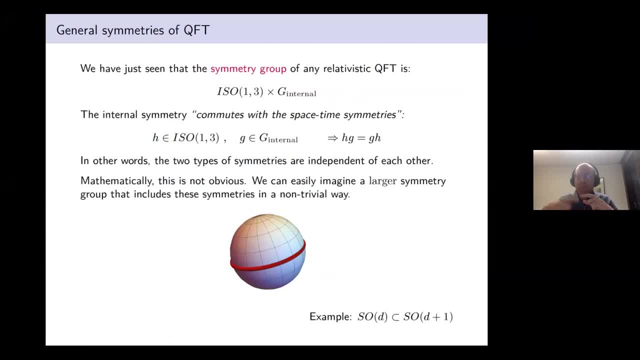 group of any qft is uh, those uh in the space time symmetry times, some internal symmetries and uh, by definition, those entire symmetries we say commute with the state time symmetry. that means that again, if i act with an internal symmetry and then with the, with a translation, 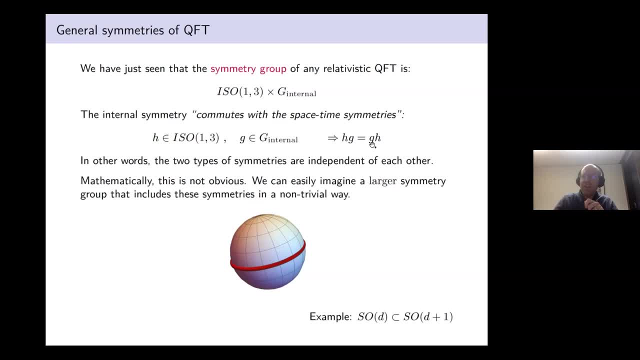 for instance for my first accurate translation. then with the entire symmetry i will get the same result. this seems natural, but it's not guaranteed mathematically. i mean, in mathematics we could easily imagine that all these transformations are part of a larger group. uh, which like talk to each? 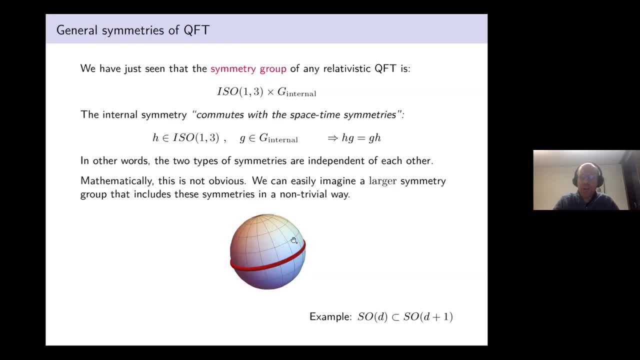 other in a non-trivial way. here i draw a picture of such a, of such a group, group embedding here. if you see this sphere, you can see that there is a group embedding here. if you see this sphere, the sphere is to uh. to uh represent rotation in uh in three dimensions, because i can go along any. 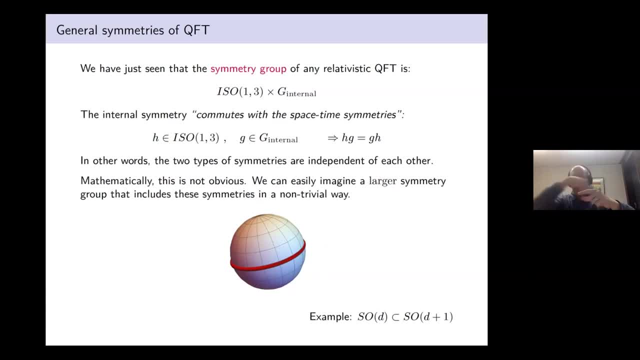 direction on the sphere, like vertically or horizontally. that will be a particular rotation group that we call so3, and but if i just go along the equator, this is just going along the circle. it's a one-dimensional group, but this one-dimensional group is embedded in this. 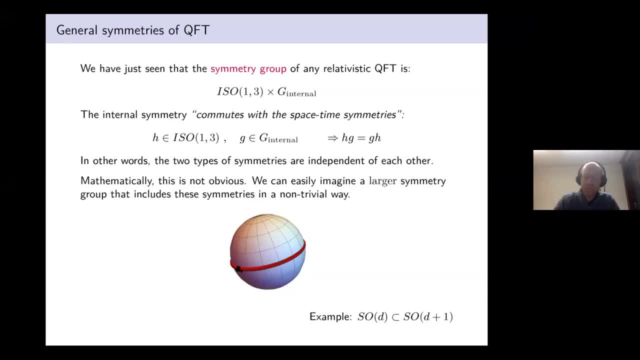 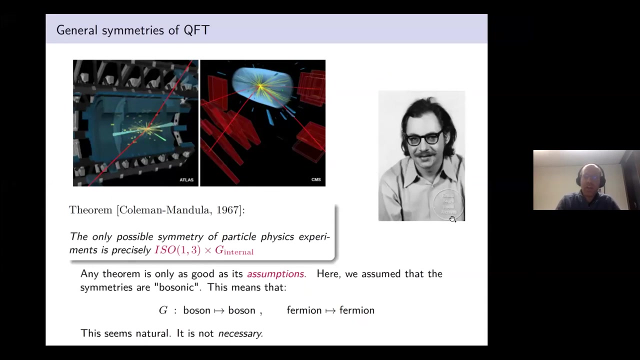 higher dimensional group of rotation and you might think you might ask what is the most general group? actually, i think it's because we were talking a lot about this one-dimensional group, so it's a group that supports an analysis and such two-dimensional groups that that that can be satisfied, that can that by which we transform particles of fields, quantum fields, into. 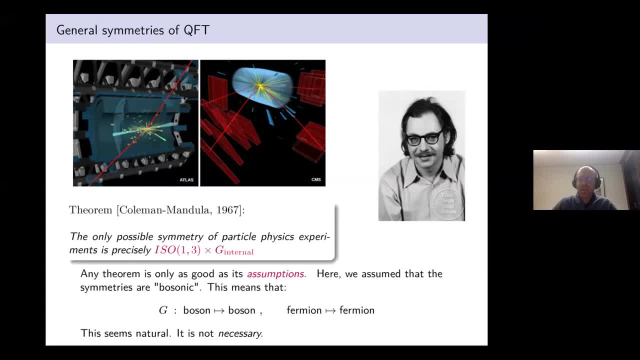 each other in particle physics. so it's a question that people ask: in the 60s, when they were confused by many crazy experiments, when they were finding thousands of new literature, almost thousands of of new particles and they were trying to organize them, and, of course, when we have many, uh, confusing result. 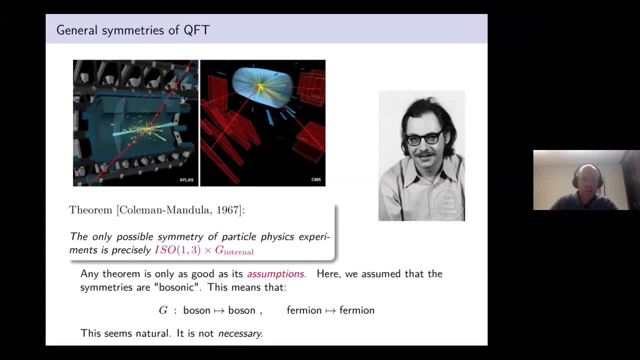 uh, the best thing is to see if there is not the symmetry that would organize this result in a in a nicer. uh, For instance, you know, if you have n particles, but you see it's a vector that transform in a given way under a rotation group, like some matrices and so on, then you're in a better. 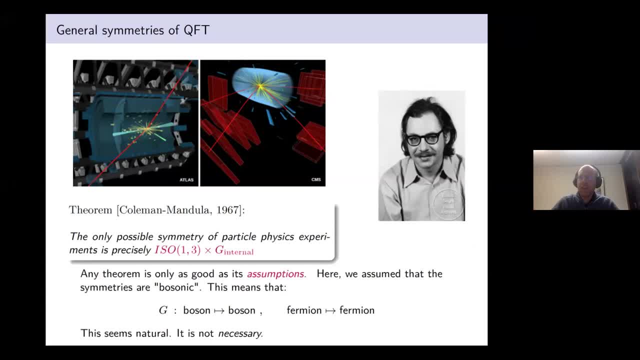 shape, Even though it looks like a very long vector. you understand it as just not n different numbers but a single vector. So the same with particle physics. we would like to understand what is the more general organizing principle, symmetry principle for particle physics, but 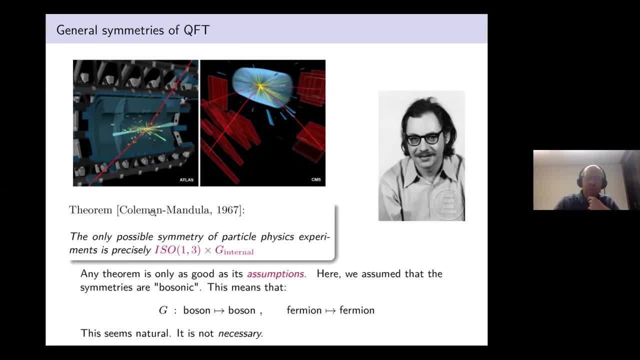 low and behold, in 67, Coleman and Mandela- here is Coleman, here on the right. They proved that in any uh reasonable particle physics experiment the symmetry is that will be apparent will only be the symmetries we just discussed. So ISO 1-3 is the mathematical way of saying. 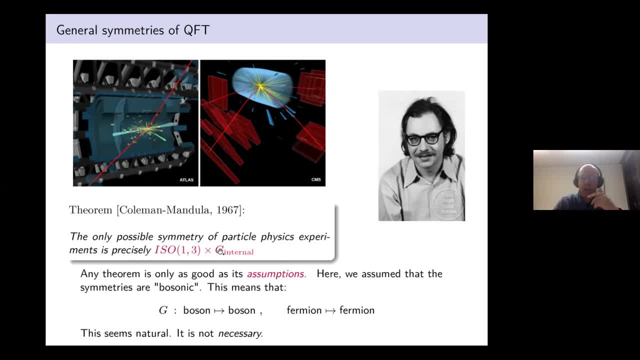 this spacetime symmetry group of Einstein and G is the internal symmetry, G internal. Now, this is a theorem as far as physics theorem go. but any theorem is only a mathematical homework. It's only as good as it's assumptions. And here what they assumed implicitly was: 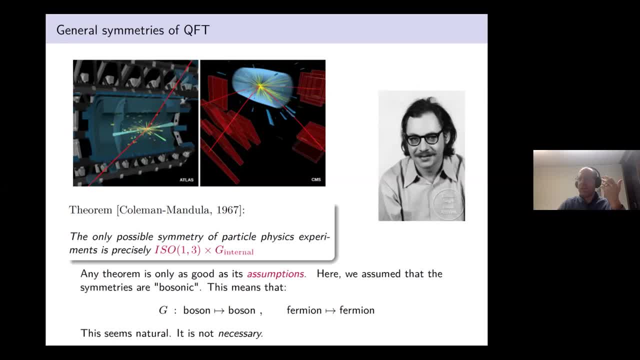 that all the symmetries are botanic. What it means is that it's a symmetry that always sends a boson to a boson. It sends an electron to an electron and the quarks to a quark. Maybe it can send the quark to an electron, but it cannot send a quark. uh, a quark because? 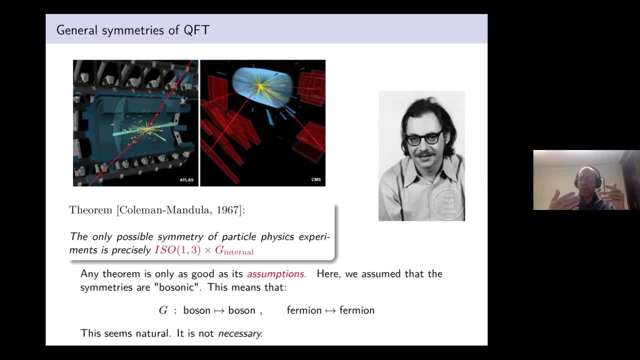 those are the electron and the, and the quarks are both fermions, so it sends boson to boson and fermion to fermion. So it it can send, for instance, maybe a quark to a quark, and 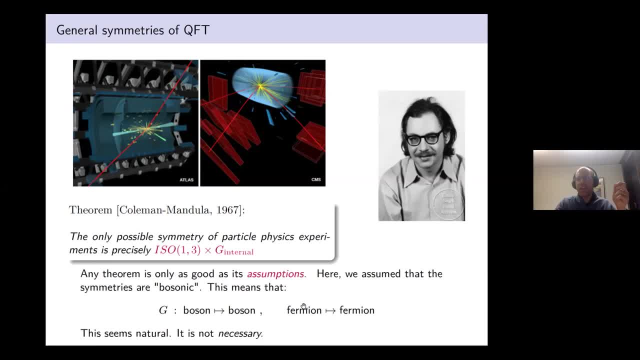 to an electron, but it would not send a quark to a photon because the, while the quark is a fermion, the, the photon, is a boson, as we saw. so this assumption that the, the symmetry is is, is bosonic, so it's sent. it sends boson to boson, ferment to fermion, it's. it's actually not. 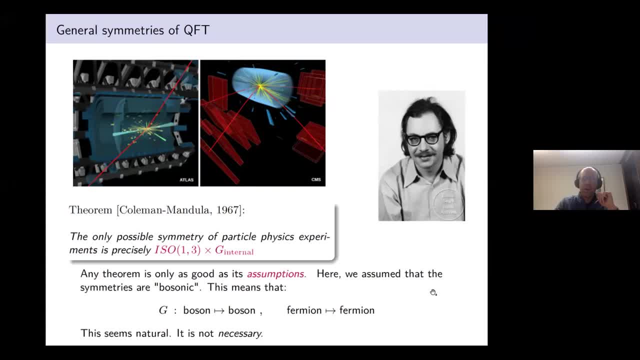 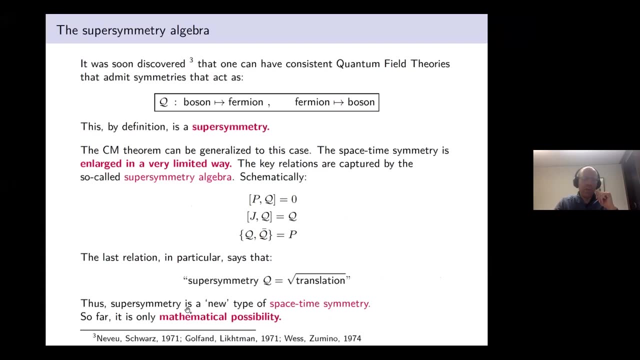 necessary, and that's where supersymmetry comes in as an id, as a mathematical idea at the beginning. it was discovered, in fact, a few years after this theorem, by colman mandela, in 67. uh, so the actual history is a little bit uh confusing. and because it was discovered by 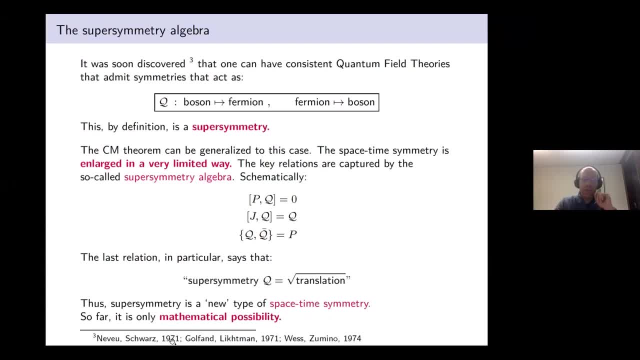 various people uh in 71, both uh in the united states and in the in in russia, and just at the time they didn't really talk to each other, so they didn't really know about each other for a little bit. so anyway, um, by the mid 70s it was well understood by various groups that you had 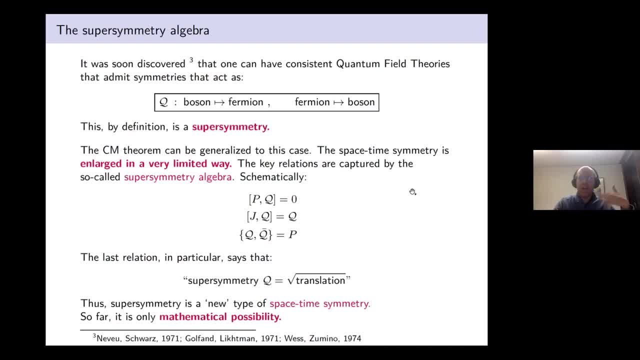 things as supersymmetry and that it could be realized theoretically in quantum field theory. so what is a supersymmetry? it is a symmetry, as you, as you might expect, generalizing this picture here at the bottom right, uh, supersymmetry that i will denote by q in the rest of curly q is any symmetry? 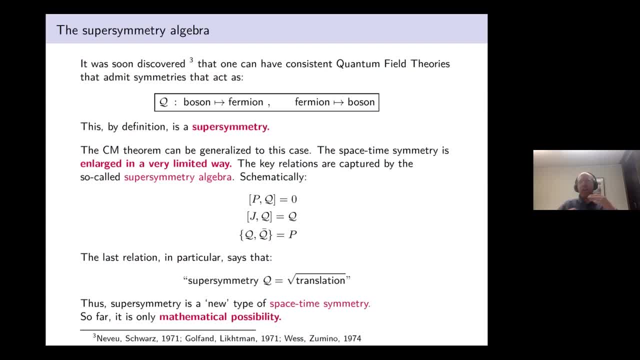 by the definition here that that can send a boson to a fermion or a fermion to a boson. so this seems a bit strange and very interesting, because we just saw that bosons are all the particle of forces and fermions are all the. 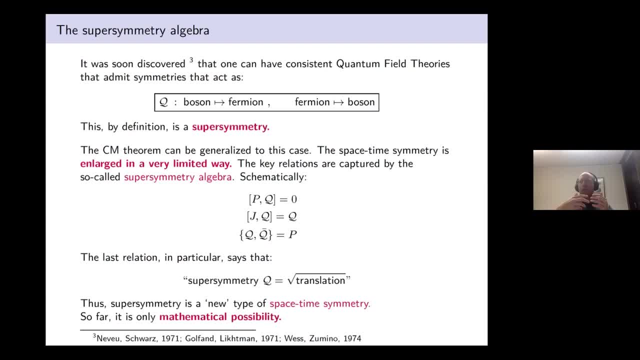 particles of matter. so supersymmetry is really mixing in some real sense, exchanging particles of forces with particle of matter and vice versa. so this is the idea of supersymmetry and the coleman mandela theorem can be generalized to this case um the space-time symmetry in this case is enlarged, but in a very limited. 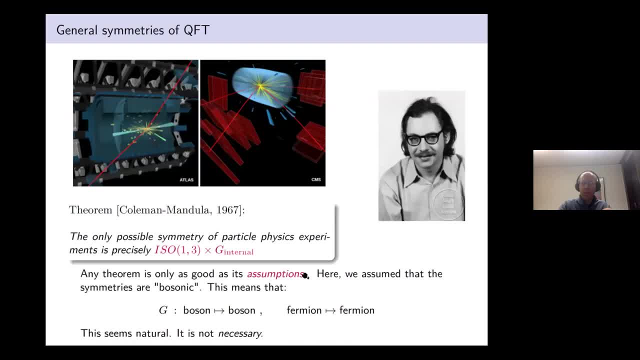 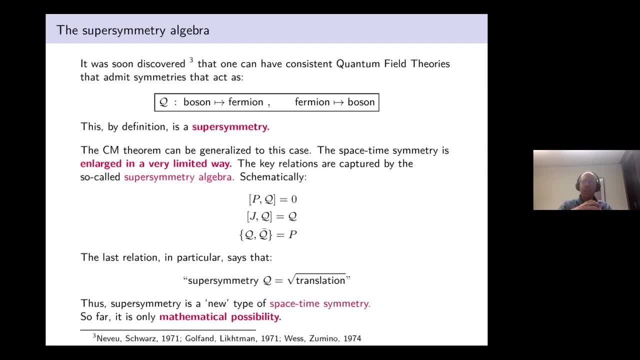 way compared to this result of command mandala. so what will happen is that the space-time symmetry will be part of a slightly larger group, which is called the supersymmetry group, or technically the symmetry algebra in this case, and it goes as follows. so you have you. 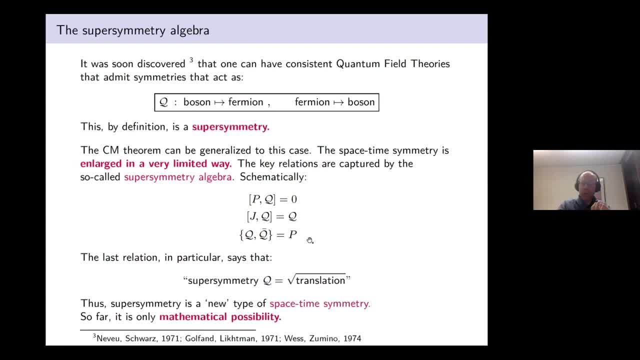 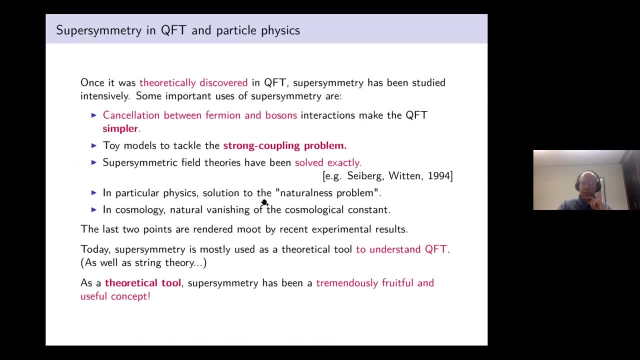 so okay, let me explain this notation here of the three commutators in the middle of this type. so the first, um sorry, the first p commutator with q equals zero, means you can do a translation, do a supersymmetry or vice versa. you get the same result, right? 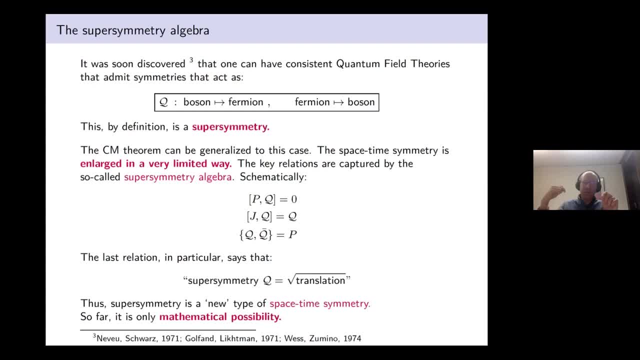 the second one tells you that if you do a rotation, then do a supersymmetry, or instead, do a supersymmetry then a rotation. you will get a supersymmetry. this is related to the fact that the supersymmetry itself will have a spin, and spin is just a type of rotation. 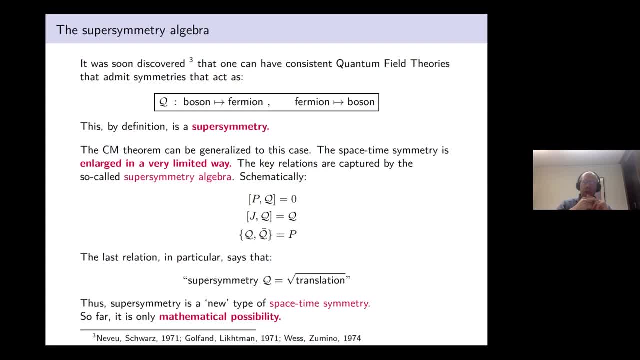 so j here is the angular momentum operator and on the other hand, if you do a supersymmetry and a supersymmetry or a minus supersymmetry and a supersymmetry in the opposite order, what you get is, uh, i mean, if you do a supersymmetry and supersymmetry, then plus the 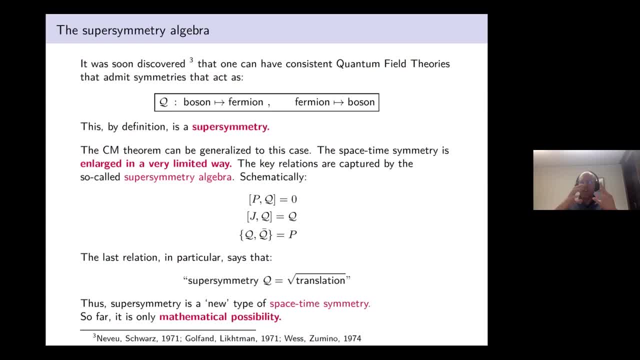 other supersymmetry and supersymmetry. technically, what you will get is a translation. so, in other words, you can act with supersymmetry twice and you get the translation. so, as you can imagine, from the first line right, i told you that q, acting with q, sends a. 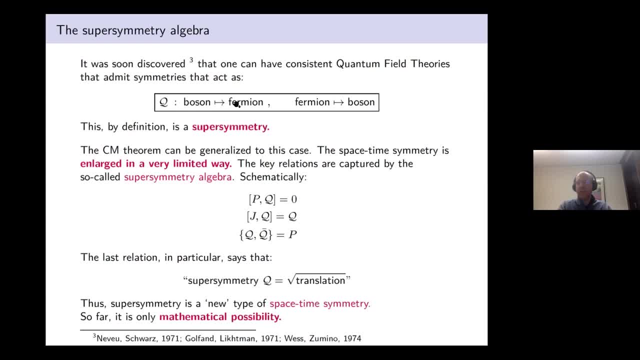 boson to a fermion, then i can act again with q. then i send the same fermion back to a boson, so it goes back to itself, so to speak. well, it gets back to itself. up to a translation. it's what the last equation says. it will get the same boson you started with if you act with q twice. 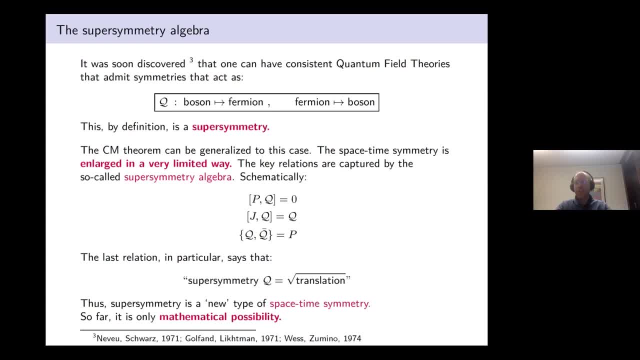 it will extend the boson to the same boson, translated. so in that weird sense, supersymmetry, you can say it's really a space time trans, a space time, uh, a space time symmetry of a new kind which is, as you can see, morally speaking from this last equation in the middle, it's a square root of 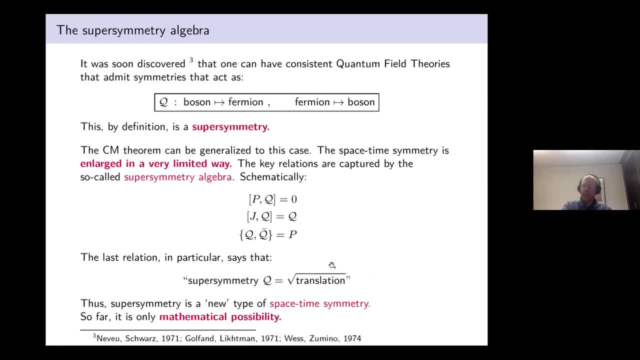 a translation. i mean, it's a slightly imprecise way of saying it, but maybe it's a more striking way of of seeing that the supersymmetry is just a slightly more subtle type of space-time symmetry that we didn't discover until the mid-20th century, like galileo already knew about translation. 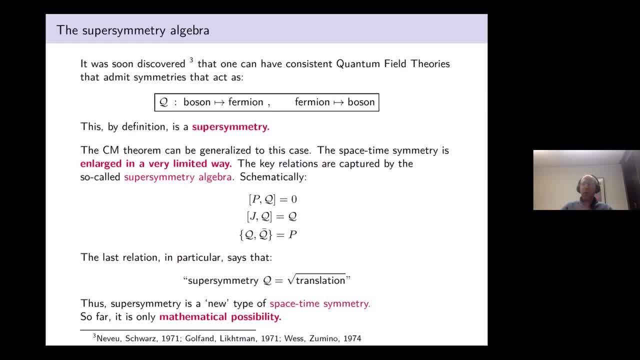 he had all this beautiful picture about our uh balls in in. uh balls that you throw away in a in a standing, in a in a moving ship will fall at the same rate, at the same place as if you, you, you know you throw it out in uh in on on the if you're not on the ship, and and so on, this kind of thing that. 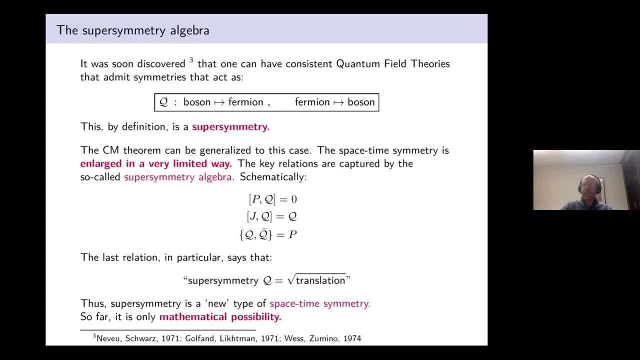 this game that we we do with trains now in in first year physics, uh, so this kind of thing, were not intuitive, but they were. they were well understood by the by a few centuries ago and uh, and then einstein in the 1905, understood all the symmetry was space time. 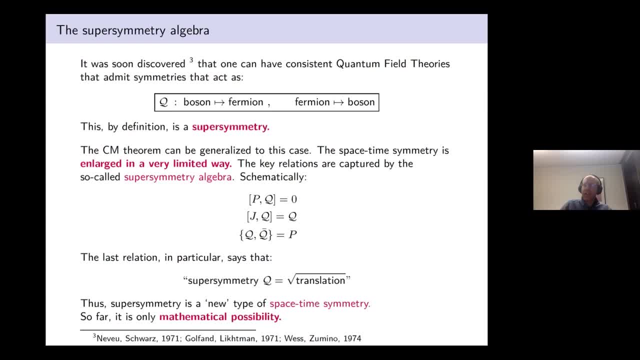 which are bosonic, but then we and those are realized in nature. but then thinking about it just essentially mathematically, uh, like first principles we cannot. we came up with a notion- i mean people in the mid 70s that i quote in the bottom here, especially western domino. 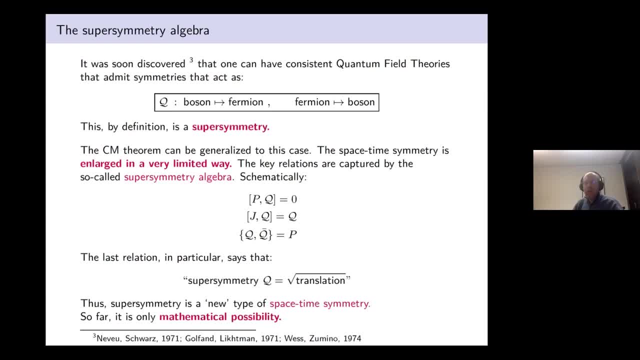 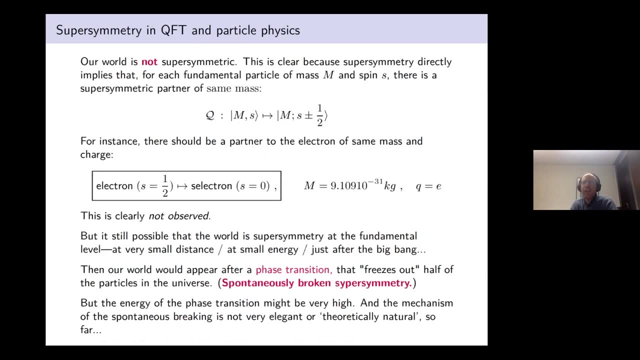 uh at cern in the in the mid 70s, understood very precisely that there was a new type of space time symmetry called supersymmetry, which is this kind of weird square root of of rotation that mixes and fermions. now, this is. this was a theoretical discovery and then, of course, being physicists, the 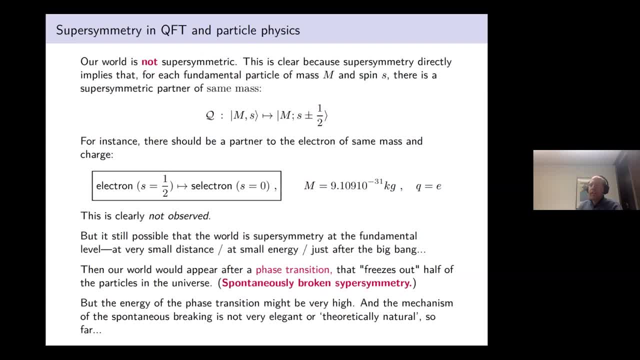 people who discover that and the mathematician. they always. they thought, oh, this is so beautiful idea, and so on. it must be realized in nature. we will just try to find how this is realized in particles, physics, and we've been looking for a while, for a couple of generations now, and we were 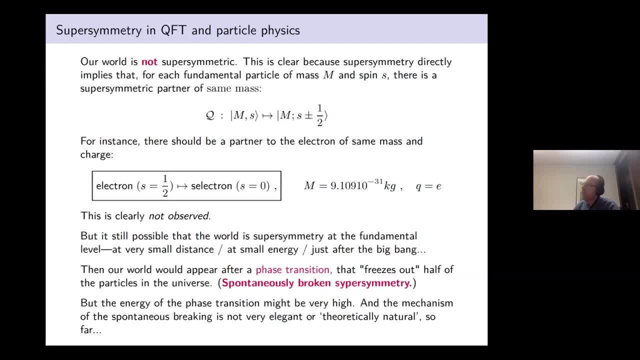 pretty hopeful that we would discover symmetry in particle physics. uh, maybe in the 90s, and then at at lhc, at cern, in the last experiments over the last few years. but so far no luck. uh, it has not been observed. so there is a good reason why it's not obvious that it should be observed. of course, 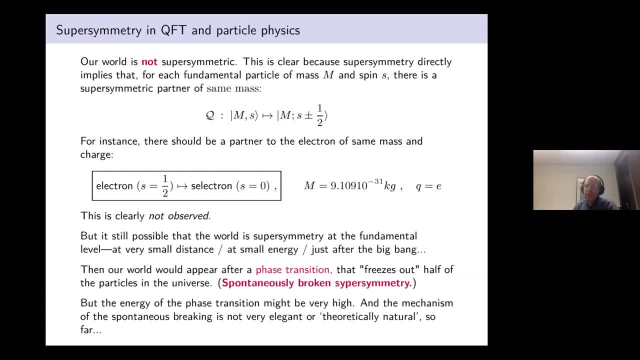 our world as we see it, we already knew from the start that it's not supersymmetric, sadly maybe, sadly, i mean, although thankfully for us, because chemistry would be very different if we have supersymmetric particles. but it is clear though, our world is not exactly supersymmetric because of essentially this supersymmetry. algebra i: 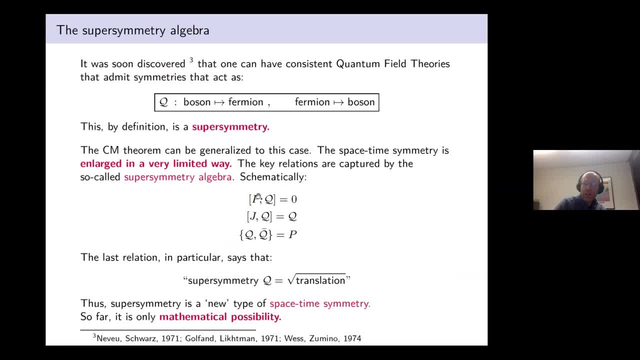 showed you. here you see, the first, uh, the first equation is telling you that momentum and supersymmetry commute. but momentum in relativity is essentially the same as the energy of the particle. i mean, it's related to the energy, the momentum squared, although what i call the mass. 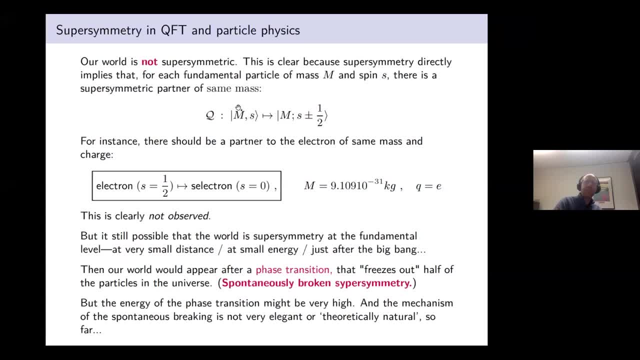 here the mass is the intrinsic energy of the particle, and if the moment, if supersymmetry commute with momentum, then it means it commutes with the energy of the mass of the particle. and so if you act with a boson of a fixed mass here and a fixed spin, 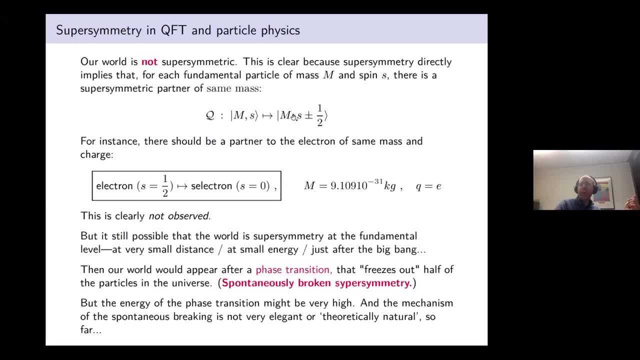 the supersymmetry sends you to a fermions of the same mass, and so the spin shift by one half, right? so if you have a fermion, spin one half, you can go to spin zero or spin one. and if you start with s equals zero, spin zero, you can get to a fermion on spin one half, but the mass is the same. so 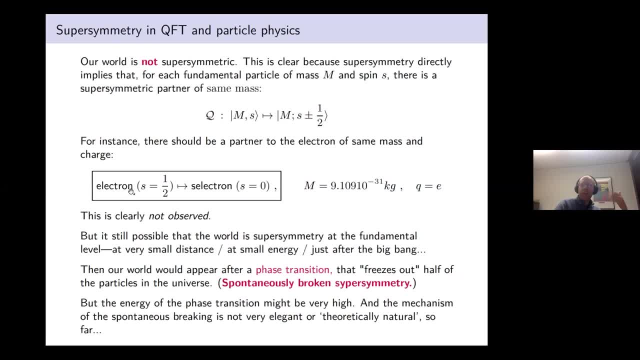 if supersymmetry is an exact symmetry of nature, each time we have an electron which has a fixed mass, of that we know experimentally to be this tiny number right nine point one, uh, ten to the minus 33 kilograms, uh, then there should be such a thing as a selectron, which would be a particle. 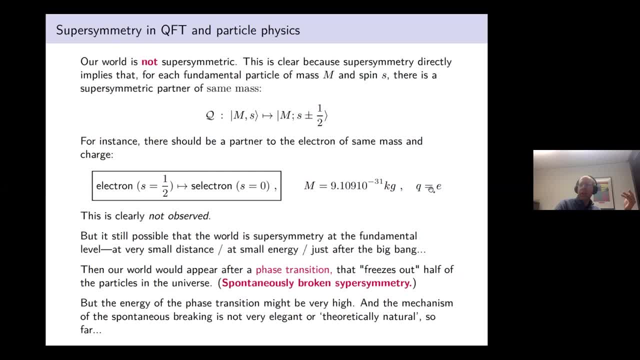 which has spin zero and the same mass, and it should also have the same electric charge as the electron. but if there was such a part, a light particle, uh, with electric charge, one like the electron, we would have discovered already. i mean, the world will be completely different. 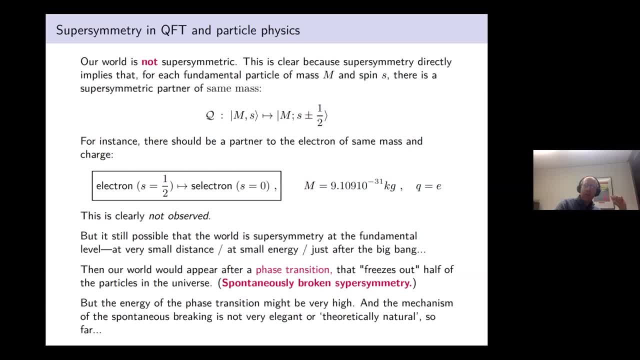 so it's not such a thing as exact supersymmetry in nature, but of course people knew that from the start. but the idea was that maybe our world is not supersymmetric, uh, in everyday life, but it's completely imaginable and it can be more precise that the world is supersymmetric at the more fundamental level. so if we go very, very 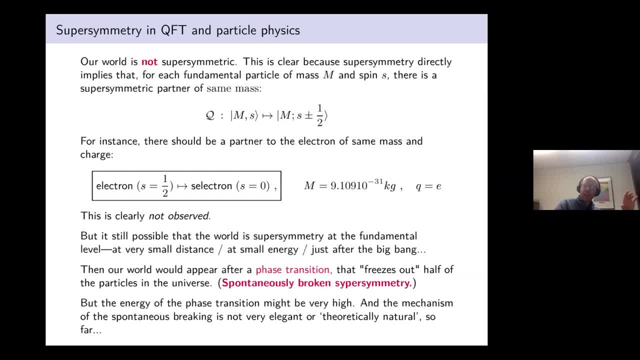 small distances, which means very, very large energy, or in term of the history of the universe: very early, very soon after the big bang, when the universe was very hot and dense, maybe the world was supersymmetric. and then what happens is that there is something that we would call a phase transition, like when the liquid becomes a solid. 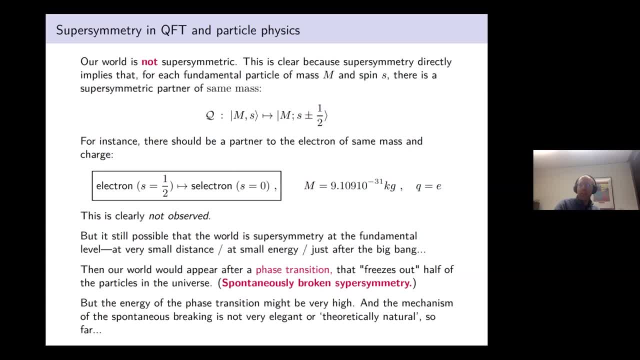 right, uh, like when water becomes ice. so supersymmetry then would be the symmetry of this, of water. but then, when you, the universe becomes like dark and boring, like today, the the symmetry freezes out and we, we, you're left with a non-cybersymmetric world. 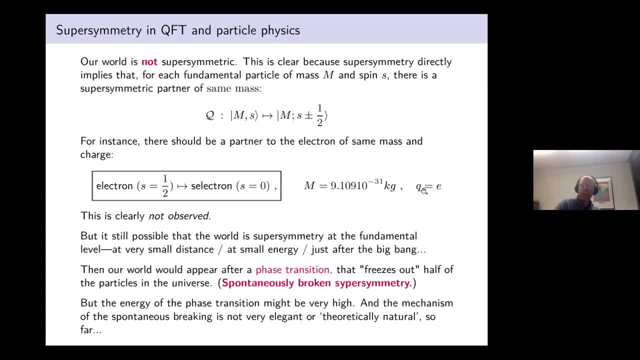 this uh of phase transition scenario is called spontaneously broken supersymmetry, and this can happen in very stereotypical scenario, the the catch is that the energy for this situation might be very high. it might be just a tiny moment after the big bang, and then it's very hard to recreate the condition for supersymmetry. 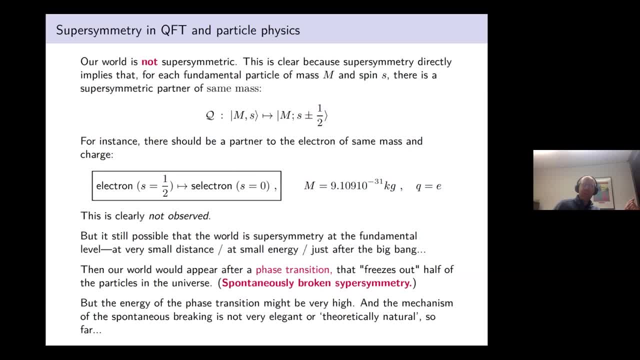 in particular accelerators. so we were hoping that if supersymmetry, this breaking of supersymmetry, is relatively, it would be very high energy, but it could be low enough that we can actually reproduce this energy at CERN or at SLAC or other particular accelerators around the world. and so people are looking to 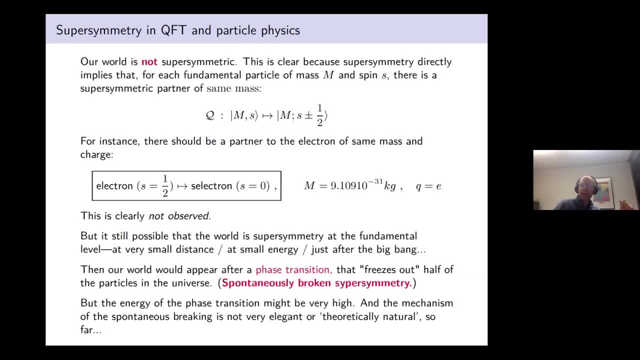 observe supersymmetric partners when you go to high energy, higher and higher energy in particle physics experiments. but, as I said, we had no such luck. we had some reason that were never completely airtight to hope or like be well motivated, uh, thinking that we would find supersymmetry. but 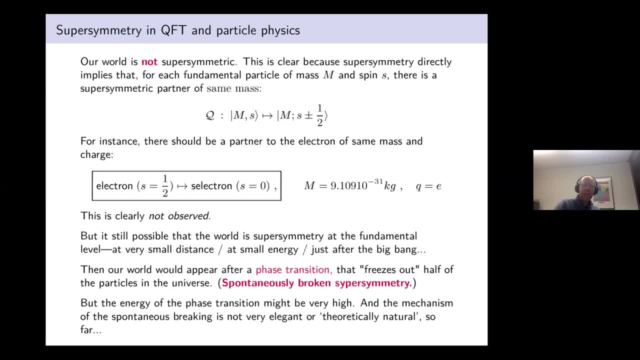 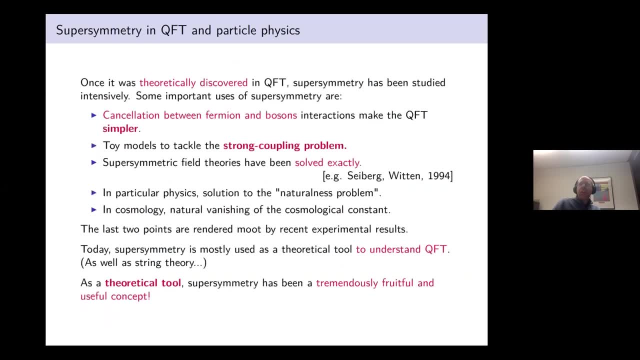 maybe those reasons were not that good and they were not like mathematical deep reason. uh, there was always a bit of philosophy to it and so we were not so lucky. nonetheless, of course, supersymmetry, I mean theory theorists will not let the experiments I mean we know only recently like experiments. yeah to that silver supersymmetry, but back then in the 70s. 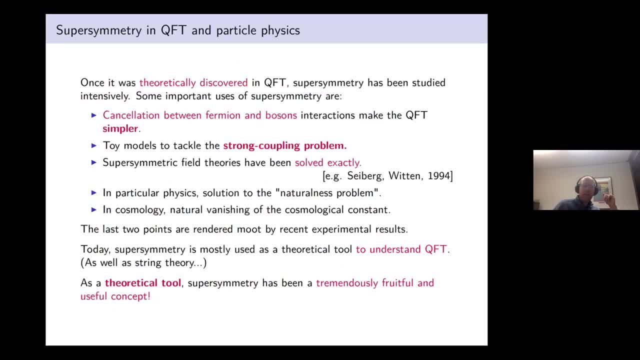 people thought, okay, maybe we'll find it in 10 years, and then so far we waited almost 50 years. but in any case, theories don't really wait for the experiments through their work. they just work on whatever they find interesting and and fruitful to do: new type of computation and so on. and so why once supersymmetry was was? 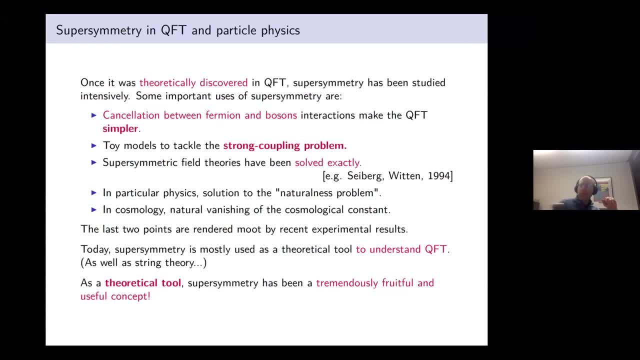 directly discovered. um, I realized that I'm. I will go a little bit away over time while you tell me when, uh, when, when I should stop. um. supersymmetry, then, was studied intensively in the last few decades, um, and one of the important uses of symmetry that I want to emphasize today. 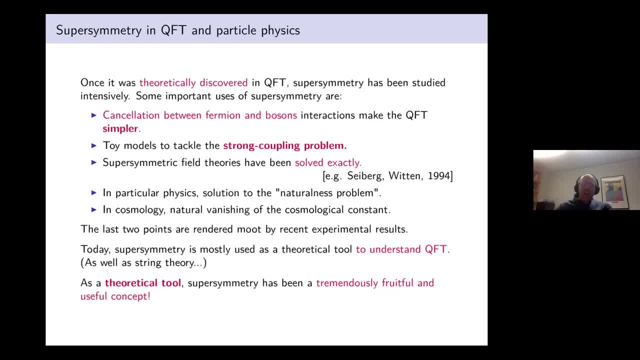 is that in the penalty of whatever, sorry, in the penalty of whether supersymmetry is realized in, in the, in the world, in particle physics, in nature, it's very interesting theoretically to tackle problems, conceptual problems that we have with quantum field theory, like these trunk coupling problems I was telling you earlier, and I will conclude with uh in a at the end of the talk. 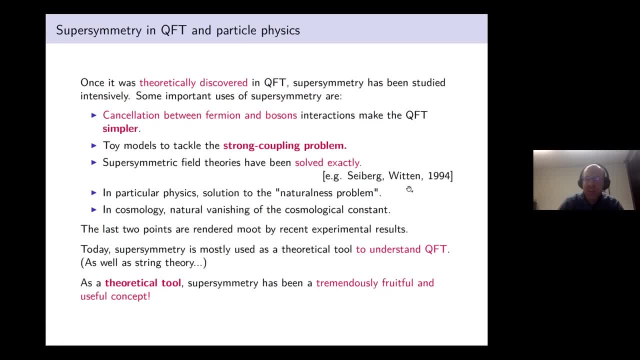 I want to discuss a little bit how we use supersymmetry. I mean I, we, I mean collectively humanity and in particular saber and ritter in 94 used supersymmetry to solve a particular type of quantum field theory which is strongly coupled. but they use symmetry to solve this and without 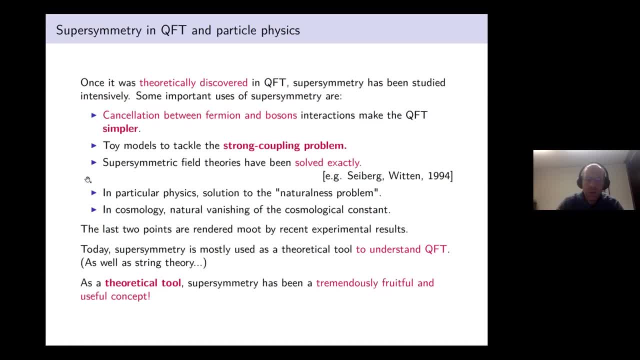 supersymmetry. we would never be able to do this kind of huge computation. there was also the last two point about particle physics and cosmology. is that, at least up to relatively recently, the over the last, up to, uh, 10 years ago, there was good reason to think that supersymmetry 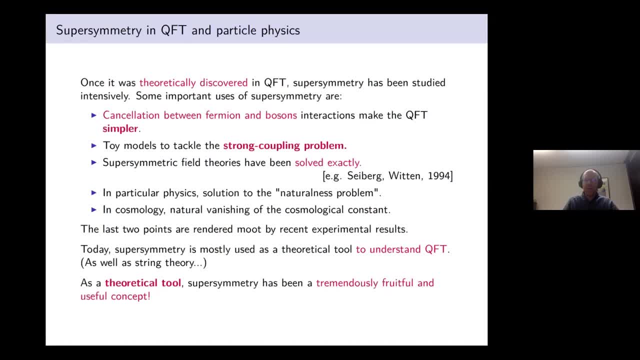 uh, would give solution to various puzzles in cosmology and particle physics, but i think so far those ideas have not been successful experimentally. so that's why, as a theorist physicist who lives in the mathematical physics building, i really think of of supersymmetry as a theoretical tool, and that's what i would like to emphasize in the 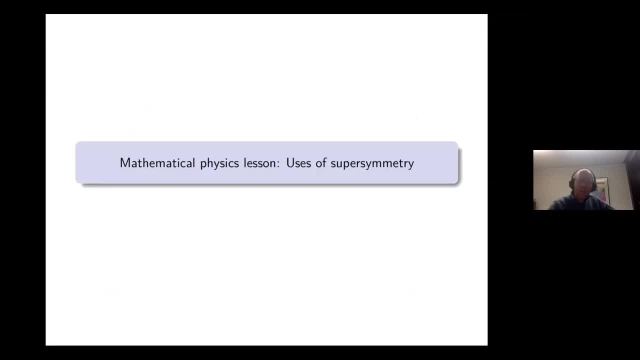 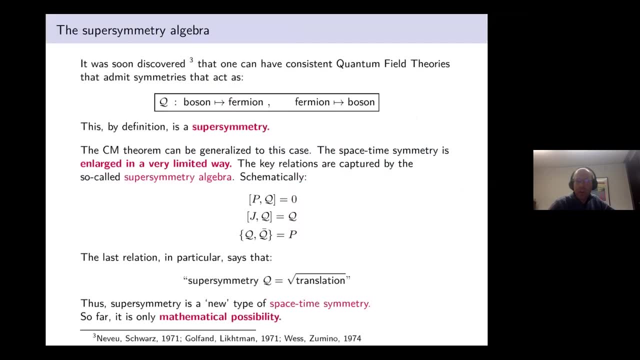 the remaining of the talk. so this was the the history of particle physics, and now super symmetry arise and what it is in particle physics or, in broad terms, in physics. so if there are any questions about that, before i go into a slightly more mathematical part of the talk, 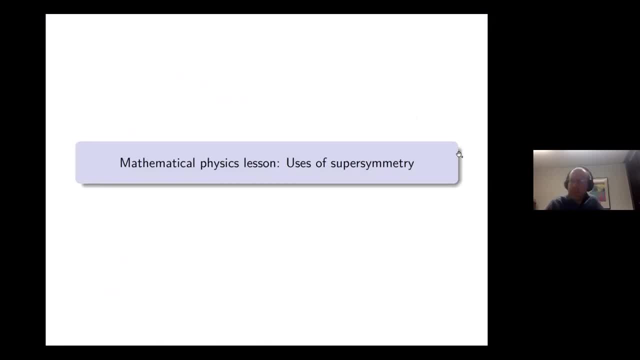 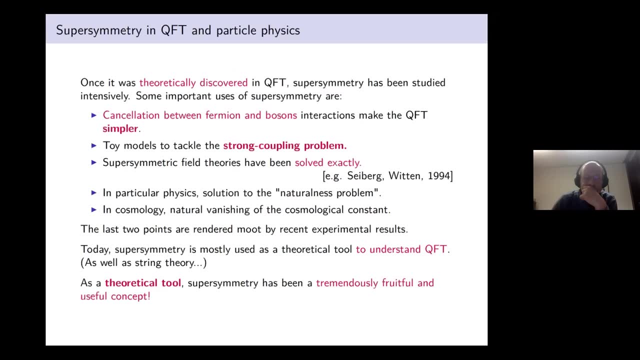 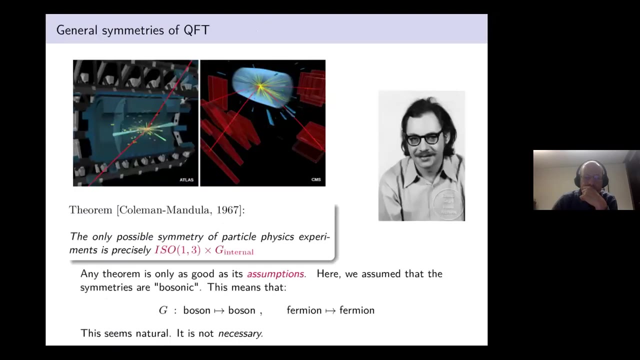 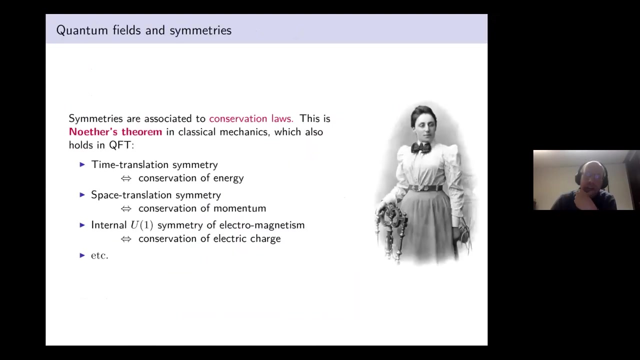 okay, uh question, yes, yes, um, so you said that a symmetry implies, uh, a conservation law by nurses theorem, yes, so what is conserved in supersymmetry? very good, so i mean there is a conservation. there is another term for supersymmetry, it's called a supercharge. 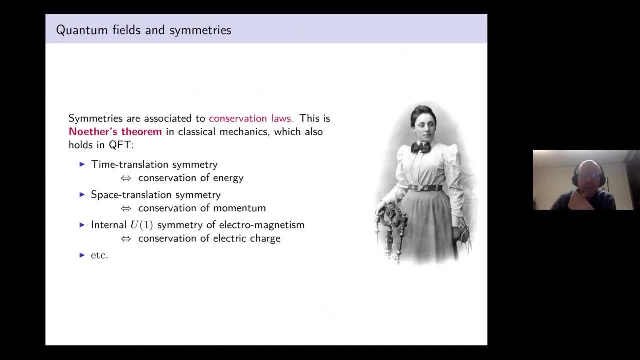 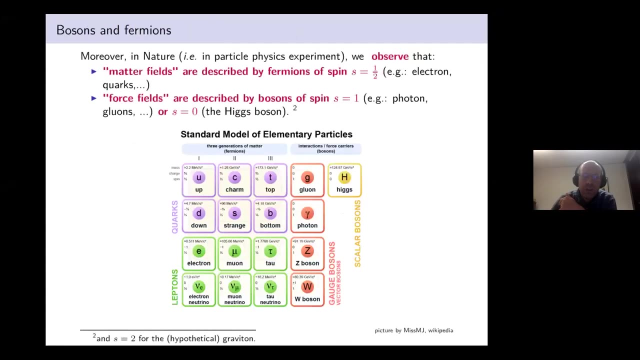 and uh, yeah, so the thing is, it's not something that you would know, because, well, first of all, we don't have supersymmetry in our world. um, but yeah, there is, mathematically, an object which is the super charge, and in fact, the super charge is what i call q, because what is a charge? 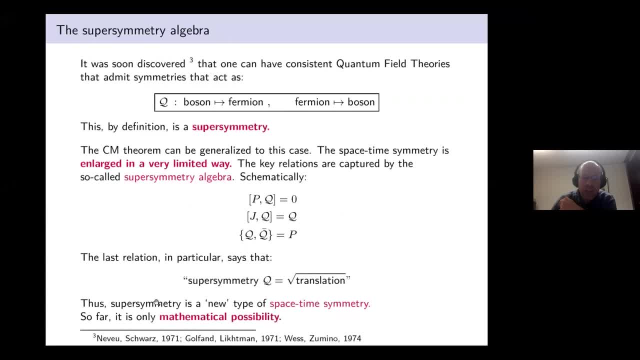 is essentially an element that would generate a transformation in the group, and this charge is conserved, like the electric charge is what generates this kind of internal symmetry of the electron, and here q is a charge, is what we call the super charge, and that's what is conserved. so 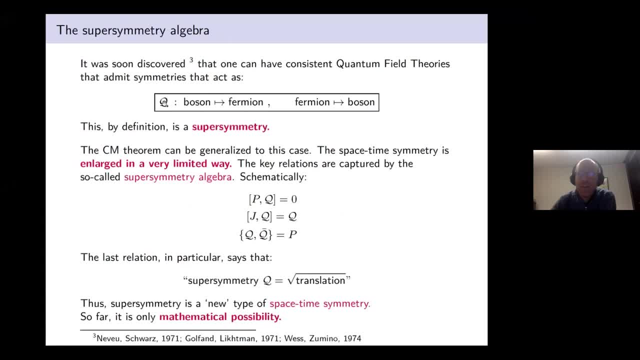 meaning that this is a part. q will be essentially, concretely uh, some kind of uh, complicated function that you build out of fermions and bosons, you know in a qft, and this particular combination of bosons and in a supersymmetric theory will be time invariant, so it will be conserved. that's the 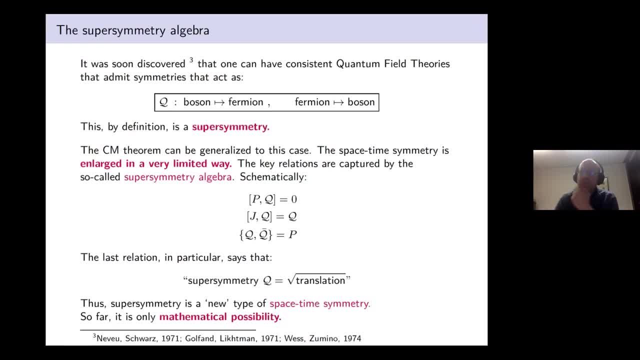 that's the super charge. yeah, so is it like it's not a particular property of one particle, or like some complicated function? well, no, i mean, it is the general property of the. okay, it is the general property of the system. a super charge, um, but in the same way, this. 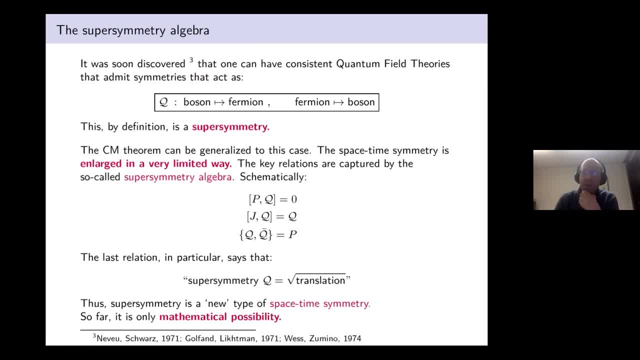 translation: invariance is a general property of the system. and then you can, in quantum mechanics, you can always realize those charges as some kind of operator that is built out of the of the particle in your system, and you always start to get acting. a particle, but it's a particular. 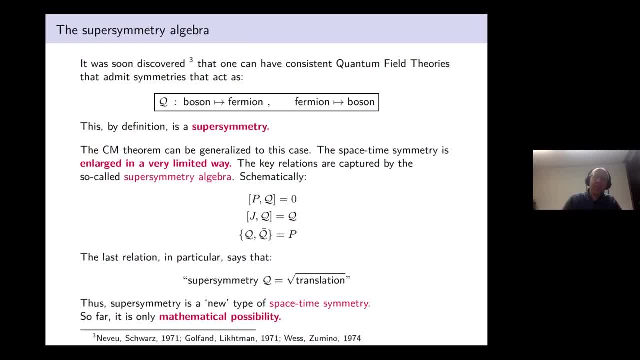 yeah, but anyway it's a. it is a just a particular property of the system. it shows that because it's a thermionic charge, it's it's not something you are like conservation of energy. there is a concern in that same sense, except that it's less intuitive. i mean, it's not something we. 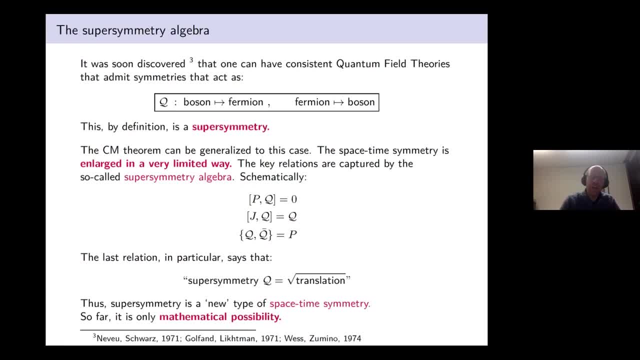 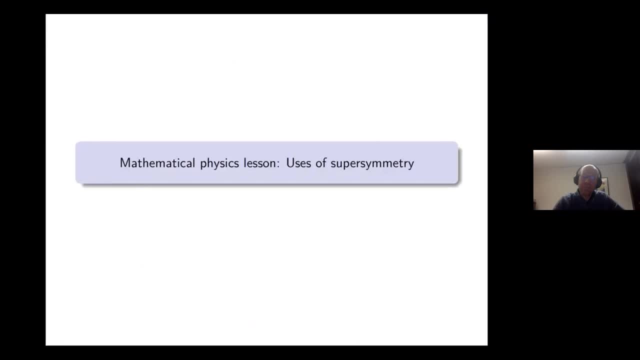 see in in the real world. so, but yeah, they will be nonetheless neutral. current is still still, is still true, and so there is a concert supercharge. okay, any other question, all right. so, um, let me then go through, uh, slightly, the less technical, the more technical part, i thought. 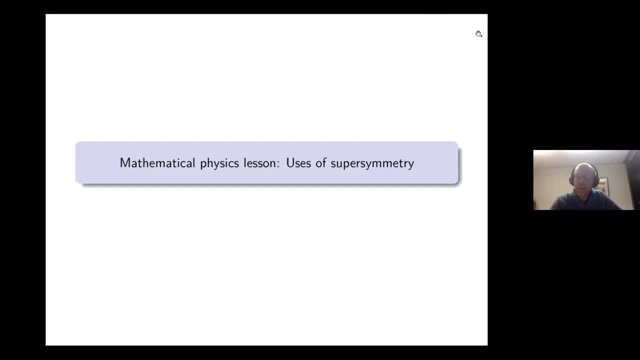 you know, when you do this kind of uh, when you hear this kind of talk, i mean i remember reading about string theory in books and so on when i was in first year or in high school, and there is a thing when you can only do so much right, without equation. and then when they, when 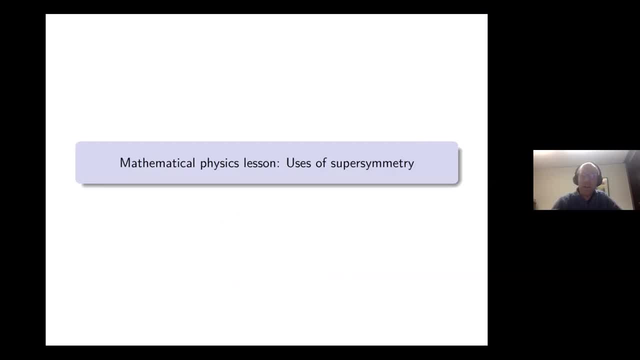 people write like physics book. the editors will always tell them that you use half of your readers. each time you write an equation, uh, i think the only person who sold books with a question in it- and i'm not talking, but we are also among you- know oxford students, so i will take the risk here. 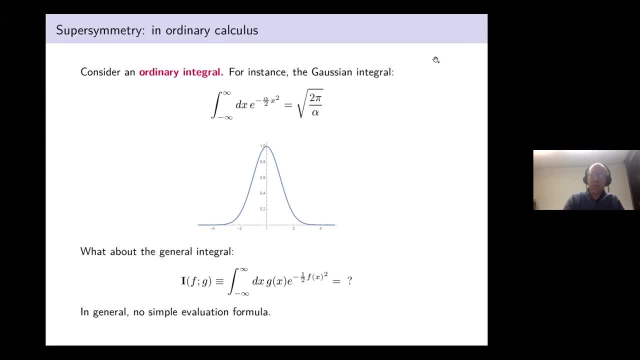 of assuming that you would like to see a little bit more under the hood of what is going on with supersymmetry. so i will like show, like a sort of toy, model of supersymmetry when you can see all these. supersymmetry helps solving problems using a model of supersymmetry in just ordinary 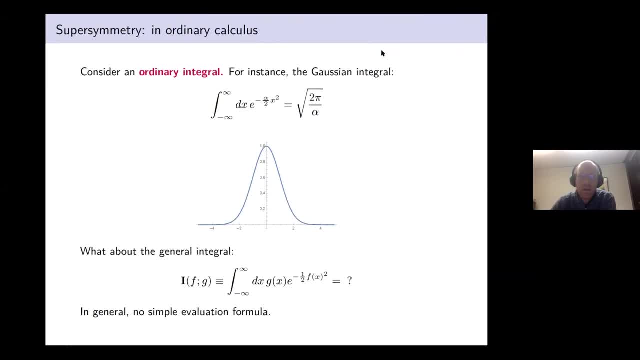 calculus. so let me then, sorry, where is this? yes, so you see here, uh, this particular curve, this integral, so the the volume under the, the area, under this curve, this integral, e to the minus alpha over two x squared, an exponential of x squared, that you probably seen that in, uh, in some calculus. 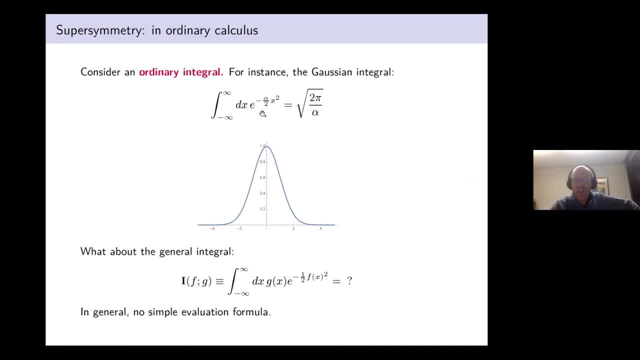 exercise or to solve this. uh, if you do the integral from minus infinity to infinity, so the whole volume under the gaussian is square root of two pi over two x squared, and this is the cost coefficient alpha here in my function. right? so this is one integral we can solve and of course there are a bunch of small integral we can solve like this: 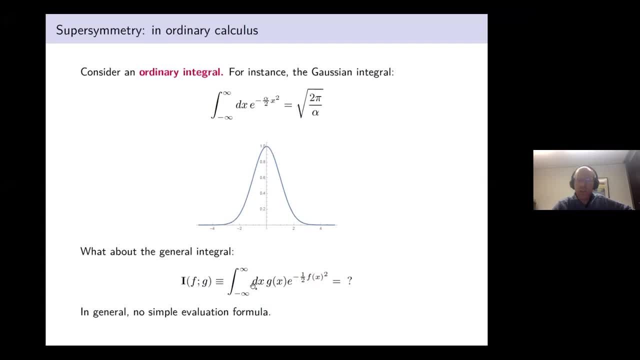 but if i give you a more generic integral, like an integral here at the bottom, vx of g of x, e to the minus r, fx squared. so why do i put i write it like this? is because i could have an arbitrary inter function: g of x multiplied by an exponential of minus f squared. so f squared if x is real. or 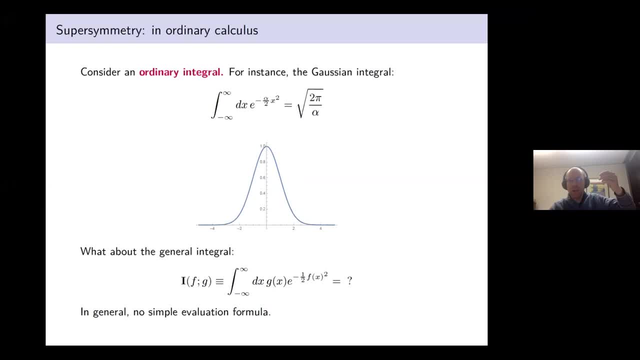 so f of x is a real function. so f, squared is, is a positive definite, and so we have an integral, we have something which pretty much looks like a gaussian that is dumped very much at infinity. so this integral has a good chance if, if g is not, if g of x, the function g of x is not growing too. 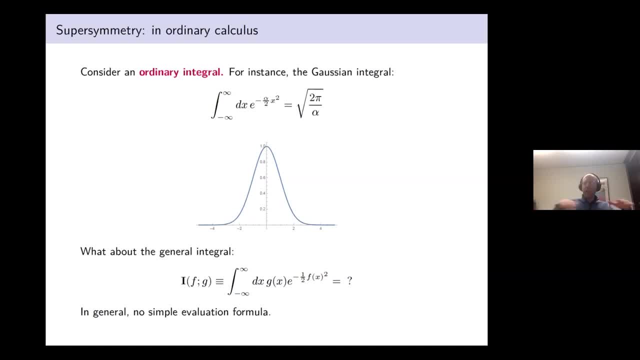 fast at infinity, this function has a good chance of being well defined. integral will have a tiny contribution from infinity, and then you can try to sum all the area under the curve, even though it might be a complicated looking curve, right? so the question here i want to answer is: how can we? 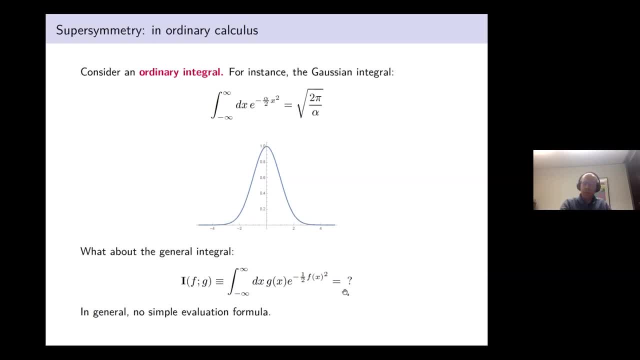 solve this integral in general? well, in general we cannot. i mean it's just a fact of life. you can compute those integral numerically, but there will not be a closed formula to solve for this, like i can say that the gaussian is just a square root of two pi. but there are some nice type of integrals. 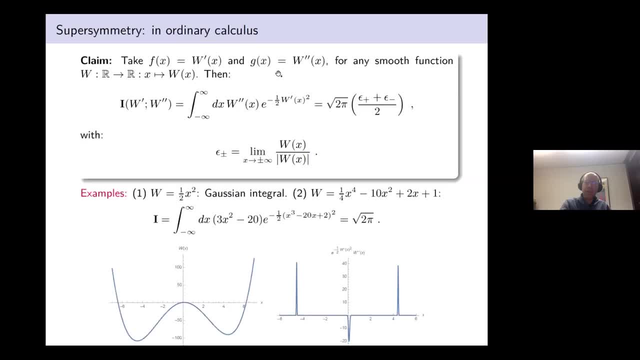 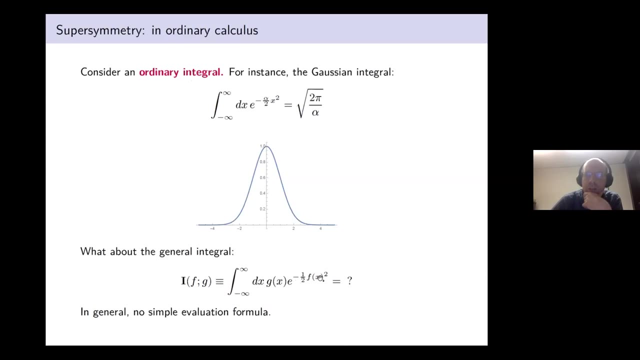 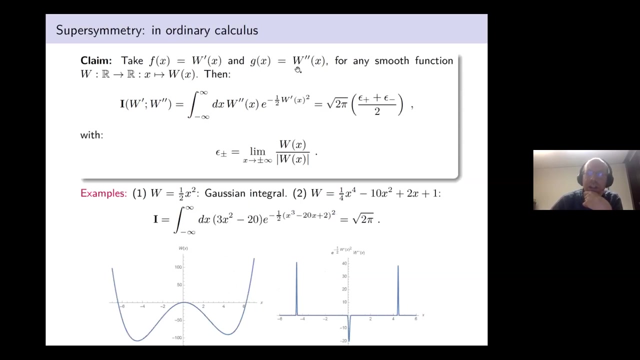 where i can actually solve it exactly and i would like to explain one such integral and give a proof of that using supersymmetry. so here is the integral of the of the form. here, right, i have dx of g of x times exponential of minus one half f, square, f to the squared squared. now what if i take f and g to be related to each? 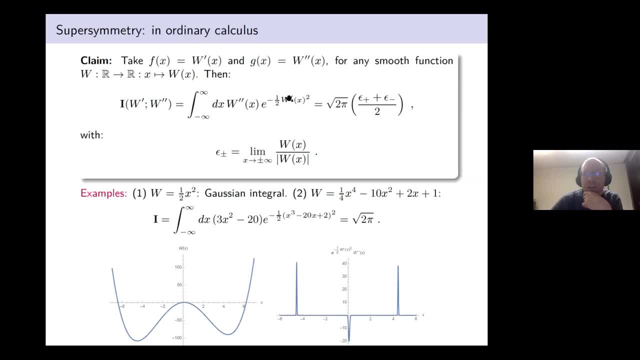 other. i will take the function f in the exponential to be some function w of x, first derivative of it, the first derivative of of w, so w prime x squared in the exponential, and then multiply by the second derivative of the value right. and i want to compute this. so i give one example. 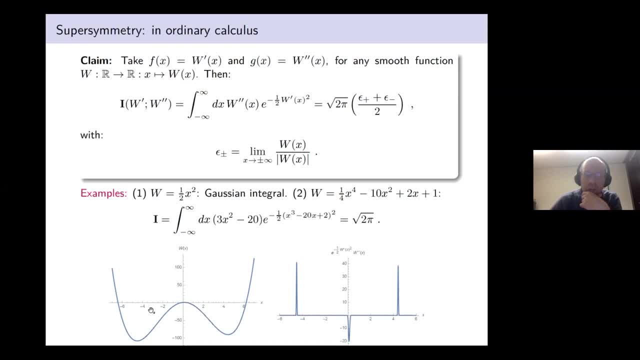 at the bottom on the left is the, the graph of some function w which is here is a particular quartic function, and then if you plug into the integrand here w prime, prime e to the minus one half w prime squared, that's the one on the right. so it looks like, roughly speaking, a bunch. 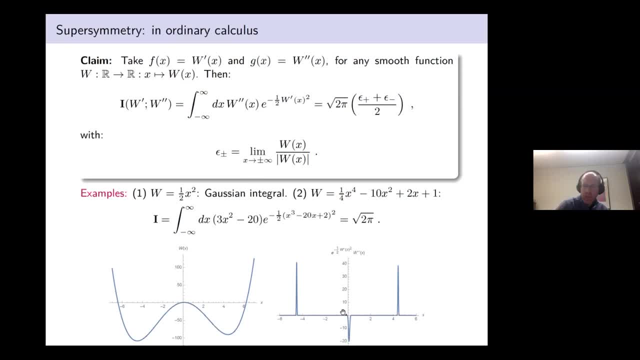 of gaussian, but really it's much more complicated. it's some peaks like that. it's just that it looks like ocean because it's very tightly peaked towards around some points. but you want to compute the area here you see that we seem to have some two positive contribution, one negative contribution, and we know what, what they want to solve, what. 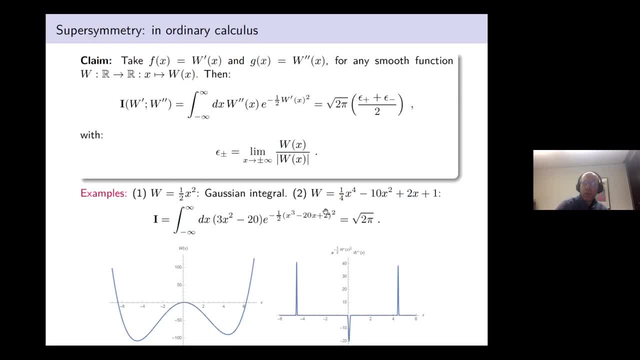 they send to. and good luck to try to do this computation directly. i mean nowadays some computer program can do it for you, probably, but if you do it with pen and paper, i mean, in some cases you can find some clever tricks, but in this case i think it's pretty hard and i can give you even more complicated polynomials and so 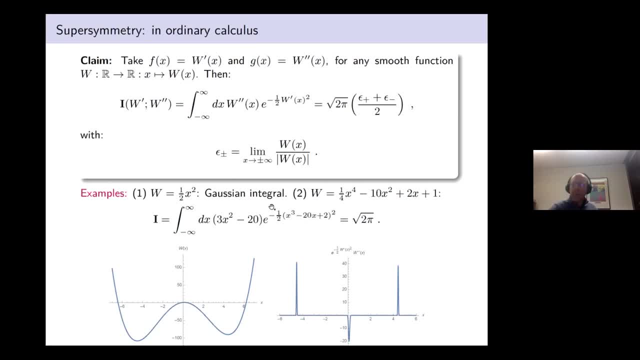 on to or more complicated function, and and my claim is that the result will always be a multiple of square root of 2 pi. in fact, in this case is square root of 2 pi and in general it will be either. plus square root of 2 pi is if, if the the 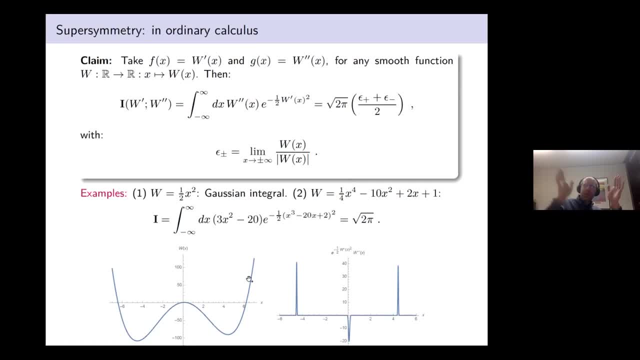 function w on the left here goes to infinity, plus infinity on the left, on the left and on the right. it will be zero. if it becomes a plus or minus infinity on the left and on the right, it will be zero. it goes on plus infinity on one side and minus infinity on the other side, and it will be minus. 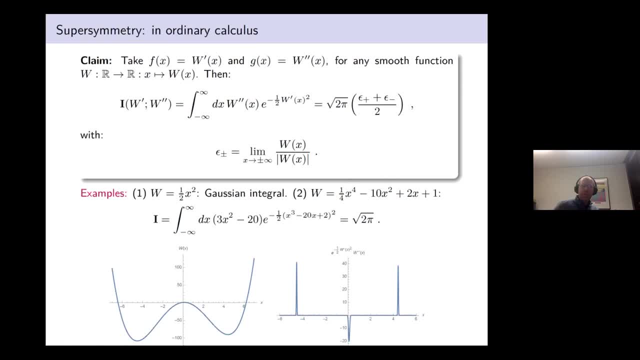 it will be minus one, so minus squared of two pi. if, uh, the function is like, goes to minus infinity on both sides, on the left, on the right, in x. so that is the statement of uh, that's, that's my statement here, the disclaim, and i would like to prove this. 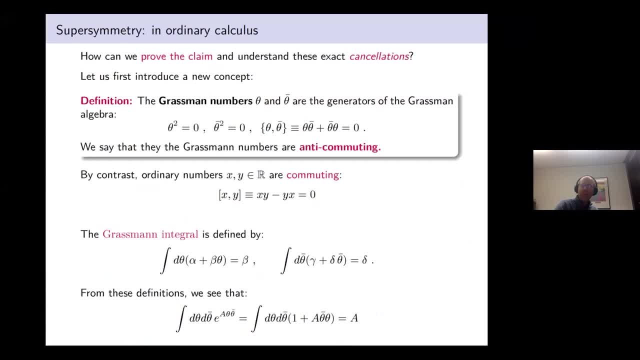 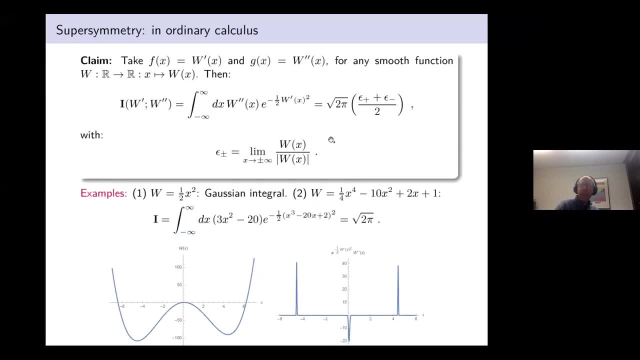 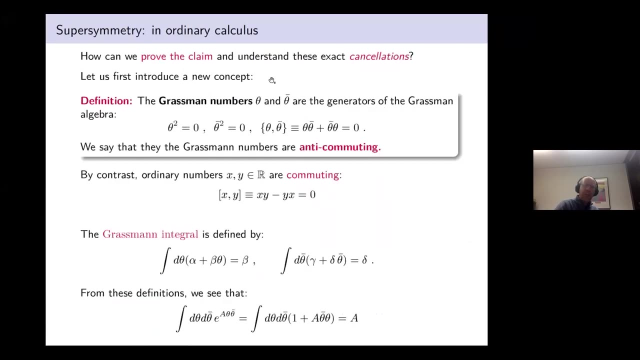 so how can i prove that? well, i will introduce some crazy looking things. that will not be too surprising now that we discussed fermions. so x you can think of like the bosons in this game. they're like bosonic fields, spin zero fields. now what if i introduce a fermion, a fermion in 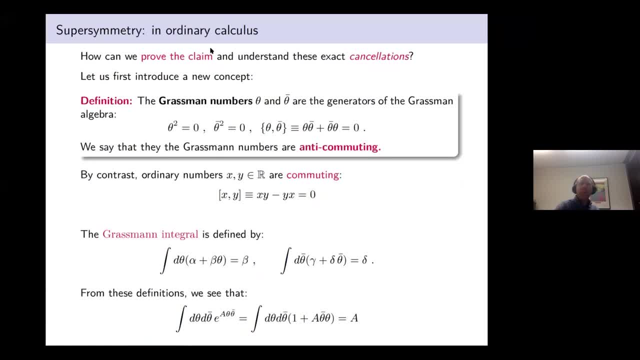 in ordinary calculus will be what we call the grassman number. those are those formal numbers that are denoted by theta, which are generating this, what is called a grassman algebra. so theta is a number that's square to zero. it's non-zero itself. in some sense it's an abstract. 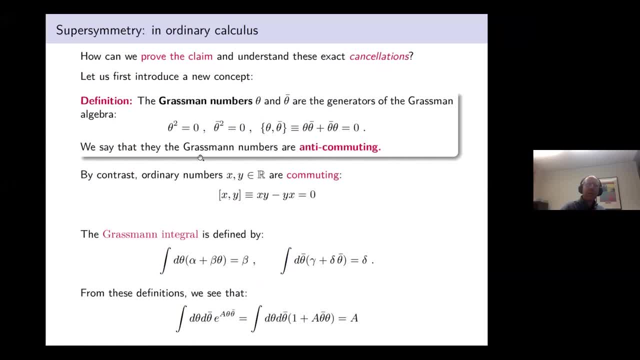 algebraic number, but it's square to zero. and similarly i will introduce another number which i call theta bar, which in some sense you can think of the complex conjugate, but they're independent theta bar squared to zero. on the other hand, if i look at the anti-computator, so t, theta bar plus. 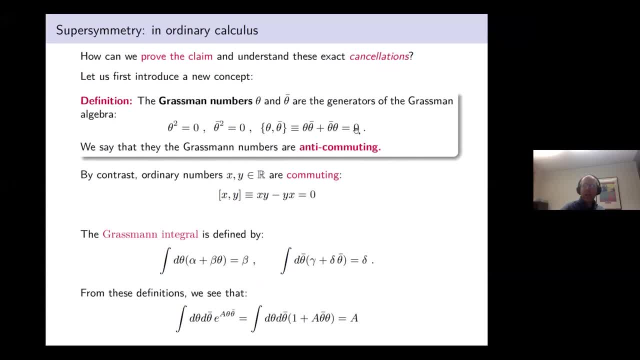 theta bar t, i get zero again. so it means that the anti-commute, so if i take one or the other or the other and the other one, i get a minus zero sine right. so that's by contrast with ordinary numbers which commute right, i can x, x, x, y is. 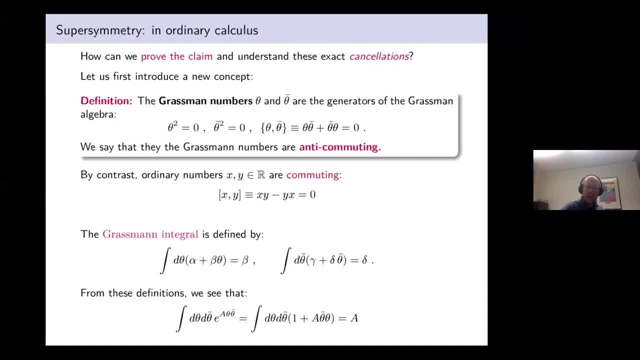 equal to y, x in ordinary commuting numbers, ordinary algebra. so those grassman number look a bit odd but they can be treated in many ways very much like ordinary numbers. they just have this weird rules that they square to zero. then you can also derive and integrate along Grassmann numbers and in particular integrating is defined as: 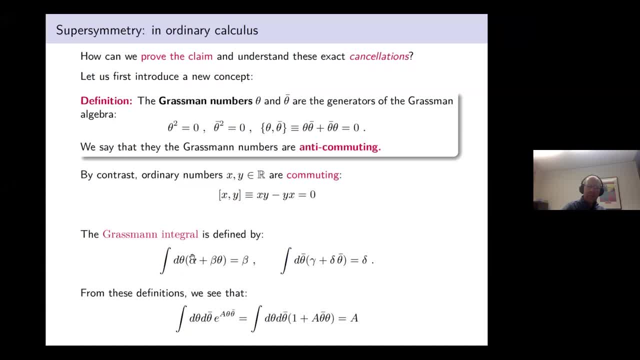 follows in the in the line below. so if I integrate d theta over some alpha plus beta theta, so that's the generic function of theta in fact, because I can always expand any function in in power series and it truncates at theta square because theta square equals zero. so this is a general function of theta and it just 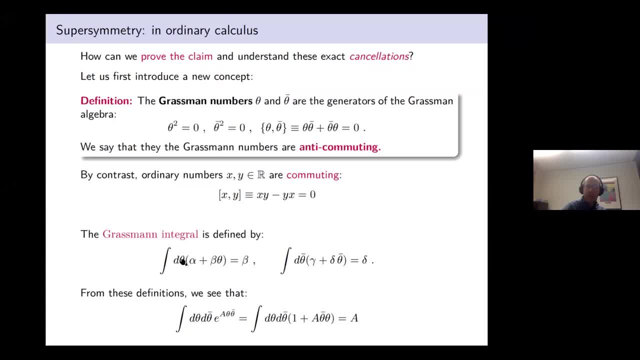 integrates to beta here. so that just means that the integral of d theta, theta is equal to one by definition and everything else is zero. that's my definition of an integral and in fact, yeah, that's the correct definition. and from this definition you can see that if I have this object, the exponentiated theta- 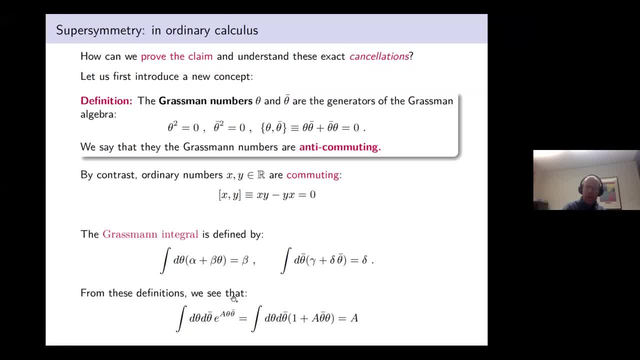 theta, theta bar or theta bar, theta, sorry, I mean exponential of a theta bar, theta, and I integrate this along d theta and d theta bar. I will get a. that's the last time what I did. here I again. I have a function which is an exponential. the exponential is defined by its Fourier series. this is the. 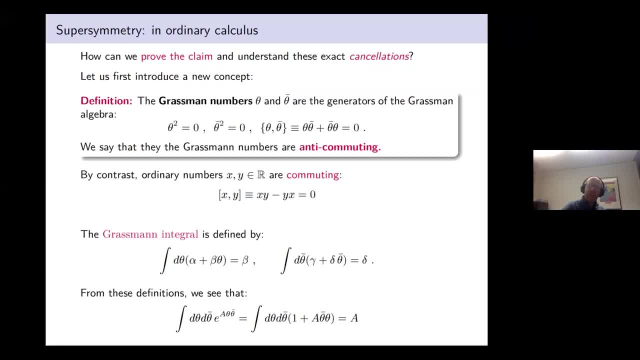 fact that the exponential of X is one plus X plus one half X squared, and so on and so forth, with an infinite series. I can do that with this grassman variables, but it stops at the first term because theta square equals zero. so I just get the second thing, and so I integrate, I get a. so 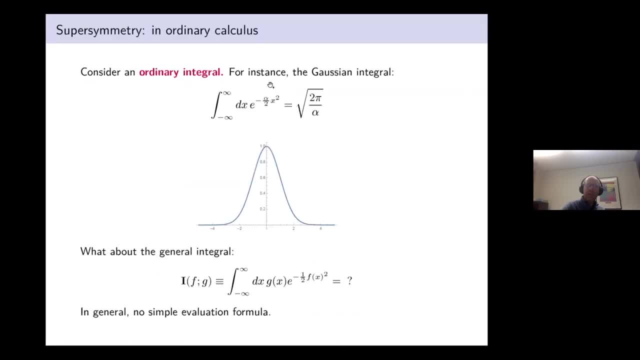 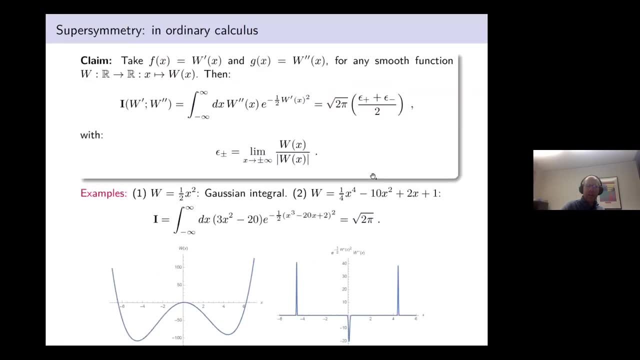 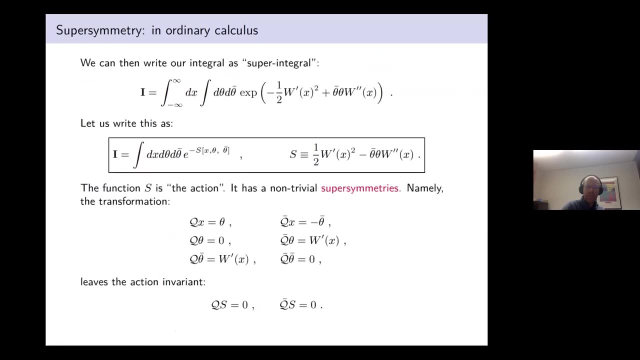 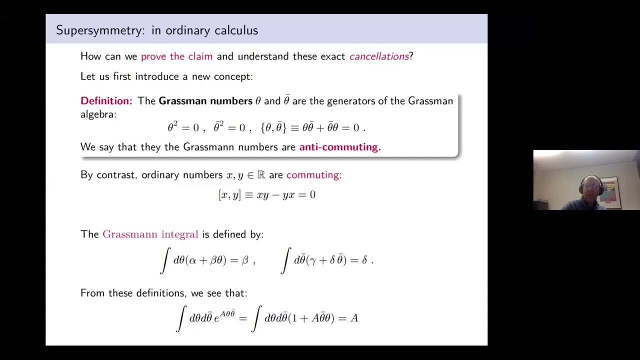 this is the analog of this Gaussian integral for the X variables. the Gaussian integral is is something we can do by standard methods, and the grassman integral for a Gaussian is even simpler. it shows the coefficient here. now, why? why introduce this, this beast, the disturbing number, the grassman number? is because I 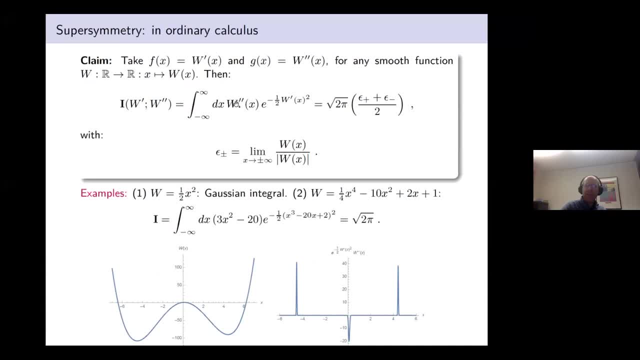 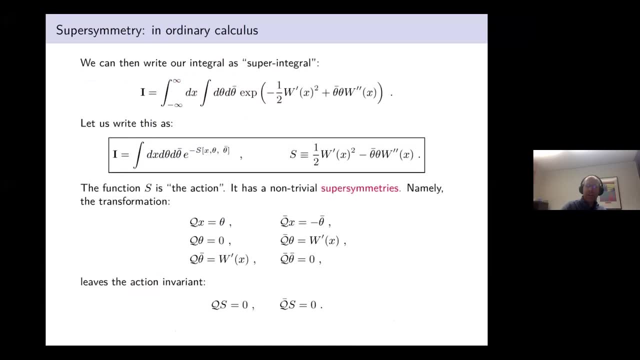 want to write this integral W with the integral being W times the exponential as a single exponential makes it simpler and it's very natural in physics. so I write the same integral as exponential of minus one half W, prime X squared to square, plus theta bar theta W, prime prime, since we. 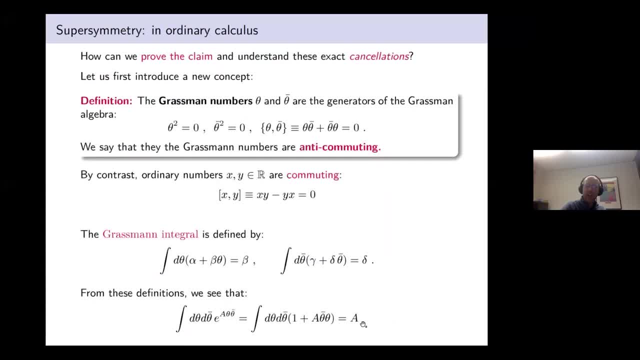 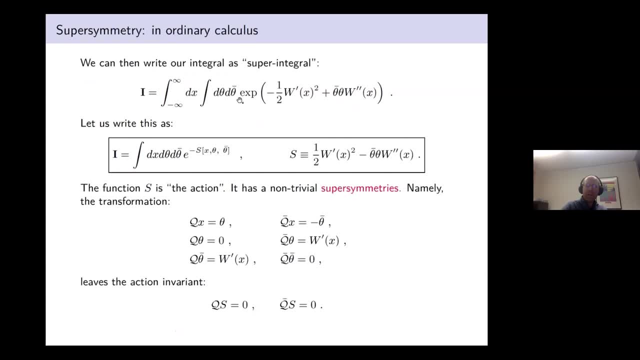 just saw by this last line here that the exponential is the same as just bringing down the coefficient of the theta prime theta term. so this is literally the same but written in a fancy, fancier way. but it's the same as my integral I started with okay. so I just write this same line again in the second line in the box as: 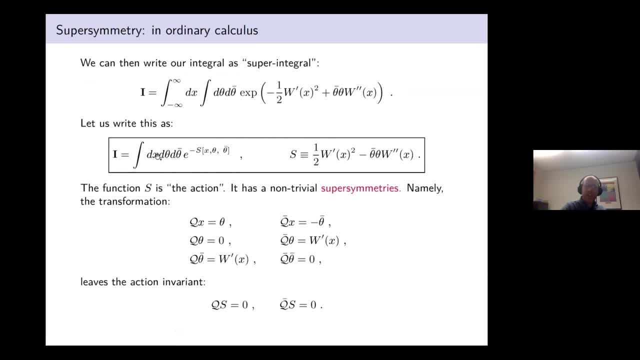 this integral over the X, the Titas and the theta bar, and I forget, the integral is from minus infinity to infinity in X, that's implicit here, of e to the minus S, when S is a function that in physics we will call the action, which is one. 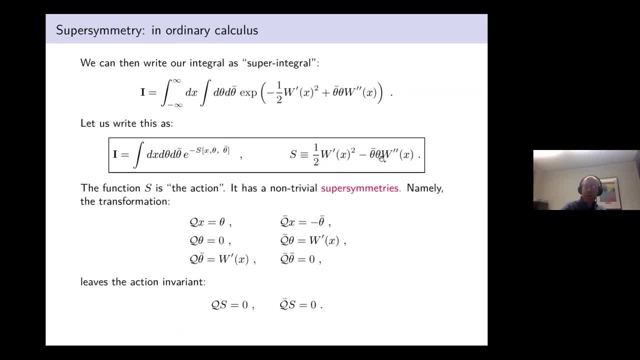 half of W prime square minus theta bar theta W prime prime. okay, so I'm just rewriting the same thing now the. the interesting thing is that this action has as a non-trivial supersymmetry. so again, a supersymmetry is something that actually that maps the boson which is my X. 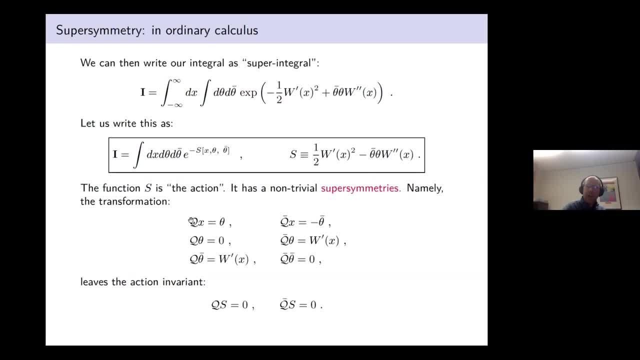 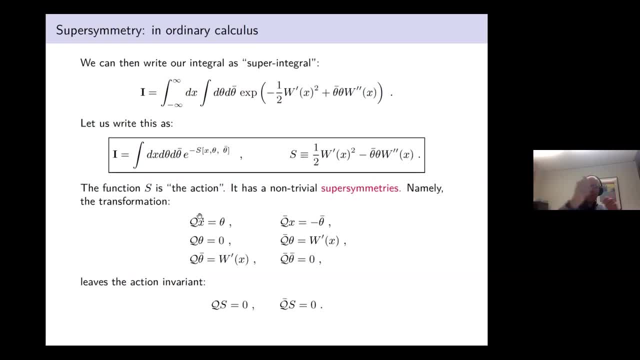 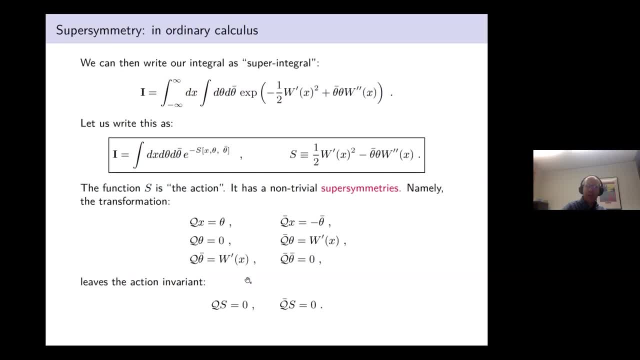 other權ic variables you get W prime of X, okay. so again, boson went to a Therian, a Therian goes to boson, which equals 0 in that case, and off to W prime of X, which is also a boson. it's a bosonic variable. and similarly for theta bar. 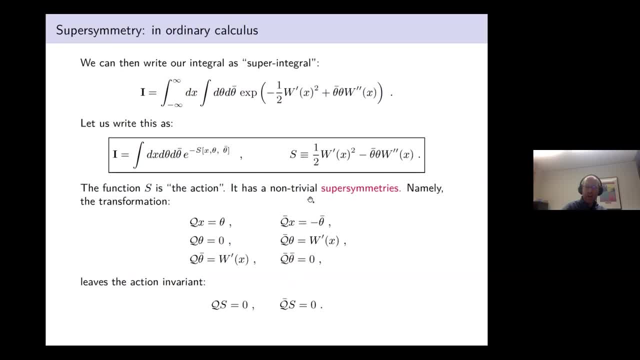 with some minus. there are two different supersymmetries of this action. so this action is supersymmetric in this definition of supersymmetry. it's just a particular action that you need to determine or guess or whatever that brought it. that mixes bosons and fermions, now the, the supercharged Q. so 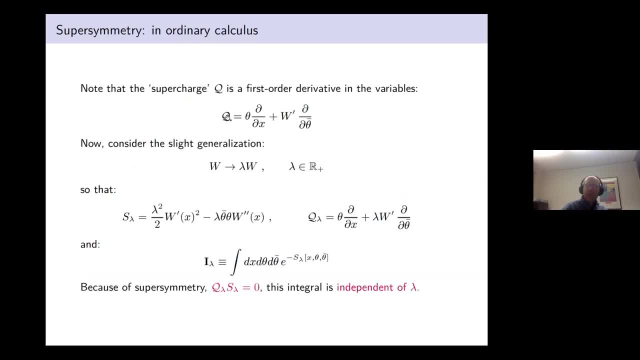 what we, what I mentioned before, the supercharged is conserved quantity or the thing that generates the symmetry. equivalently, the supersymmetry, you can see it as a, as a derivative, the same way that you can see translation as being generated by derivatives on fields, and Q is generated by this particular. 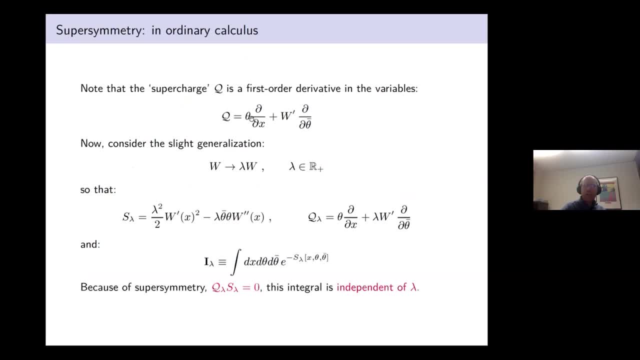 first-order derivative. it's a bosonic, it's a terminic operator. so it's theta, which is terminic, times the derivative along X, the bosonic direction, plus W, prime of X times the derivative along theta bar. and taking the derivative along theta bar, it just means collecting all the terms. 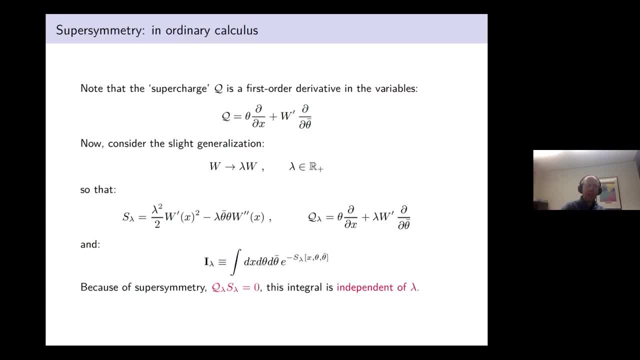 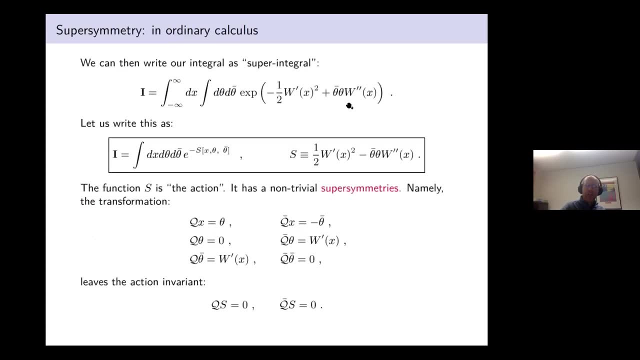 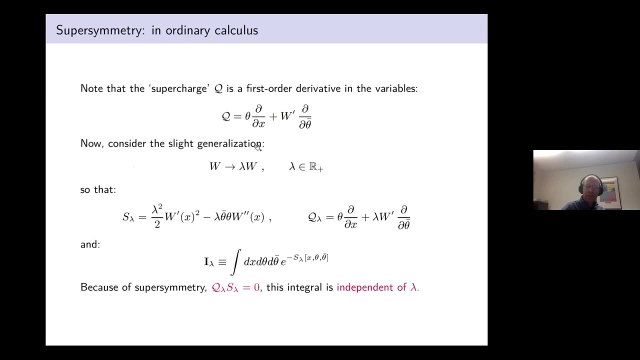 with one theta bar and taking the coefficient like the integral. okay, so I just wrote this fancy integral in a supersymmetric way. but what does it bind me? well, let me first consider a side generalization of the same integral. I will just multiply W by any coefficient lambda, it's a real positive coefficient. 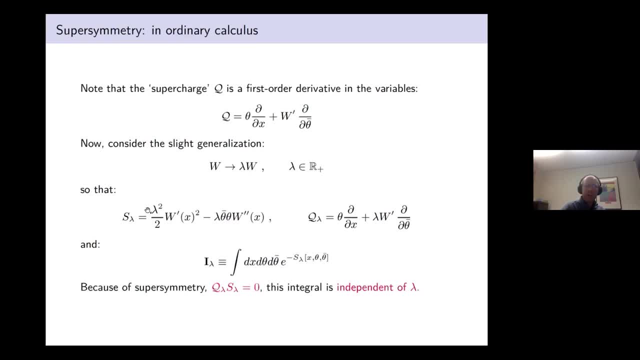 could be equal to one. you get back the original thing, so it could be equal to 100 or 1 million. so you just rescale W by lambda, then S- the action is that we know called S of lambda- is rescaled like this right, because W? 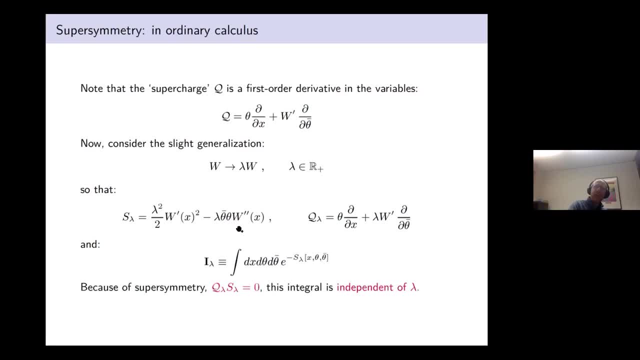 prime square. so it tells lambda squared in the first term for lambda in the second term and the supercharge itself is depends on lambda in front of W. but that I didn't change anything, it's just a change of notation. if you want, I just pull out this coefficient lambda, and my action is still supersymmetric. Q, Q, lambda. 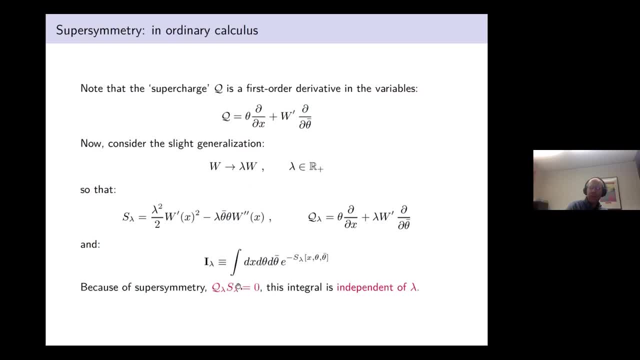 acting on the action. Sigma S lambda is equal zero. now the claim is that this symmetric integral is actually independent of this coefficient lambda. the overall coefficient on W, the proof is one line and is the most important proof in in supersymmetry. the proof is four lines are here. it goes as follows: 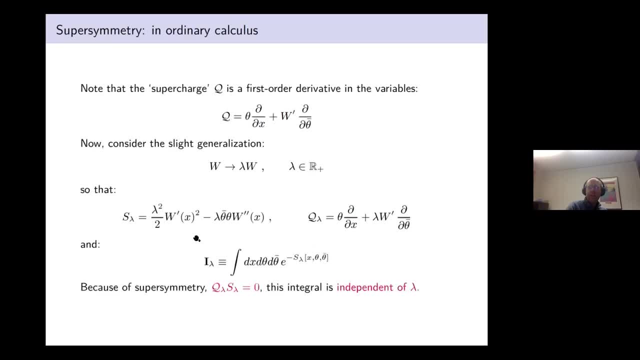 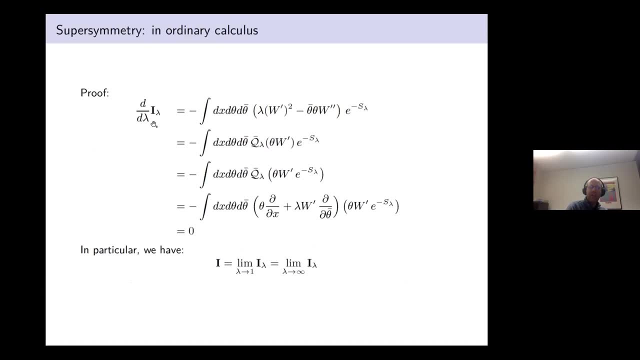 so let's see what does it mean? that it's independent? it means that the derivative of I of lambda with respect to lambda is actually zero. so let's do that. take the derivative of W of I of lambda. with lambda you can easily. it's E of S of lambda. S of lambda is given here on the, on the last, on the. 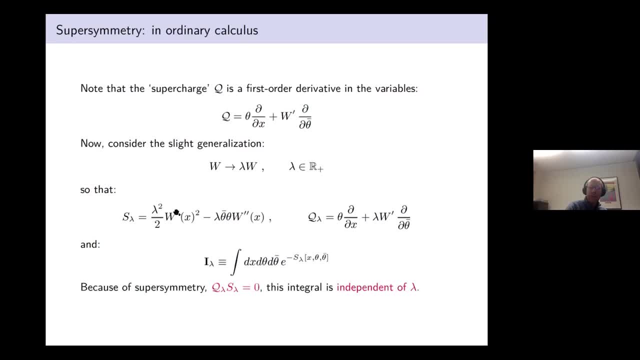 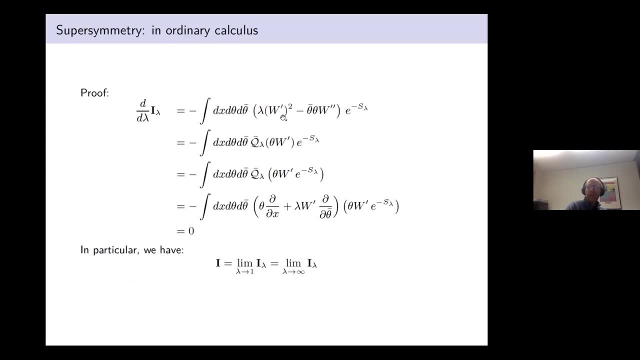 on the third line. so well, you can do the derivative of E of a function. so it brings on the function. take its derivative. so that's the first line. now these first lines can be written as Q bar. it might be Q anyway, I think it's Q, Q of lambda on on theta W prime, so you can check that. 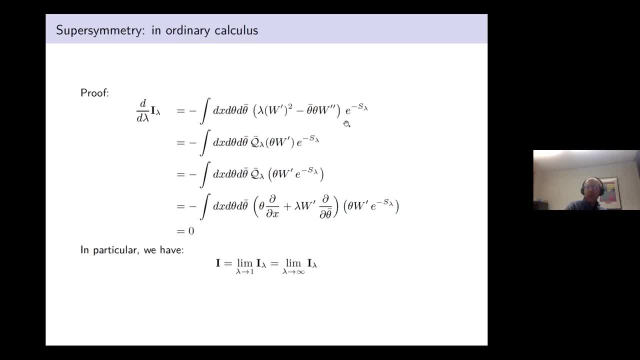 this, all this, all in the thing in parenthesis in the first line is actually Q, the supercharge acting on theta times W prime. but we also saw that Q leaves the action invariant. so I can just in the third line, put everything around the same parenthesis meaning that the action invariant is the action invariant. so I can just in the third line, put everything around the same parenthesis meaning. 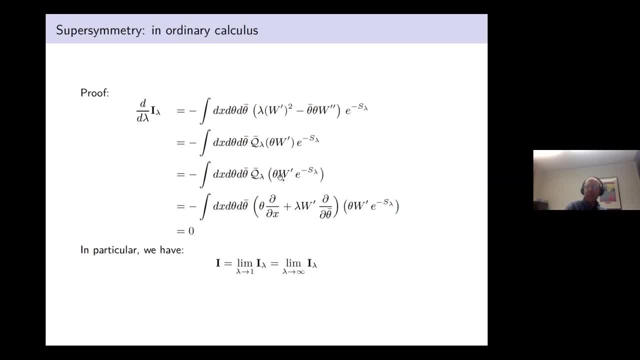 like the supercharge acting on all of this is zero. sorry, it's not zero In that on the first term it gives the first line, it acts on this. on the second term, by the general it just gave the same because the action is invariant. so I mean Q of S is zero, so E to the minus s. 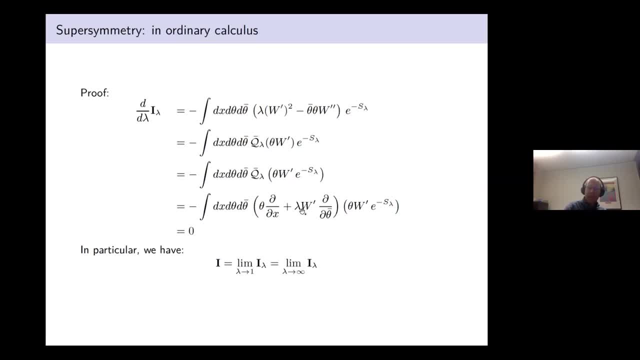 is stays the same product, it factors up. ok. so last line, I just write out explicitly the supercharge Q of lambda. sorry, there's this typo. it's it's q, not q bar, and it's just this operator, as we said, is this differential operator. so the first term, um, it's an. it's like an integration by power that you. 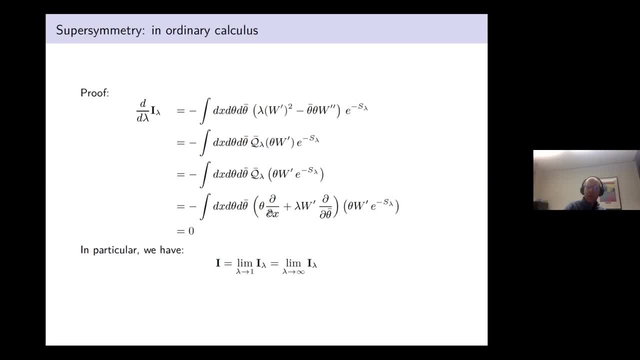 probably have done many times in integrals. so it just tells you that. uh, you know it's a dx of a total derivative of something. so that's the fundamental theorem of calculus, right? so it just gives you the, the results of uh, of whatever is on the right, uh at minus infinity, plus infinity. 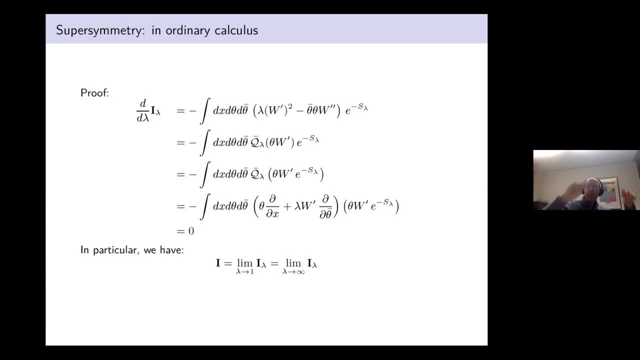 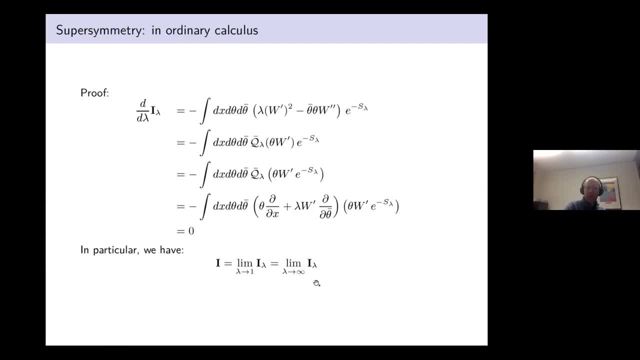 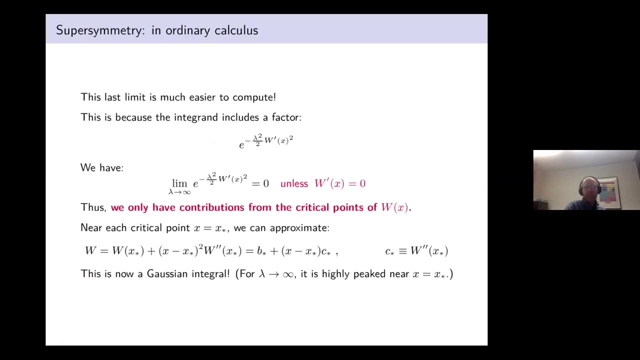 actually, um is zero as well by the definition of the grassman integral. so we just prove that this supersymmetry, uh, this, this supersymmetric action, does not depend on the coefficient lambda in front of of w, this function, w. okay, so finally, um, i can take a, then a limit to compute it more. 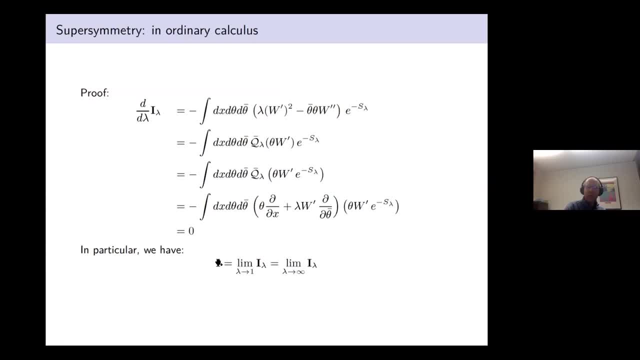 easily, since i just told you it's in terms of lambda. so what we will have to compute is when lambda equal one. but then i can just take a limit when lambda goes to infinity, and you have to be careful that nothing drastic happens when you take this limit. 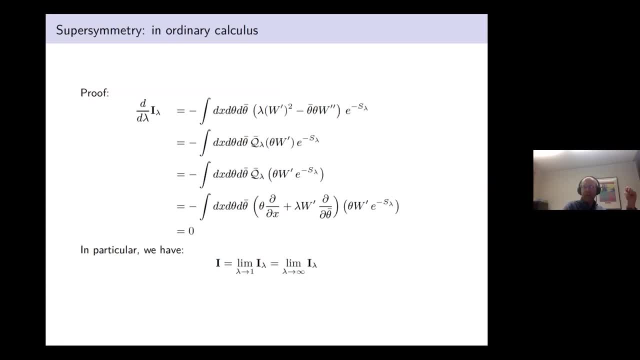 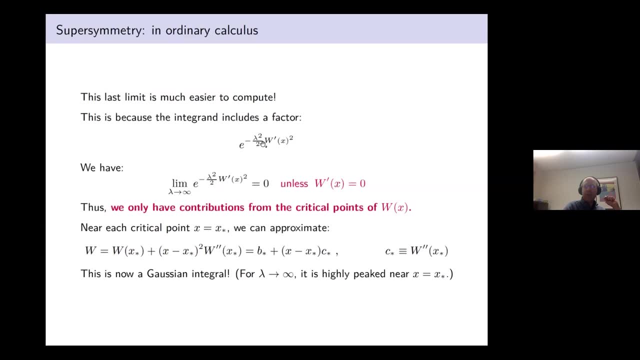 but under the mile assumption, nothing will happen if you just continuously move it all the way to infinity. but if i so that, that means i will weight my integrand by this factor e to the minus lambda squared, when lambda square is very, very large. so what happens in this limit? well, i can take try to. 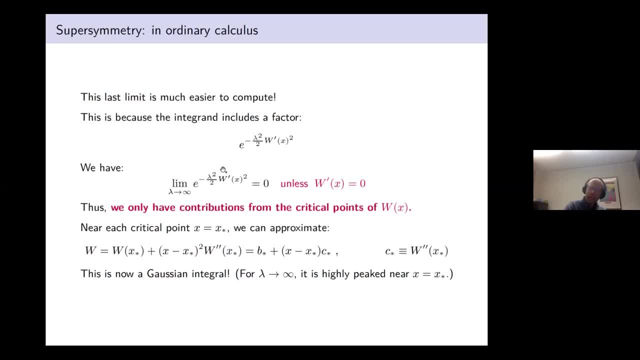 take the limit of this function: e to the minus square of w prime of x squared, and obviously if w prime itself is non-vanishing, this vanishes because everything is positive definite. so it's: e to the minus lambda squared, it goes to zero when lambda squared goes to infinity. 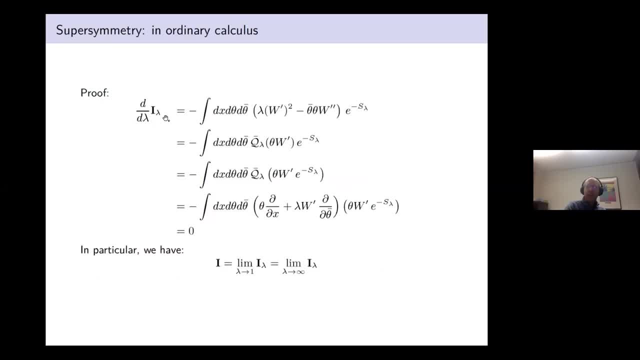 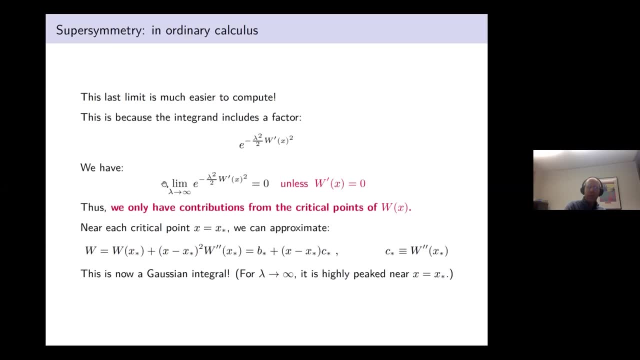 so this seems to naively, of course, tells you everything: vanish i equal zero. that's not true, because, of course, what happens is that we still have contribution at the point where this limit is more subtle, because w prime vanishes and, by definition, w prime equals zero. 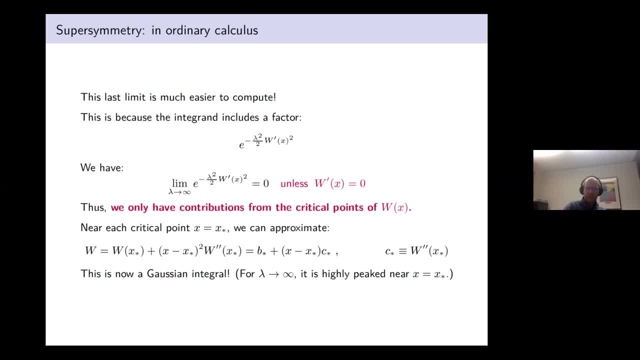 are the critical point of the function w. now, near each critical point i can now approximate by a Gaussian integral, because w can be expanded around the critical point by definition, the value of w at this critical point, the first and the first relative, vanish at this point by definition of a critical point and then 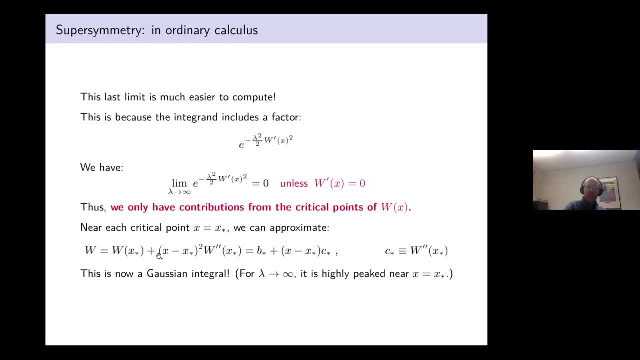 the second order term there should be one half- sorry, one half- of x minus x, x star, where x star is a critical point squared, and the second derivative at this value, right. so it's just a tail of serial expansion to second order, and i can always do this approximation of an integral. it's called the, the. it's called the. 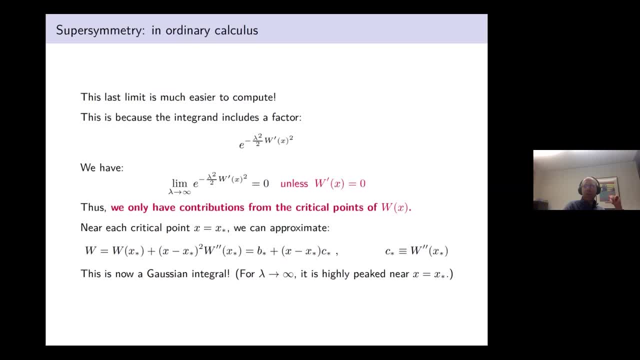 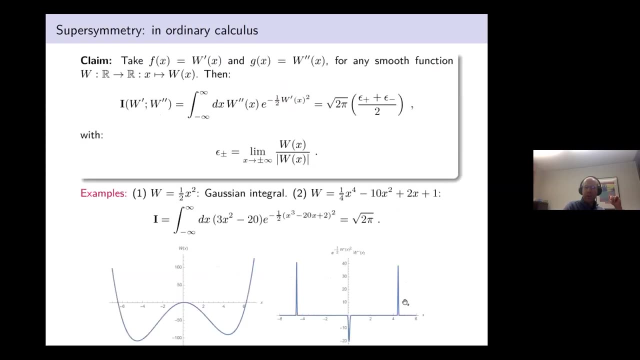 steepest descent method or some, some name like that. but the point is that here, when lambda becomes very large, this approximation becomes exact each time the integral becomes highly, peaks around various points the critical point, which are essentially those three points here on the right right which are the critical point in this example, right on. 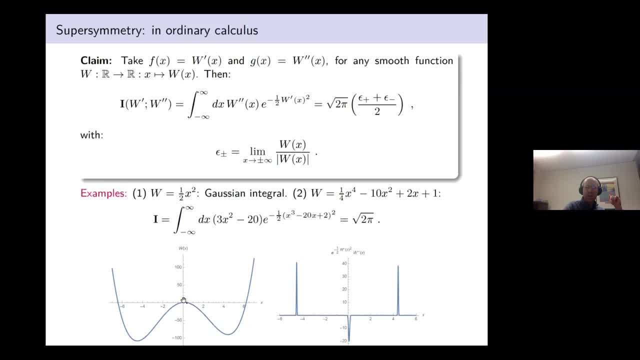 the left, i have three critical points. each time when the, the function w turns, and these are where we have three peaks and we see that the, the, the integrals, uh, in this example is already very localized near this point, but if i took lambda to infinity, in fact it becomes infinitely. 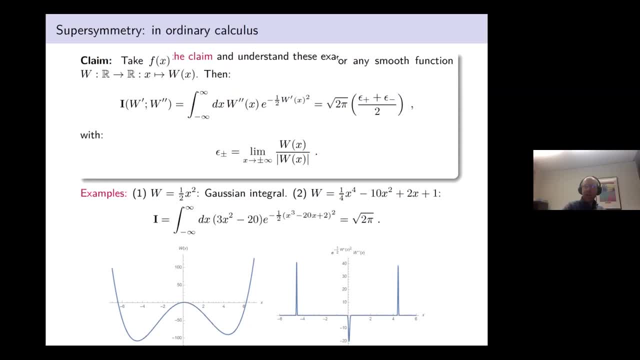 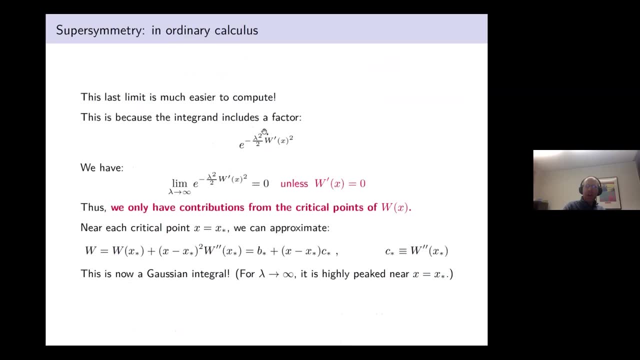 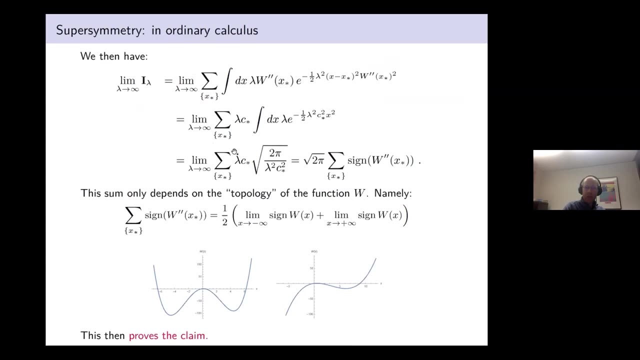 big around this point and zero everywhere else, and then it becomes very easy to compute it. so then, uh, yeah, a little a few more, uh, a couple of more line of algebra shows you that, uh, so you just need to plug in- i won't go through it line by line, but in this limit- then you just get a sum of 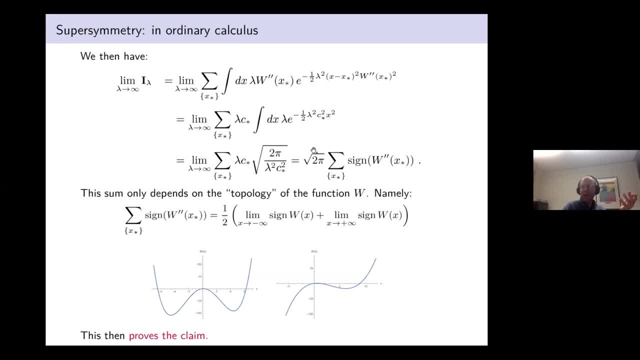 quotient integral, and we know how to do quotient. i just call it off to pi for the quotient integral with a coefficient which will not be if you follow the algebra through. it will just be uh, the sign of the second derivative of the value. in other words, you get uh, you get zero if it's uh. so you get uh. yeah, i mean. 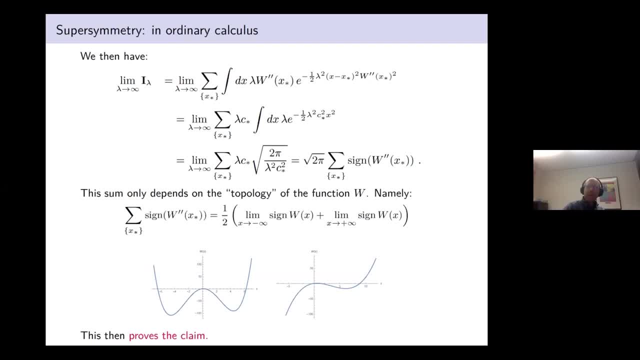 for a generic w, you would just get um, you just get plus if it's- uh, concave and minus if it's convex or vice versa. and the sum, then, of the critical point only depends on the total topology of the function, which is what's my claim at the beginning. so again in my example, uh, the first for 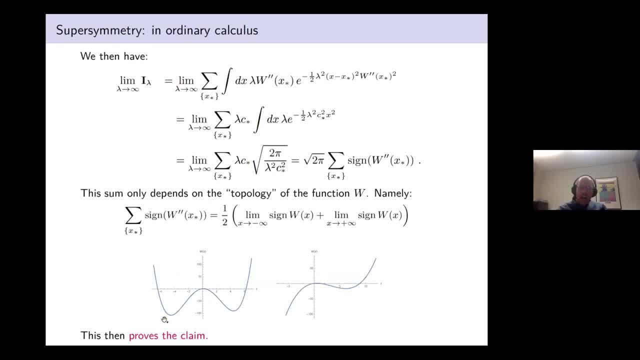 the third w the, then this complicated integral, i will just be: uh equal to plus one times square root of two pi. just because i get uh plus one from the first guy point and minus one, that's plus one. so that gets plus one in total and in general you can easily convince yourself that if it only 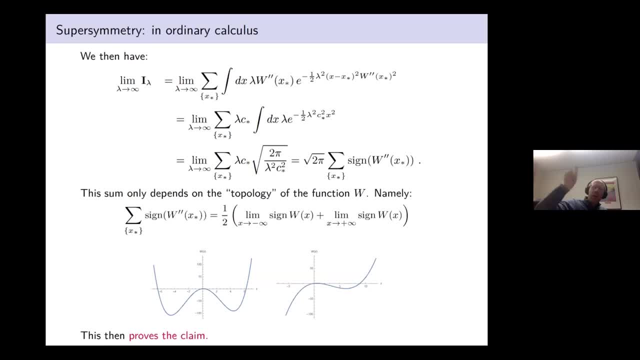 depends on. it doesn't matter how many uh ups and downs there is in a generic, polynomial or marginal function. um, it only matters how it goes to infinity, if it goes to plus infinity or minus infinity, and so that proves the claim. so that was an application of supersymmetry to a. 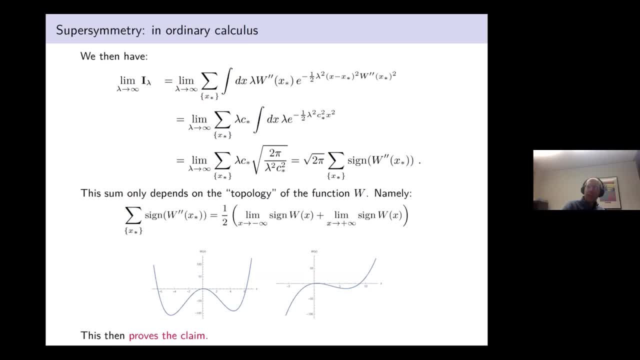 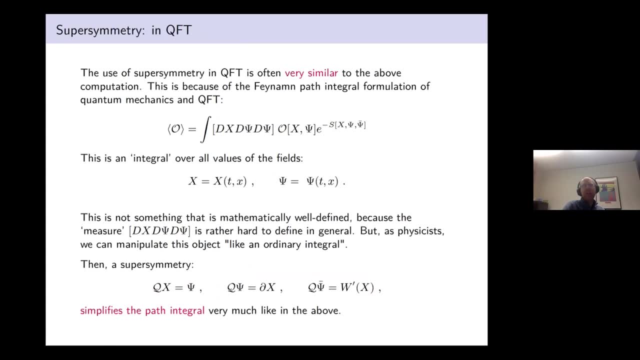 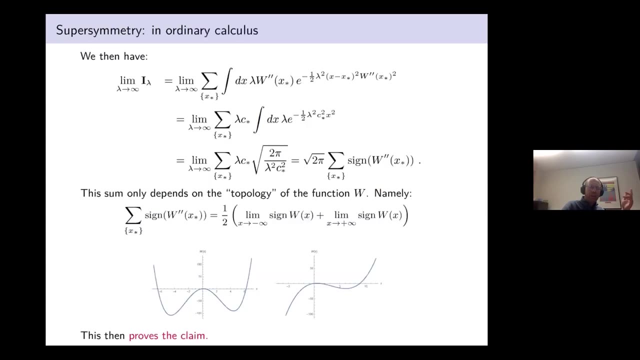 easy sounding or problem, maybe slight. i mean, you might be slightly bored at this point, but i think it's a fascinating, uh, application of symmetry. um now, why i go for this is because, actually, this i think: if you, if you wrote it down, if you go to the algebra, you can do it no problem, understand every step. 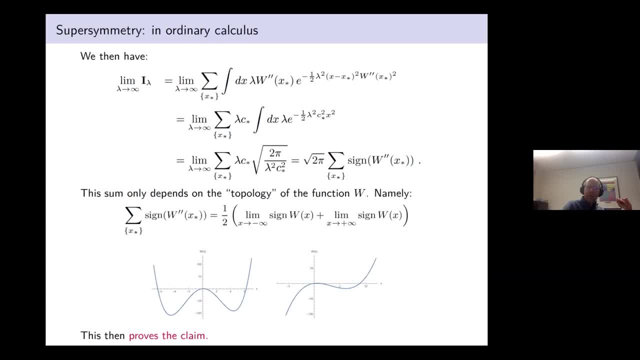 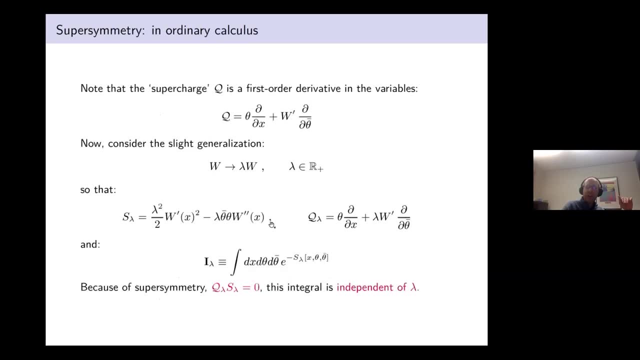 uh, even with first-year calculus. but this very same kind of principle and this simplification that has to do with the fact that my action, what i call the action, this ordinary integral, was super symmetric. uh all also in quantum field theory, where there are a much more complicated 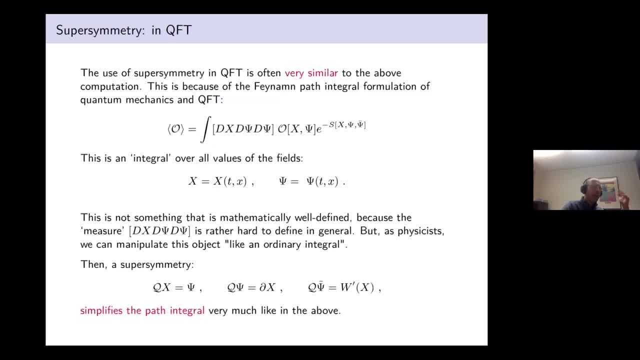 system. but the key relation is that there is a formulation of quantum mechanics and, more generally, quantum field theory, which was introduced by feynman, where every observance, everything you want to know about the system and every quantum of servers is written as an integral, except that it's not an ordinary integral with, like a finite number. 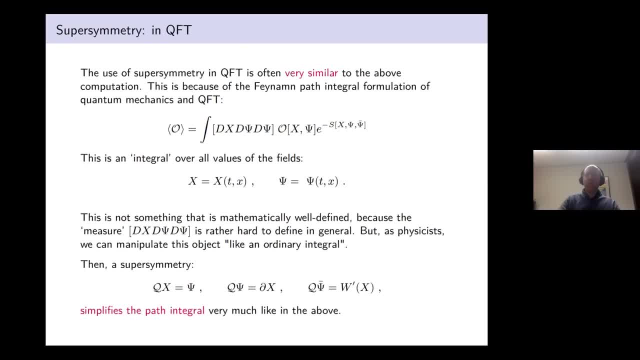 of variables. it's like, morally speaking, an infinite number of variables and such an infinity of variables and a continuous infinity that mathematician cannot make any head or tail of it. so it makes no sense mathematically, except in some simple case, in fact, in quantum mechanics. 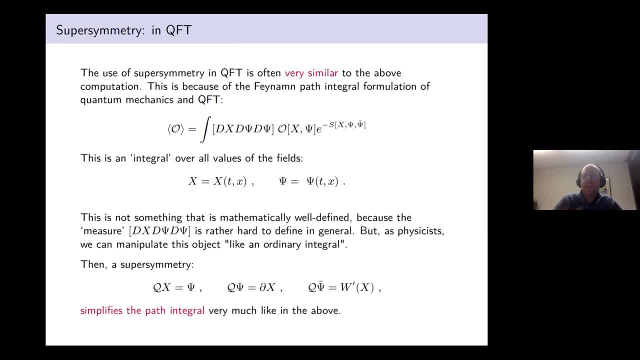 it does make sense, but not in quantum field theory. so i'm going to work with this kind of integral very formally and compute a lot of beautiful results. uh, so this integral is called the passing integral, as i said, and now it will be very similar to what we said before. it's just that my x now are the actual bosons of a quantum field. 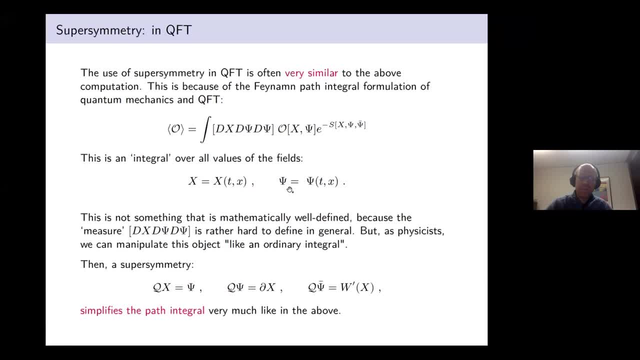 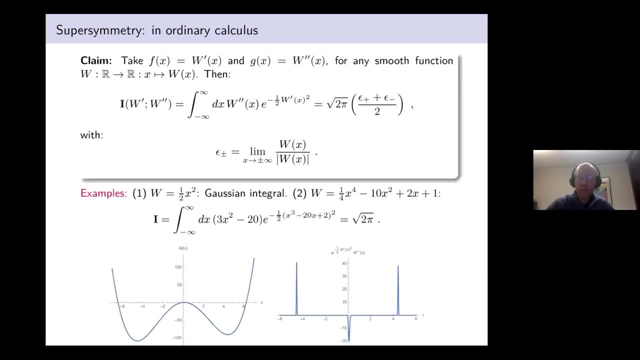 system and the psi are the other fermions in a supersymmetric theory. and the funny thing is that in the generic theory, without supersymmetry, this action is very hard. similarly to if i take an ordinary, an explicit integral and give me, ask me for a primitive: uh, there is no plus form formula. 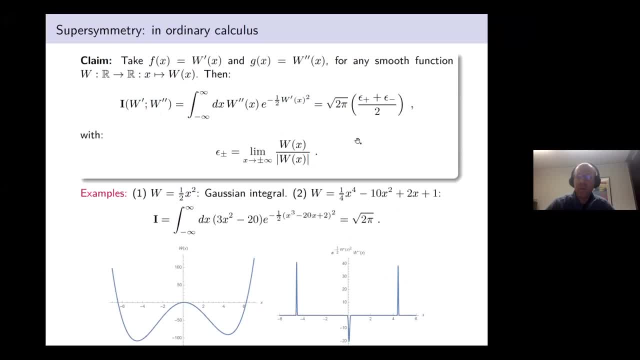 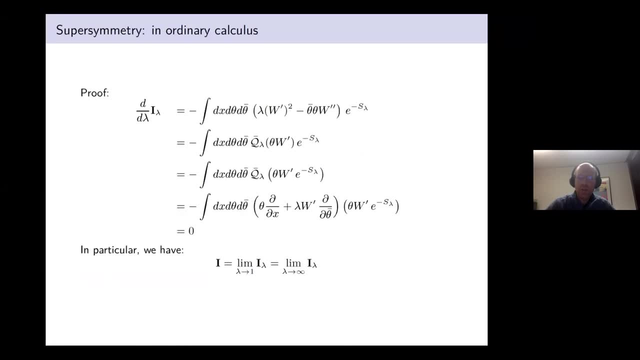 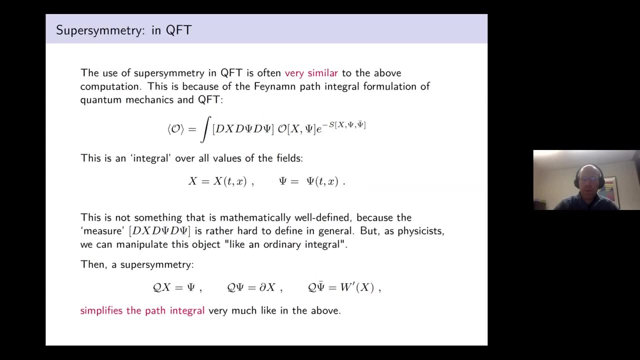 but in the case when the this pass integral is supersymmetric, we might be able to solve it like we we solve this, and it's a. it's a very active area of research, even even even today, to do that in quantum field theory, and one finds a lot of beautiful results anyway. so maybe to uh to conclude, 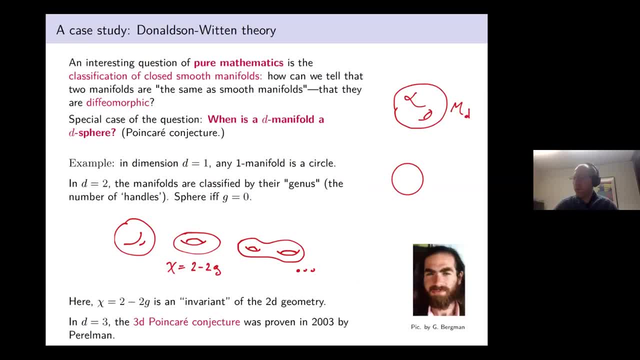 if i can have uh five more minutes. uh, i would like to uh to explore, um, i mean give an application of these ideas in uh, where there was a beautiful interplay between uh physics and pure mathematics and where these ideas of simplification of quantum field theory from supersymmetry was very powerful and this question. 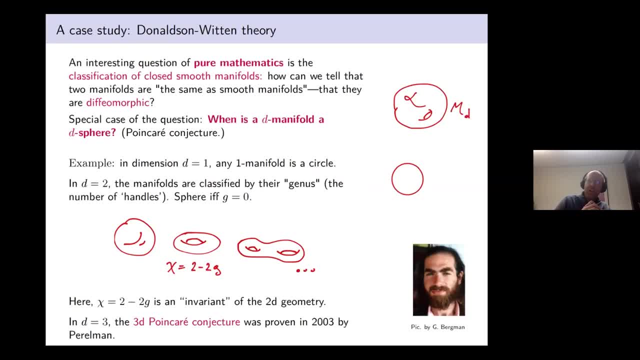 you can ask the question first, just as a mathematician, which is the question of classifying a smooth manifold. okay, so that's the the question of you know a smooth manifold, right? so if you are thinking about, uh, like a sphere, you know, because there might be a lot of to unpack here, but we can, we can get away with. 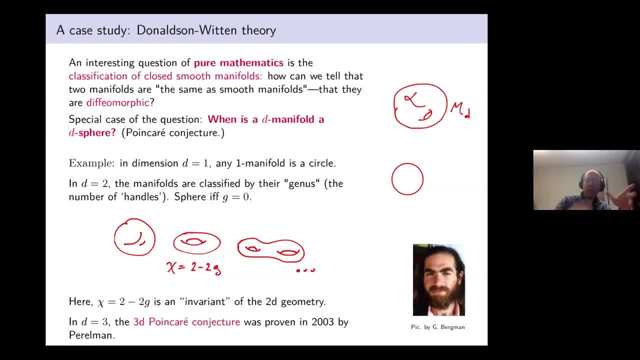 with just thinking of a few examples. so if you manifold is essentially a smooth space like a sphere or a donut or terrace and so on, and that's in two dimension. you would have the sphere and the towers, like in in the picture in the middle. in one dimension there is just a circle. um, if it's a close. 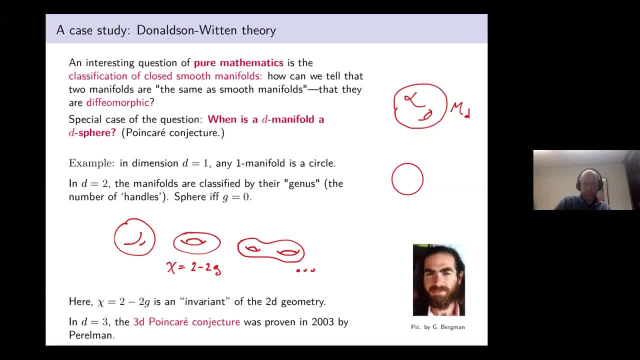 for the and so on, and the question is given to such space: to smooth, manifold. when are there diffeomorphic meaning? I can continuously deform them in a smooth fashion. so, for instance, it's well known that if I take- I mean my, my curve, for instance- in my example- any animal, I can continue deform it to a. 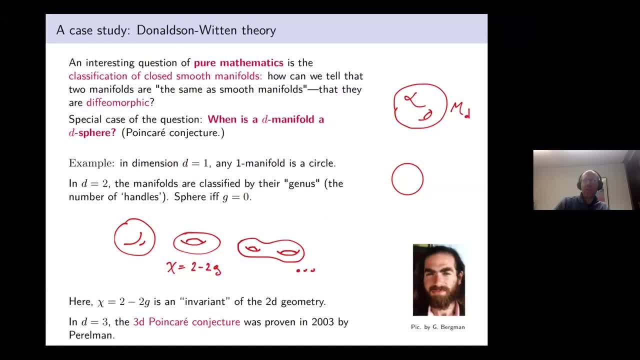 sphere. there is a continuous operation that does that, and so you might be given two very different looking manifold in in some sense, but they may still be the same in this guys, and the question is: when one are they the same? that's the question of classification manifold in mathematics. a particular case of this is 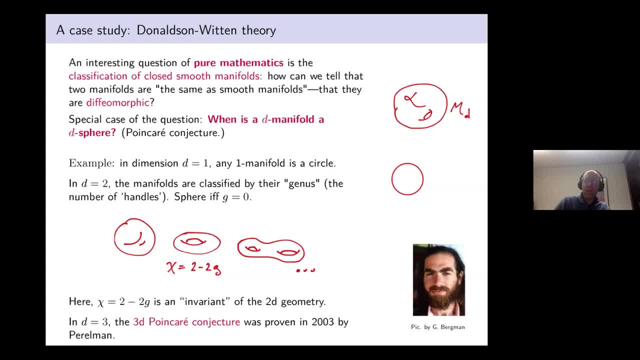 one is a d-dimensional manifold sphere. so that's the the Poincaré conjecture. in the case of in 2d, in 3d, in 4d, Poincaré gave some conjecture about when is a manifold sphere a century ago. 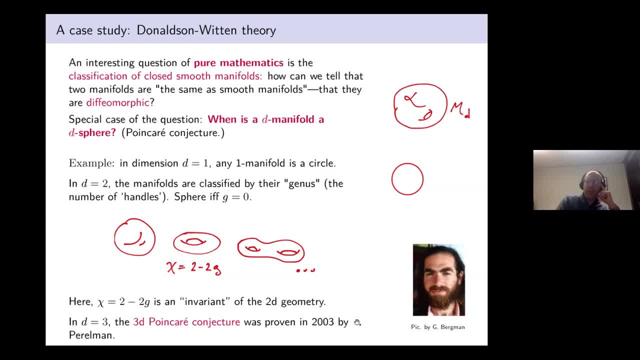 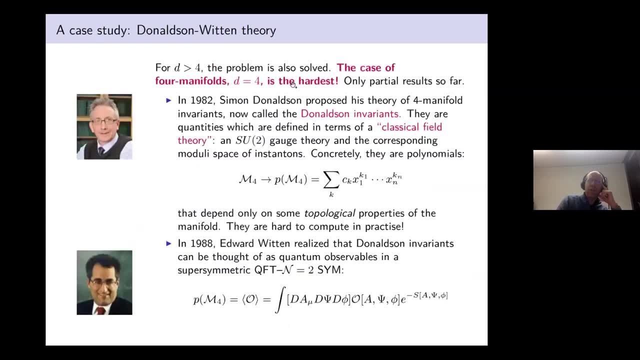 And in 3d. this Poincaré conjecture was proven recently by Perelman. In higher dimension, In dimension larger than four, this problem is also solved, Interestingly enough, when you go to five, six and any dimension becomes somewhat simpler. I'm not an expert, but I hear from mathematicians that this is well understood. 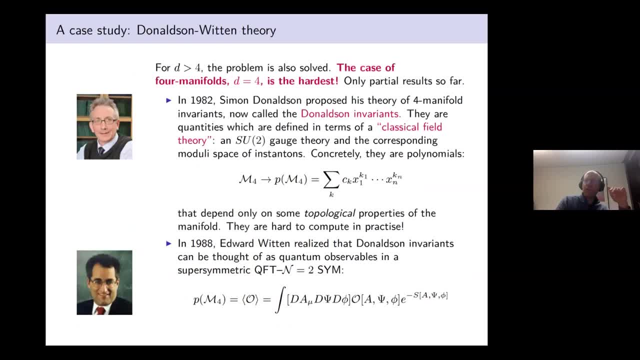 but uh, interestingly, D equals four, which is all the dimension of space time. but here we're talking about spaces, not space times, But we're talking about four space, dimension of space, which is curved into itself, So it's close. So when d equals four, uh, this is a four manifold, and this is the hardest problem for mathematicians as well. 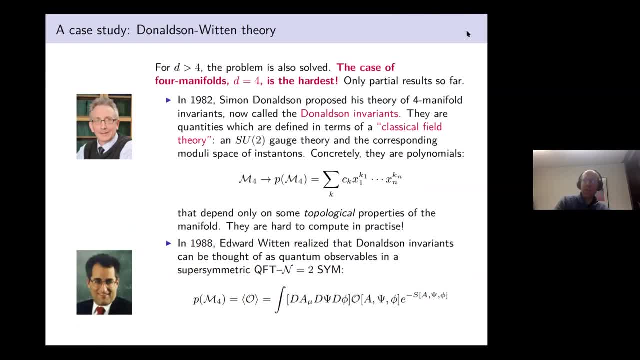 Uh, there is no solution to this problem of classifying manifolds, But there's been some interesting progress made both by faces and mathematicians, but first by mathematicians dalsons. simon donaldson In 1982 came with this theory of dalson invariant, which assigned some formal polynomials. 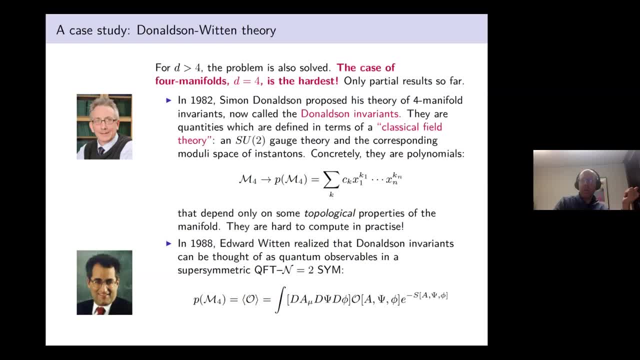 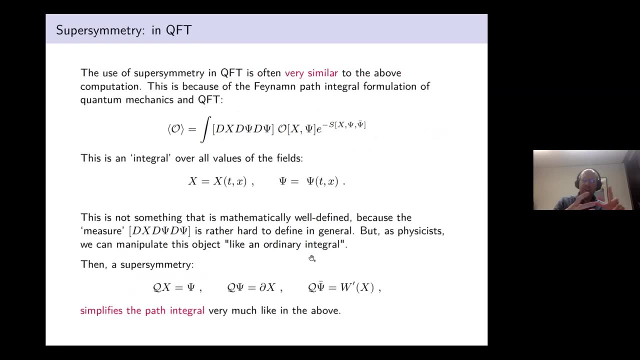 to a given manifold and those polynomials are. The definition is rather complicated but they depend only on some topological properties of the manifold. topology means like the number of points and the number of handle in my 2d example. that's This kind of topological properties, so basic properties that do not change when you start. 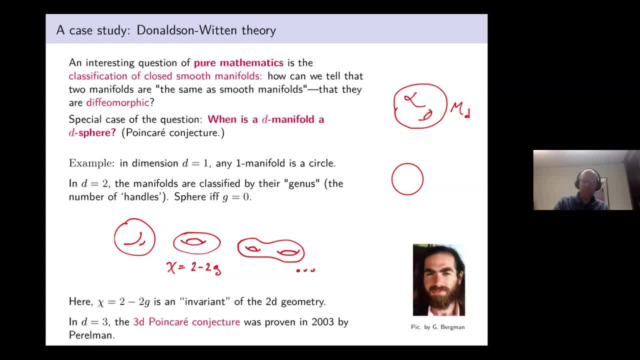 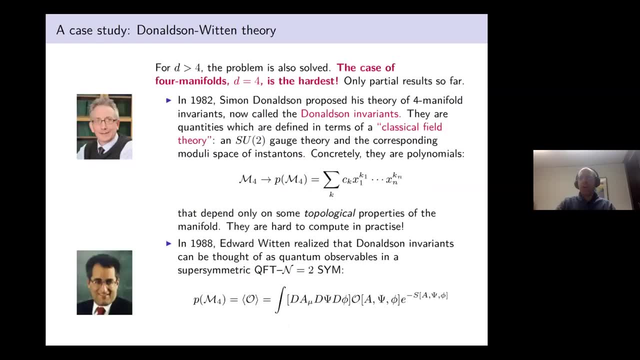 deforming the manifold and squashing It and whatnot. So he defined those polynomials that they can compute in principle, and then they would distinguish different manifolds among themselves. The problem is that those manifold that rely on what is known as a classical field theory 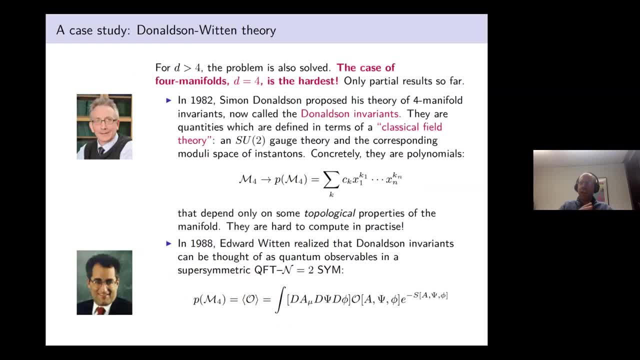 Or a gauge theory more precisely, are very hard to compute explicitly Now. in 1988, edward witton uh, the famous string string theorist and quantum field theorist, realized that those dalsons invariants that were introduced in mathematics Can be taught in physics as a path integral, So quantum observables in a supersymmetric quantum field theory. 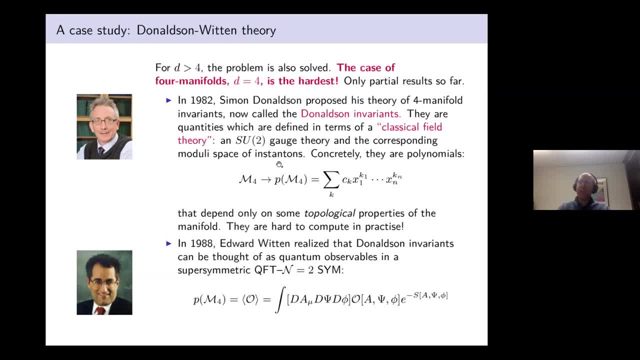 So this thing that uh dalson thought was a classical theory is really Quantum and it's actually supersymmetric. That's what's what? So This complicated, Complicated but well-defined mathematics into This is fast integral at the bottom. So at the time that seems like a very interesting point, but it didn't give. 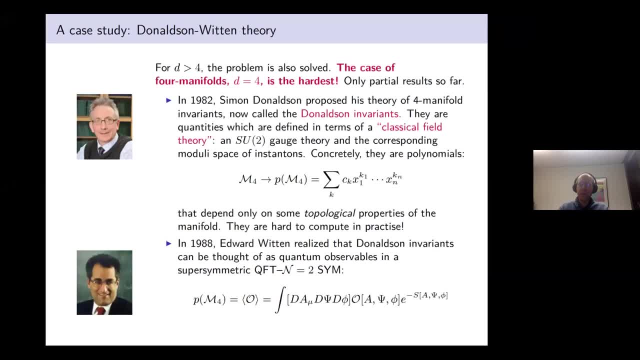 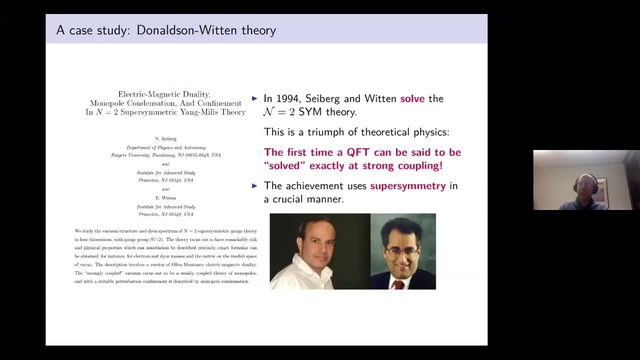 it didn't give a way of computing those things more concretely for mathematicians. But a few years later in 1994, Sabaek, together with with, actually solved this quantum system. and they use supersymmetry crucially and solving that was interesting both for physics. 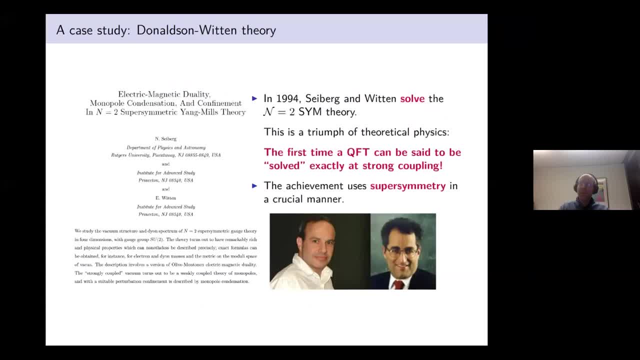 mathematics for physics, uh, it was very interesting because it's the first time that they solve a strongly coupled quantum field theory, exactly. so i told you it was a very hard problem in that case and you know, and in a few other cases like that. now, it's all those are models which are not. 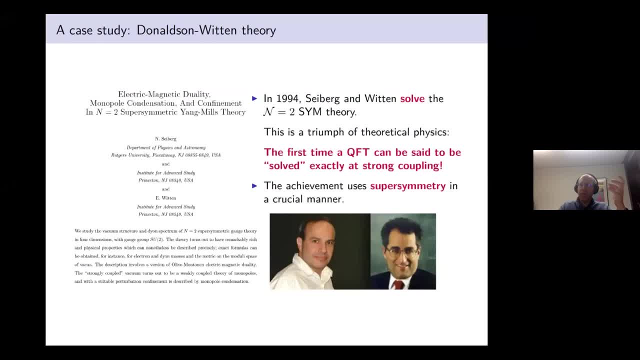 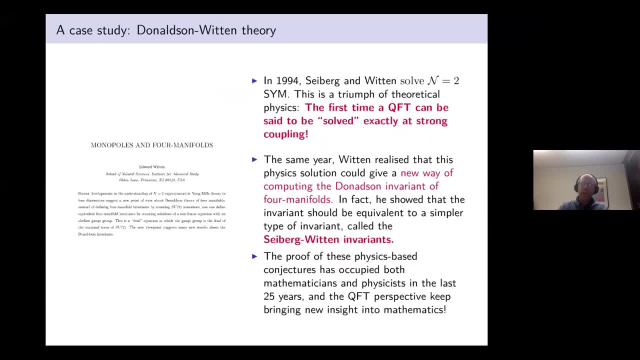 interesting in experiments for nature, but as a theoretical question it's still very interesting. we have this kind of toy model that we know exactly how to solve thanks to supersymmetry. and the same year seberg whitens realized that this physics solution of the, of this quantum field, 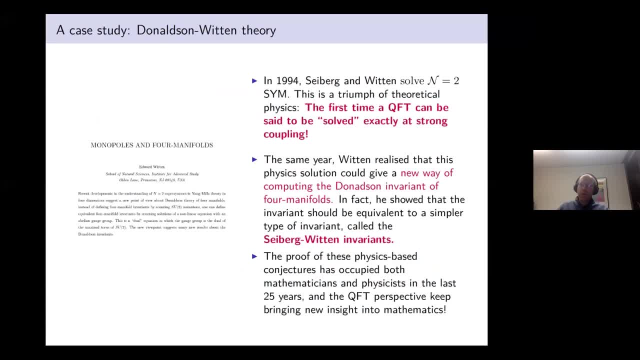 theory with symmetry could be used to uh to write those donaldson invariants for four manifold in a completely new way that was not anticipated at all by mathematicians but that was very quickly followed up by mathematicians and are now called uh seller with any variants and also with invariants. 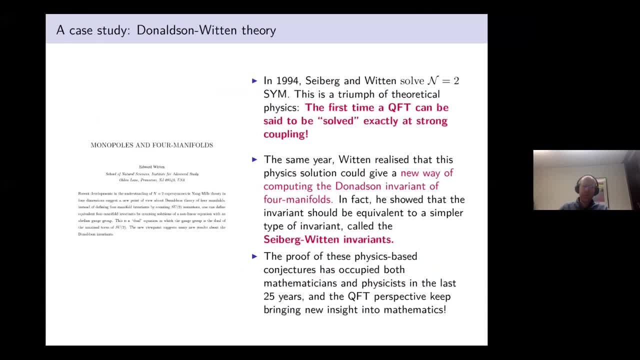 are much simpler uh to compute and have led to a lot of progress in the theory of four manifold, even though it is still an active area of research that has not been completely solved. so this is, i think, a very exciting uh example that uh some of us still work on today, where uh those physics-based 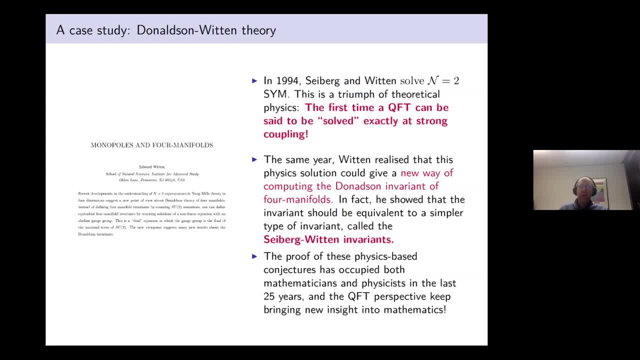 concept and conjecture: uh, really helps solve very deep mathematical problems, uh, and so, 25 years later, we are still working on this kind of things, and that's my conclusion: that supersymmetry is a very important thing, and that's why we're still working on it, and that's. 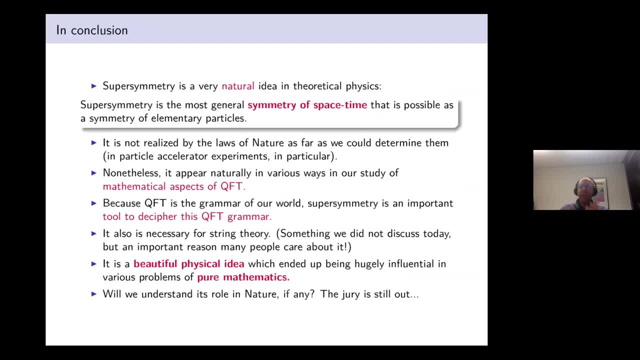 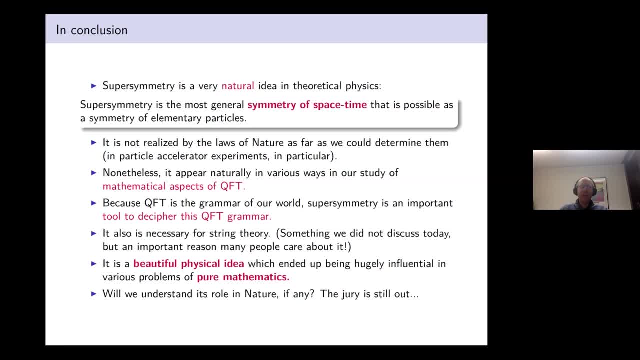 most general, in some very precise sense, is the most general possible symmetry of space-time. that is possible in particle physics, even in any world in of particle physics. that doesn't mean that does not mean that this beautiful idea is realized by nature. nature has not been so kind. 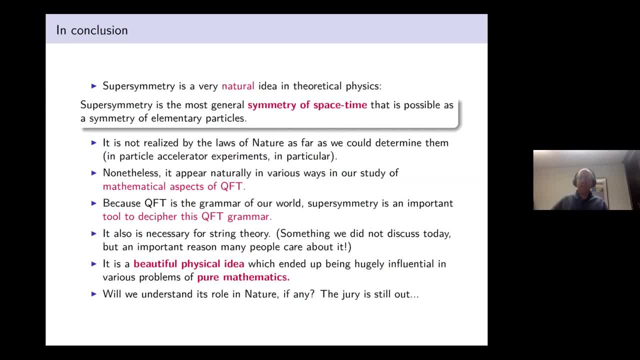 so far. uh, maybe nature is not super symmetric in any way, shape or form it. it is just a beautiful idea, but it is nonetheless a very fruitful idea. um, as i just explained in this, in this, in this example and in also in many other examples, especially in string theory, it has been very 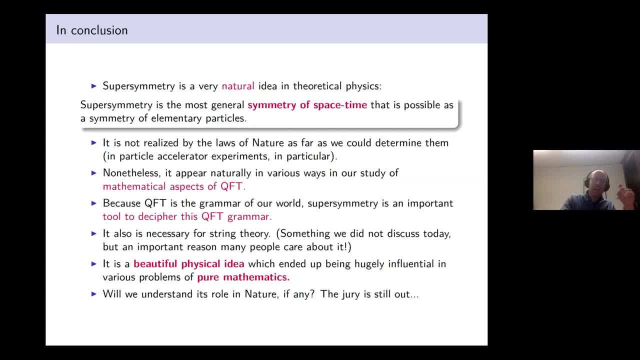 uh useful to to use supersymmetry as a tool to try to decipher um in physics, to try to decipher quantum field theory better, because there are conceptual questions with quantum field theory that supersymmetry help us address. and perhaps, more surprisingly and amazingly, it has been very good at. 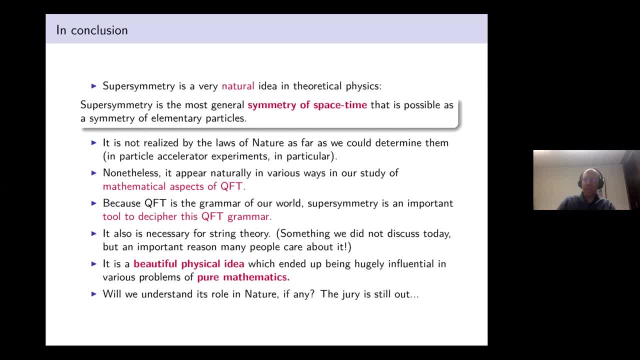 discovering new things about mathematics by just combining insights from physics with this simple idea of supersymmetry. So that concludes this talk and if you have any questions, I'll be very happy to discuss further. I'm sorry for going over time. Thank you very much. Thank you for all the details. That's probably a lot of information. 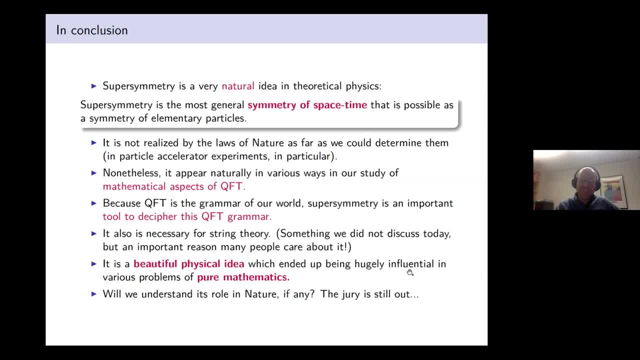 to digest. to be honest, Is there any questions from the audiences? So while people think of their questions, feel free to put them in the chat as well. if you're not having any questions, I'm happy to speak, but do feel free to unmute yourself. 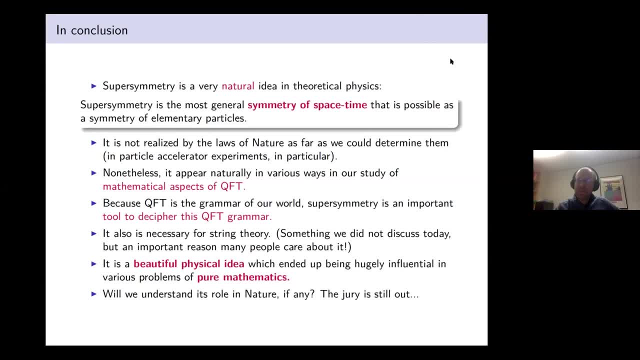 Until then. something that we always like to ask our speakers is kind of: if someone listening finds this stuff really interesting- and I definitely do- what would you recommend they do, apart from going on and picking QFT when they have the chance as one of their lecturers? 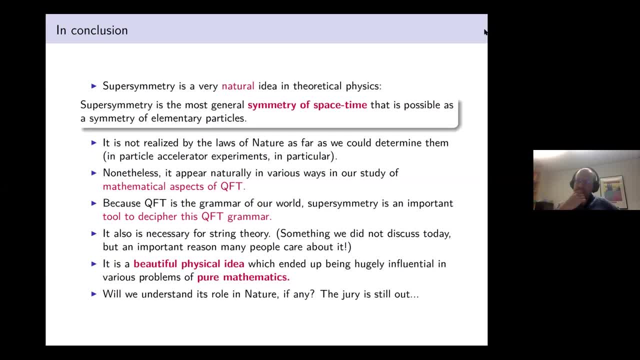 Should they look at any specific maths? Are there books you recommend or anything like that? I don't know. Yeah, I mean, there are like various lectures online about supersymmetry that are very good, but that are like indeed more for a master level at QFT and so on. 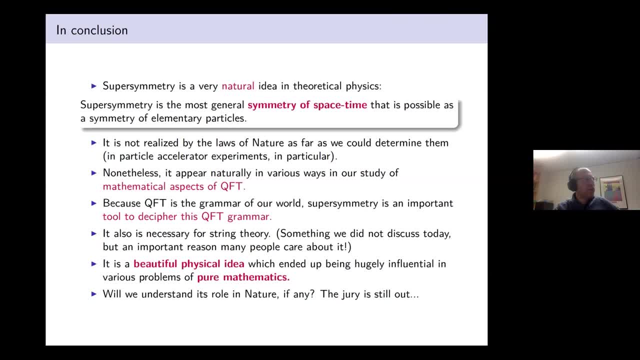 And you know, I'm not sure whether the I mean there are discussions of supersymmetry in books, of course, about string theory And so on, which are more popular level books. I don't know if there is a good entry about supersymmetry directly in mathematics. 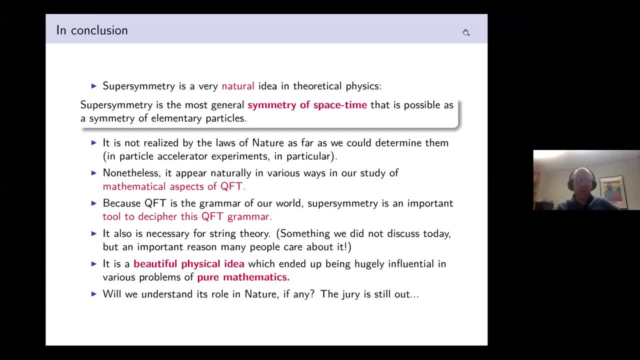 I mean there are advanced books, but not I'm not sure if I. but let me actually put a pin on that and I'll try to see if I can send you by email reference. That'd be great to put that in the event description and the YouTube channel. 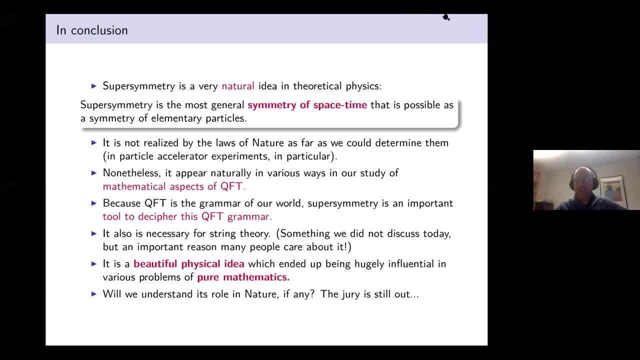 and the YouTube video, because there's different people can find it later on. That'd be interesting, because that's always there's often. it's often astoundingly hard to find good textbooks on something, And then the people who are, you know who know this stuff. they either don't remember which 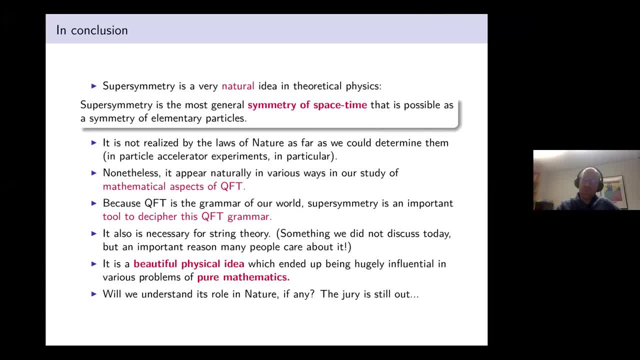 resources they actually use or they just think it's so obvious that that's the textbook to use. So it's always an interesting question to ask. so that'd be great to send that our way. Okay, I'll try to think of a good reference. Yes, Thanks. 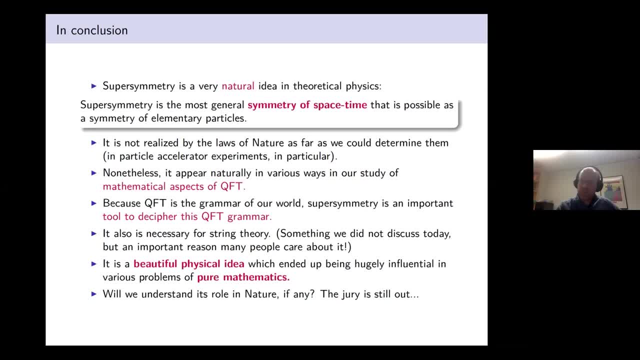 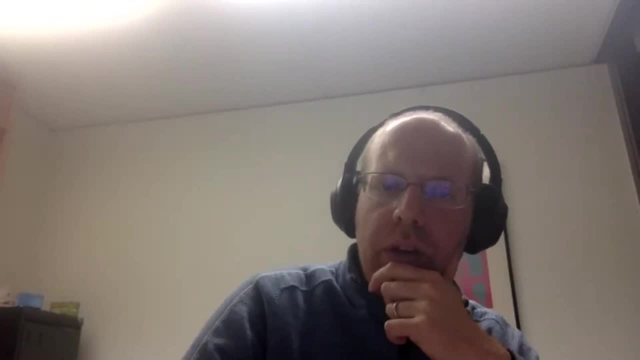 Right, And so I see that there are questions on the chat right now. The first question by Jeremy is that: how does supersymmetry relate to gravity? Sorry, I stopped sharing by mistake. How does it relate with gravity? Oh yes, good question. 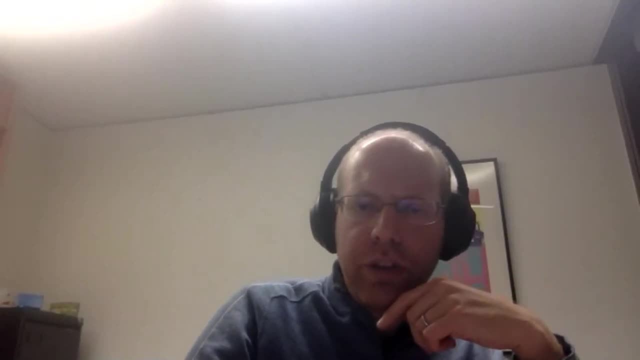 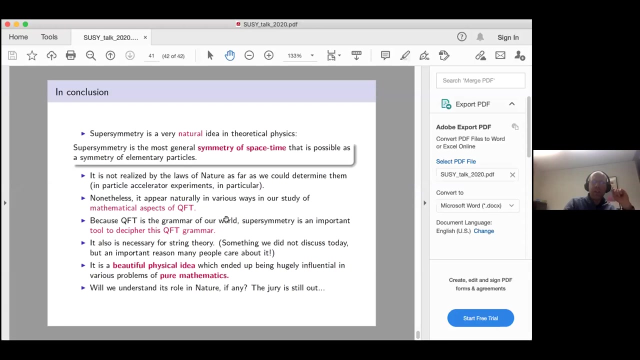 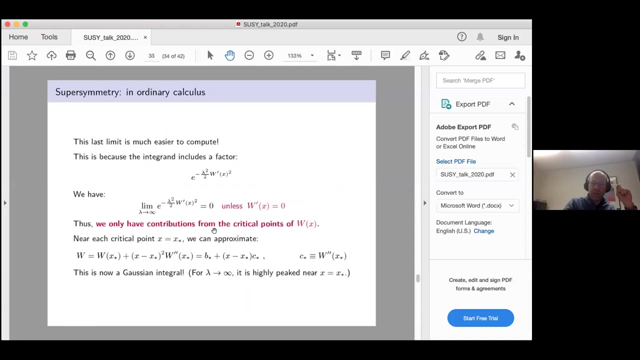 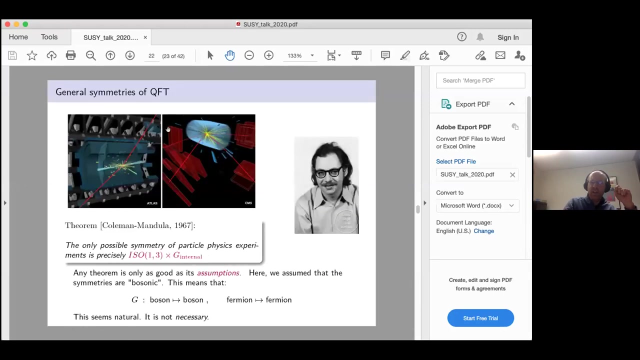 So that's maybe. let me try to share again The. so it relates in a very direct way But very deep way. in fact, historically, If you look at how you mentioned it, Yeah, When it was discovered Supersymmetry has this concept of in quantum field theory was actually discovered not. 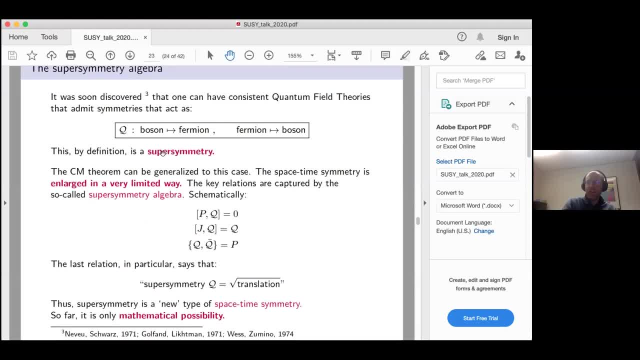 in what we would call a four-dimensional QFT of particle physics, but in string theory, In 1971, the very first model with supersymmetry was told by Mi могут, l'adachter Parisian theory. and in string theory it is an unnecessary condition to have a consistent string. um and 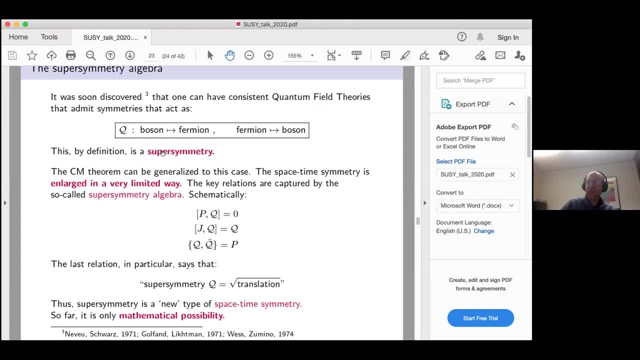 string theory is the only consistent theory of quantum gravity that we know. so in that sense, uh, the only theory we know where, uh, where gravity is is a quantum theory also has supersymmetry built in naturally. now this is supersymmetry on the string. so i think you you've heard about. 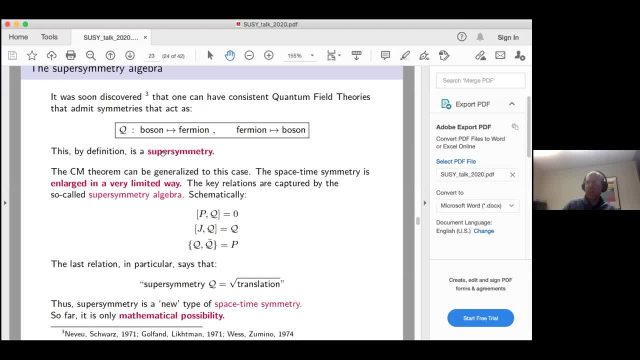 strings last week. so strings are those tiny, uh little objects, right, that replace particles at the fundamental level, conjecturally. and supersymmetry is a symmetry on the, on the string itself. it's not a symmetry in that theory. it doesn't need to be a symmetry of our space time. 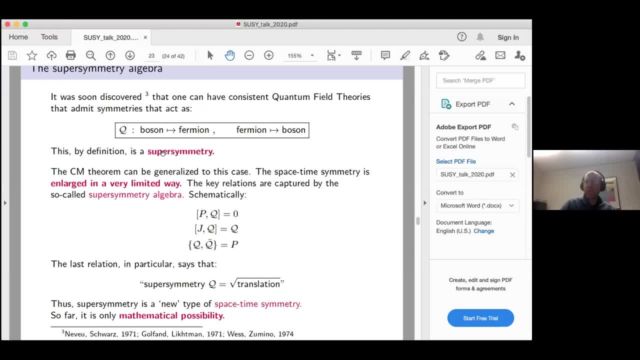 in which we live. it's a symmetry, that kind of lives on the strings, uh. but yeah, it's uh in that sense, uh, it's, it's very tied to the idea of- i mean to, to uh, to gravity, as envisioned by string theory, because we really need symmetry as a concept to even make sense of the of the equation of string. 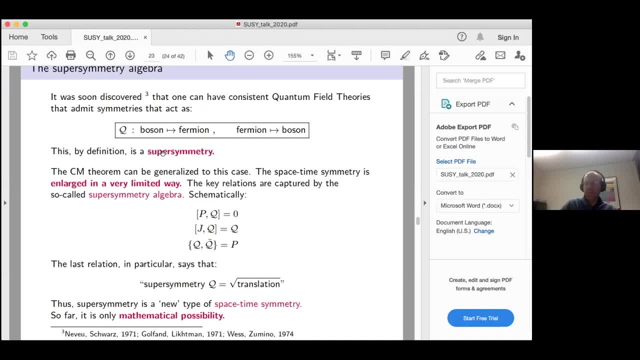 theory, really right? um, thank you very much, and so i. i see that there's a second question. oh, there's a third one. okay, um, the second question by xavier- sorry if i pronounce the name wrong- um ask: can you tell us about supersymmetry and uh and condensed matter? 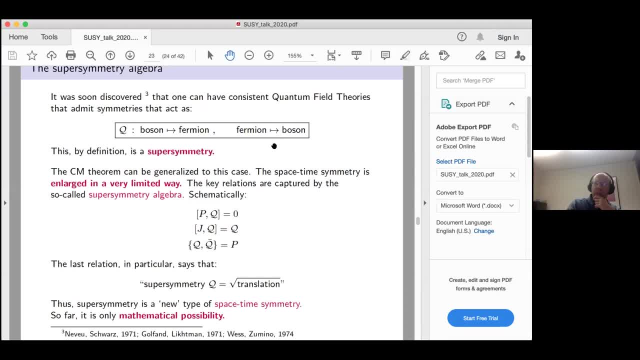 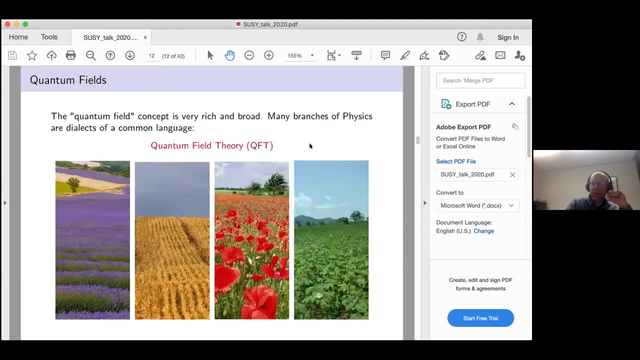 um, i wish i could. i mean, uh, i mean there's been. so i told you that quantum field, right, uh, coming all kind of flavors and precisely in finance matter, uh, there are all kind of quantum fields that are effective description of various systems like metals and so on, and we can build. 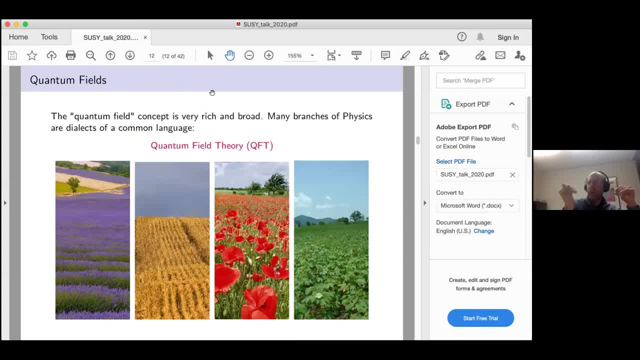 unlike in particle physics, when the number of fields are fixed once and for all in uh. in comments matter, you can, uh, you can- engineer all kind of quantum field theory. i mean essentially, you have complicated materials and they can describe by effectiveness, effectively described by complicated quantum field theories, without repeating class. 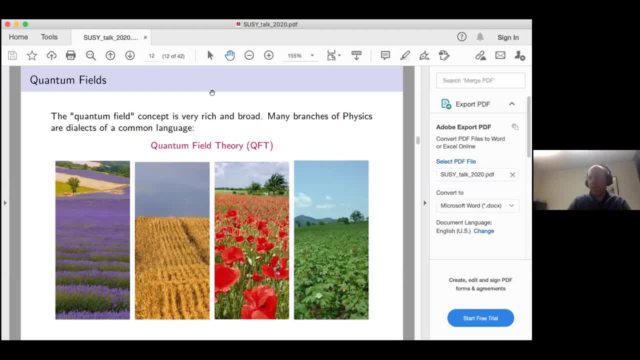 and so you could try to engineer some system in the lab which has both thermons and bosons that will be exactly supersymmetric. i think there's been trial. i think there's been even some claim recently. at least theoretically it's possible, uh, and so it's. it's possible that it will. it will be. 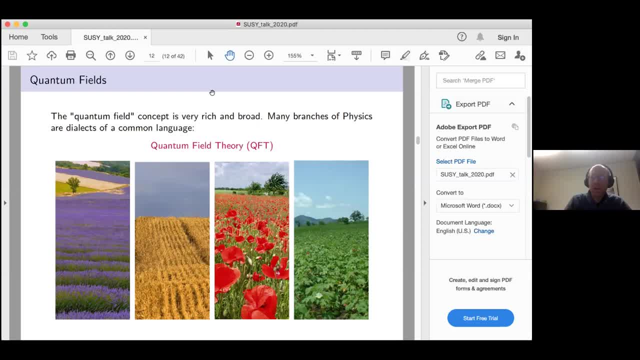 or maybe it has already been. uh tried to build supersymmetric model in the lab when you would have some kind of metals with bosonic and thermodynamic station that would have this symmetry between boson and fermion. so that's that that might happen in some complicated metal or other type of condensed. 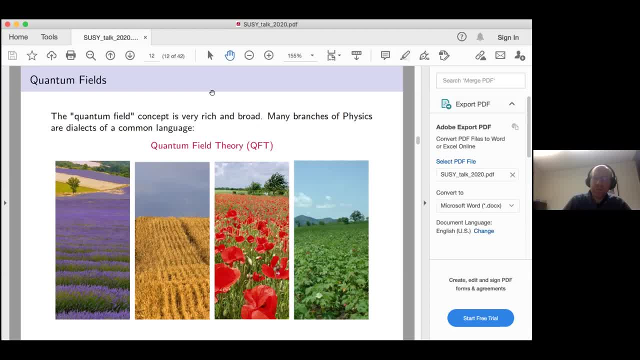 matter system, right? um so the next question is that: uh, i gave up reading the names right now. sorry about that. um so is there supersymmetry in brains? uh, yeah, i mean that's the brains are. uh. uh, brains are those objects in string theory, right i guess? 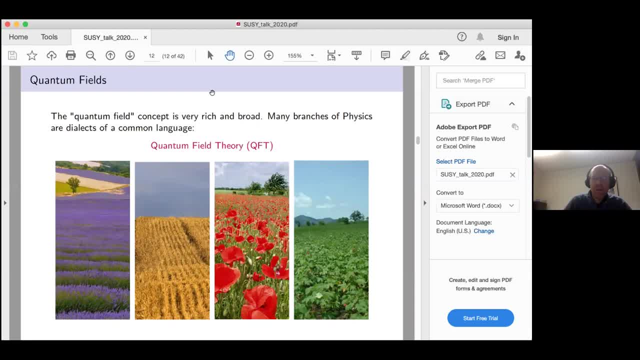 what you mean, uh, so like strings, is a one-dimensional object that moves in space time, and brains are dimensional, and planes that are supposed to move in space time and that appear naturally in string theory and, uh, i mean, a lot of these objects can be supersymmetric or not, but the 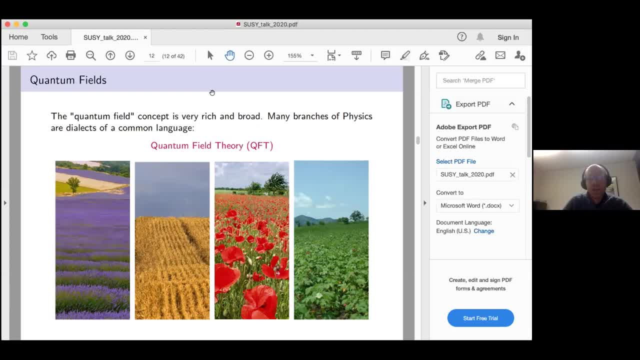 whole supersymmetric in string theory, and so yeah, the point is that here i discuss supersymmetry in a two-dimensional, in a four-dimensional particle physics world if you have three space dimension and one dimension of time. but really you can do the same game in abstractly and we do the same. 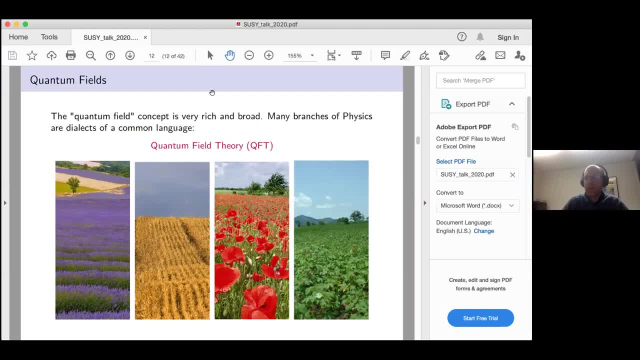 game in any type of space-time dimensions. uh, dimension space, dimension two is a string. then you can do that in dimension three, four, five, six, uh, and those will be essentially brain systems with supersymmetry. so theoretically, yes, there is no problem with that, right? um, thank you, uh. so, uh, one of the audiences said that there's a. uh, it's a pretty good. 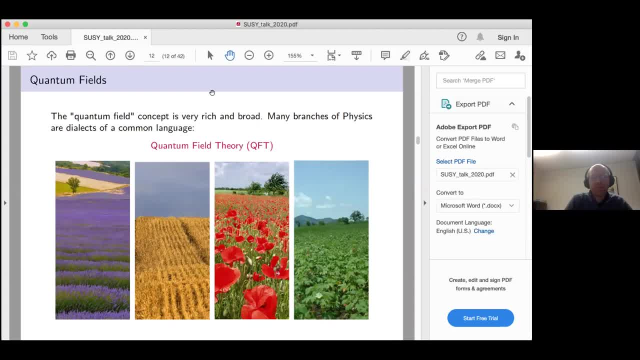 i think he means a textbook or something like that. um, so yeah, that's a good. i mean, i think it's a pretty technical textbook, but uh, it is a good textbook which has uh as the name. name subject has the name, so so just sorry, as the name, uh. 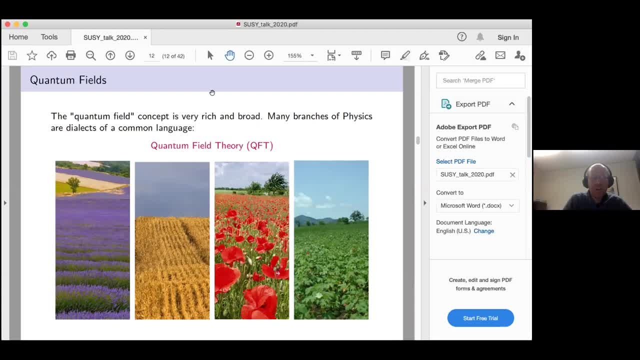 suggest uh is. uh is very thorough, it's very loud, very long, but it's it's available for free online so you can just google it. indeed, uh, but it's, it's pretty, i mean, i think it's. i mean, i don't know what you're looking for in terms of i think that's a bit advanced for uh, maybe for uh under that, but 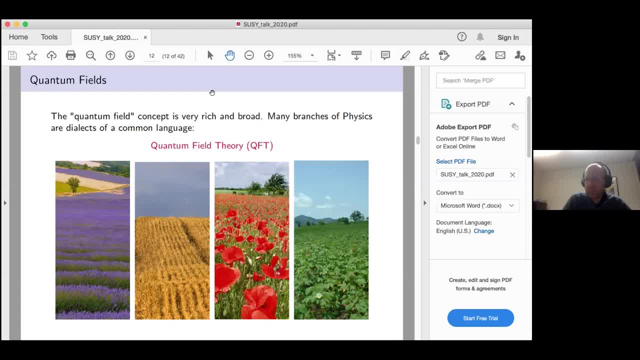 but, yeah, i think it's a good textbook. okay, um, thank you for sharing. uh, so is there any more question from from the audiences? um, um, um, um, um, um, um. ah, there's another one. um, what does q equal to square? root of translation means actually in. 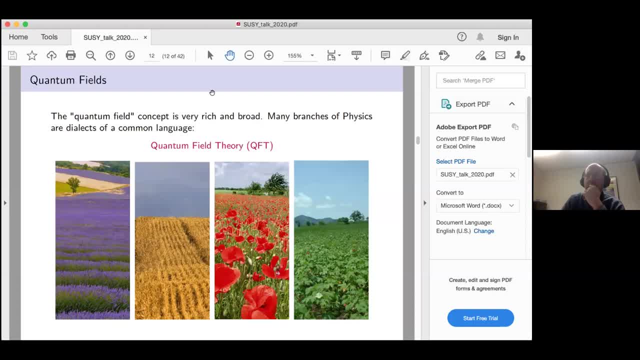 physics, right? well, in physics, what do you mean in physics? um, well, what it means is: i mean, this was more like a square of position, is not the actual things, right? because, uh, what it meant, what i the actual relation, was: q squared equal translation. um, then, you can rewrite it in that way formally, so q squared equals transition. just means that, as i. 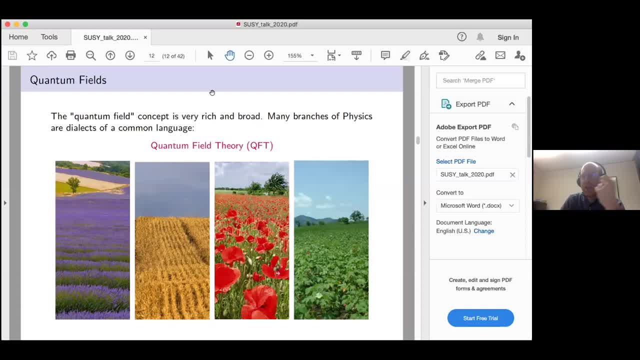 said: if you act with one supersymmetry on the boson, you get a fermion. if you act again on the on the fermion on that same term and you get back the super symmetry on the boson, you get a fermion on that same term and you get back the same boson essentially. but translate it, that's what q. 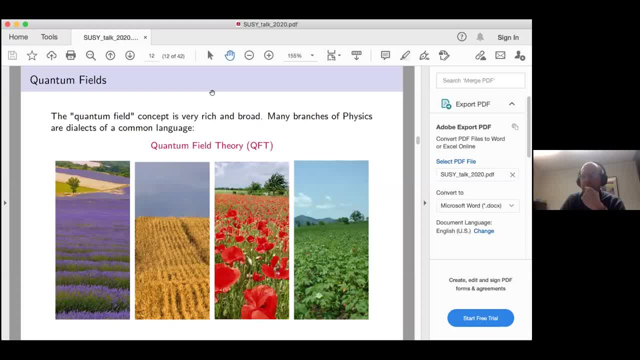 squared equal translation means: so that's, that's it. um then, i mean, it's not been realized in nature, right? so we don't. we don't have intuition about that like we have for concept like conservation of energy and so on. when we have an intuitive concept, yeah, it's a similar conservation law. 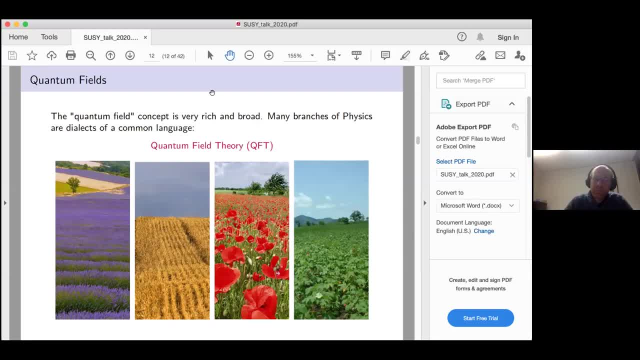 nonetheless, um all right, okay, um, uh, is there any more questions? so, um right, if, if there, if if not, so, uh, i would say that this would be the end of this wonderful extracurricular class and again, thank you very much for giving us the opportunity. um so again. 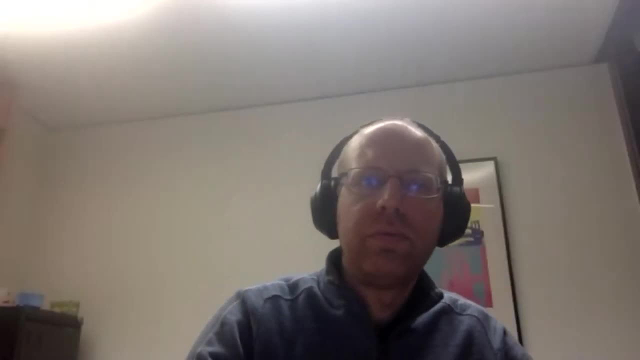 this will be recorded. we will upload this on youtube afterward and, uh, be sure to like, follow the facebook and all the stuff that we're going to be doing in the future. so thank you very much. like that, um and uh, oh. uh, there's one more question, so i i would say i would call this to. 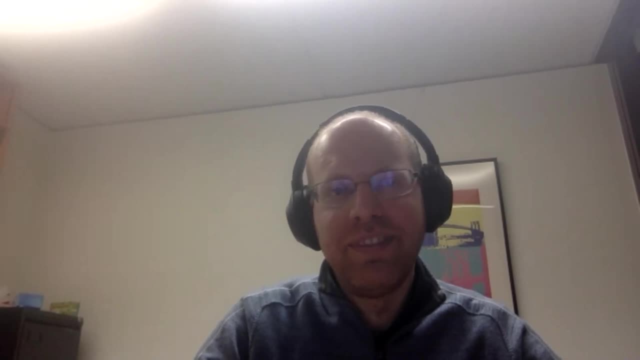 be the last question, because, uh, we're running a little bit over time. um, could q deformed super symmetry be used for deriving mathematical facts? uh, for example, smooth manifolds? uh, yeah, i mean, i'm not sure what you mean, like you deformed, but yeah, they're all kind of of course. uh, uh, they're all.